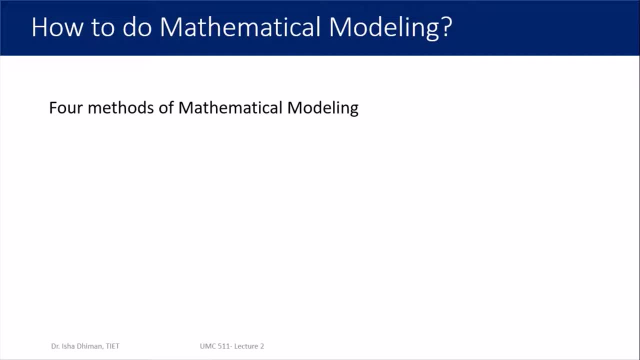 underlying real-world phenomena for which you are making a mathematical model. for that there can be entirely a different technique can be used for that particular problem, like these, four techniques can be used independently also, or they can be used in combinations also, but it's not mandatory that all of them have to be applied for one particular. 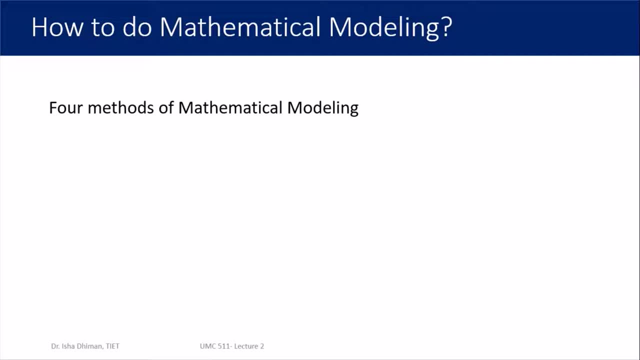 problem. so let me give you these four techniques. the first one is dimensional analysis, which we are going to cover up in this lecture. the second is scaling. in fact, these two are related with each other: dimensional analysis and scaling. the third is conservation laws. and the last one is constructing linear models. 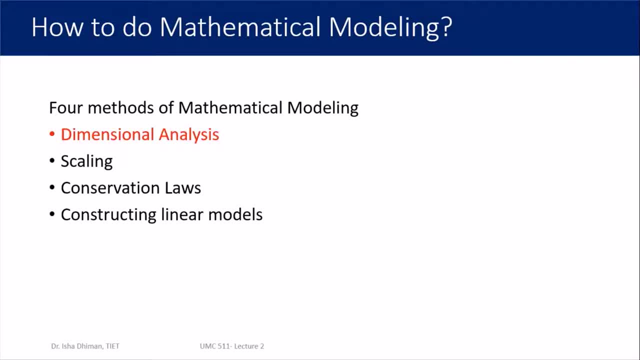 so in this lecture we'll be starting with the first one, which is the construction of linear models. so in this lecture we'll be starting with the construction of linear models. so in this lecture we'll be starting with the construction of linear models. so in this lecture we'll be starting with the. 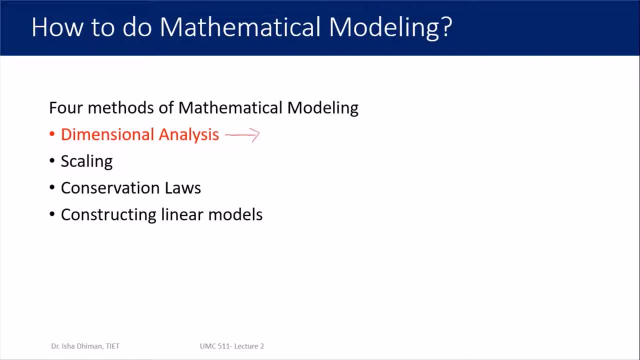 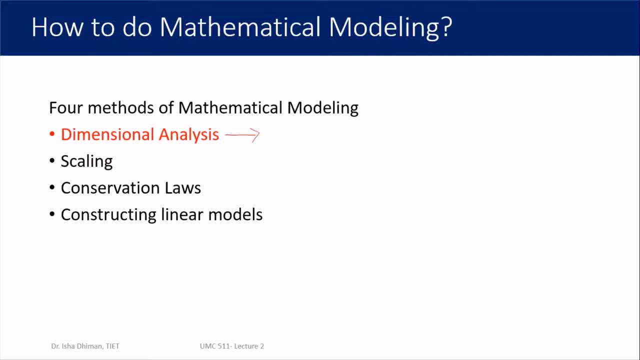 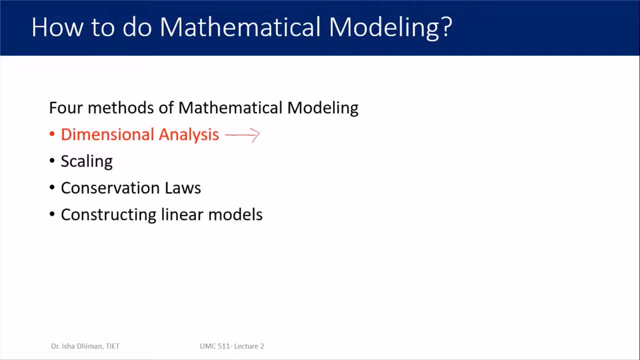 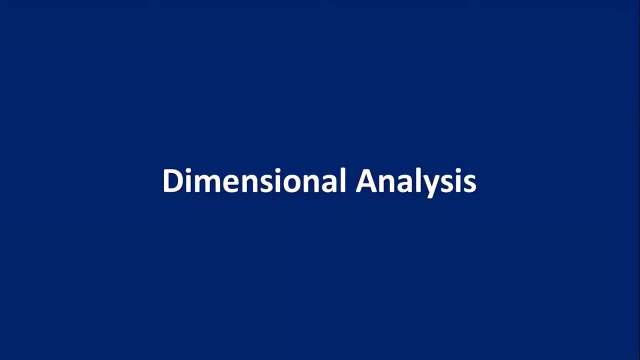 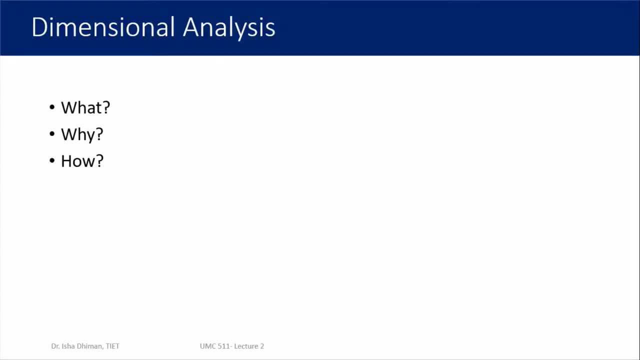 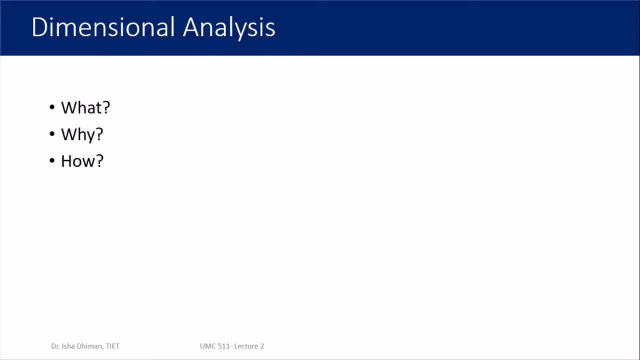 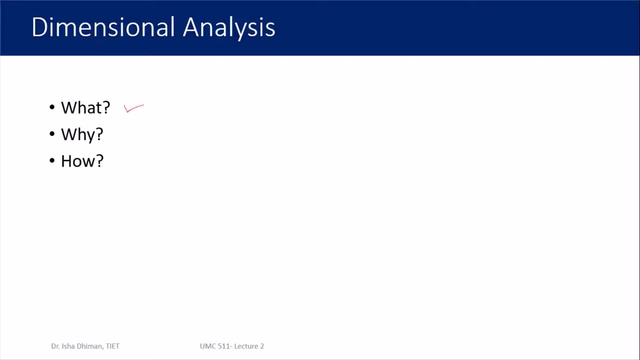 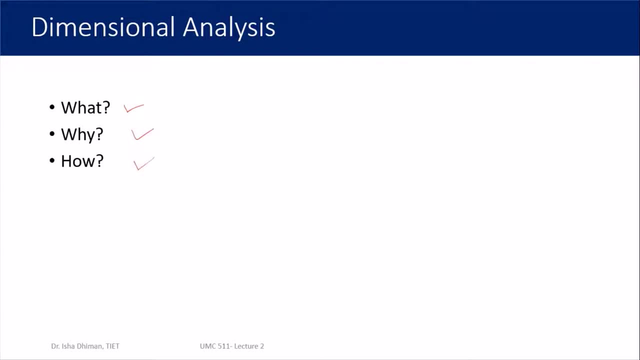 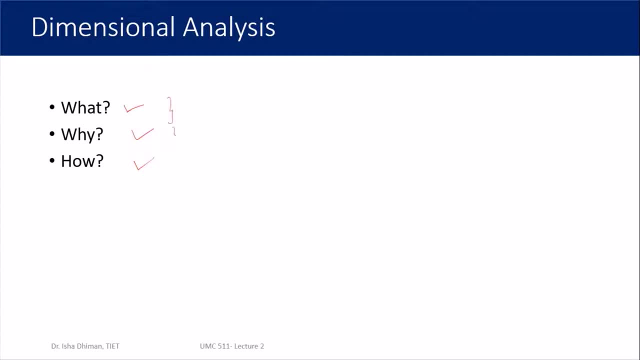 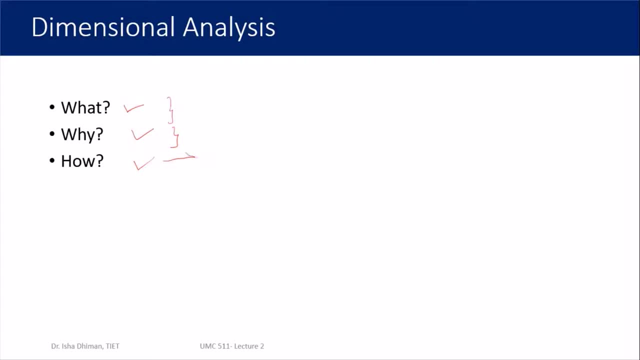 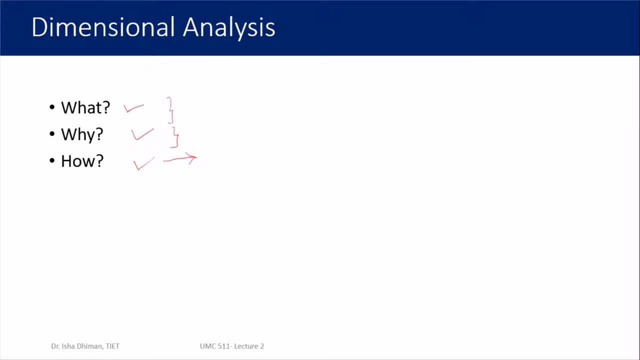 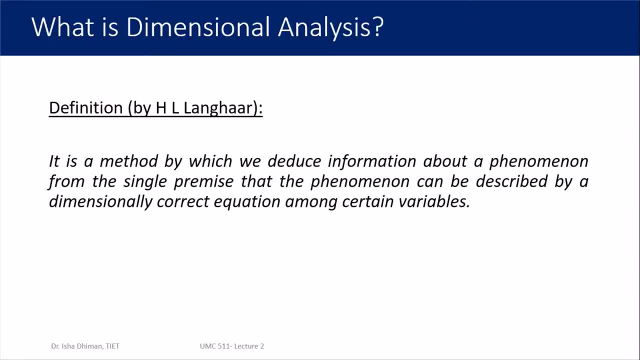 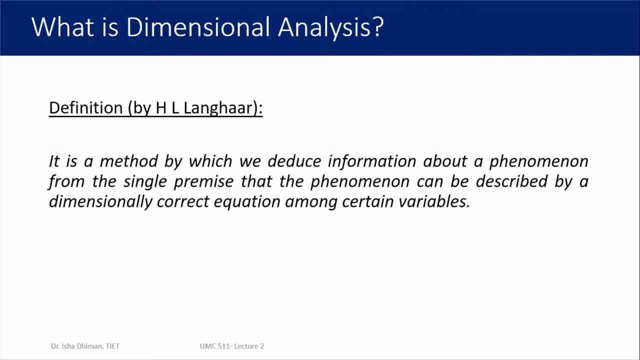 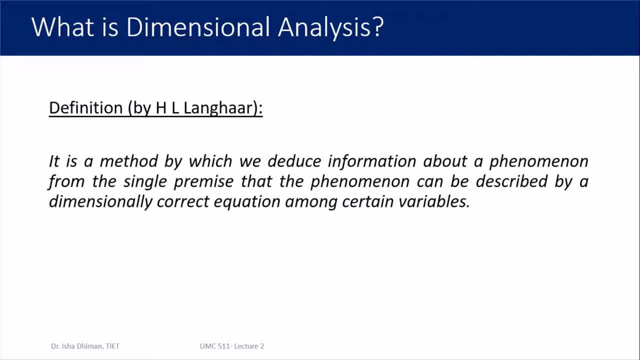 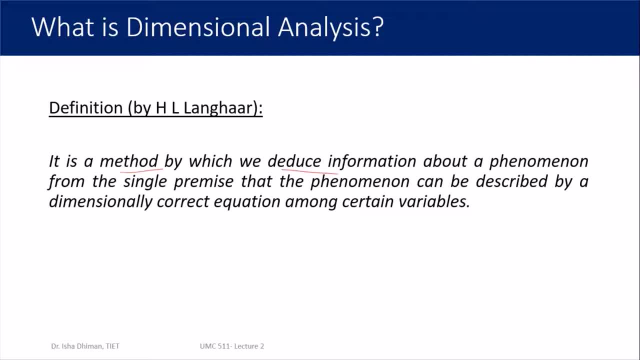 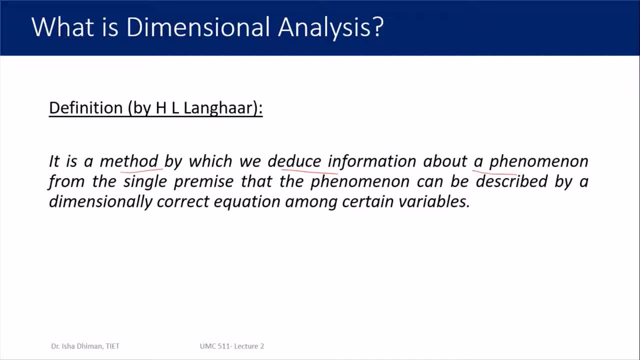 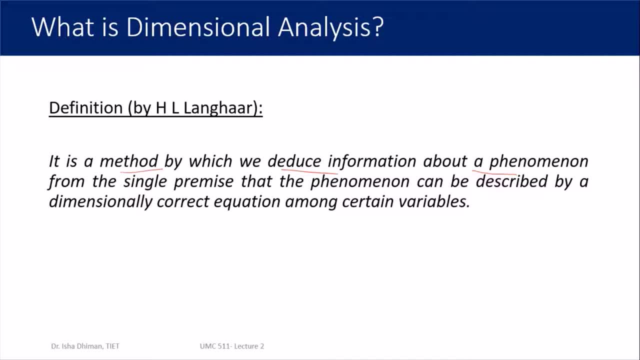 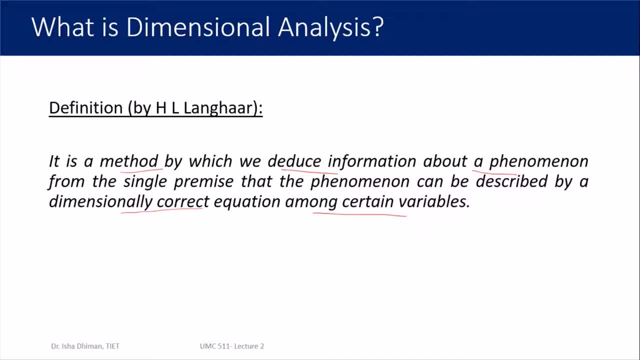 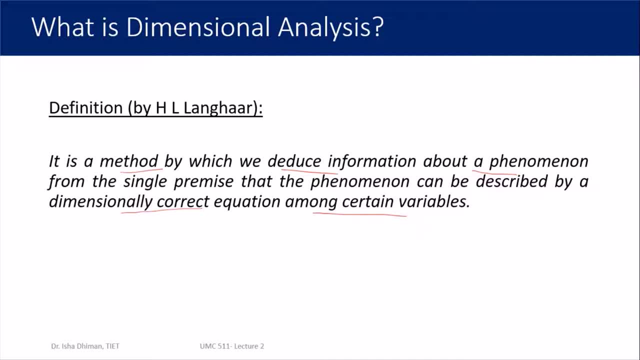 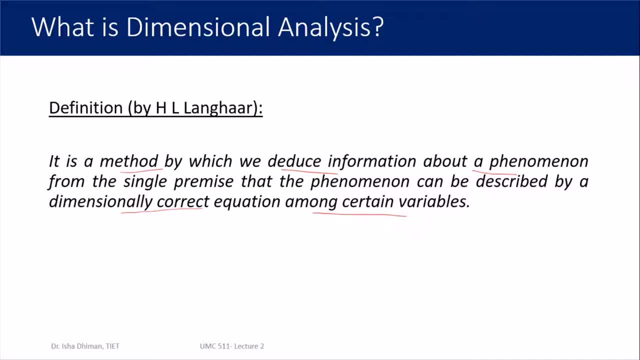 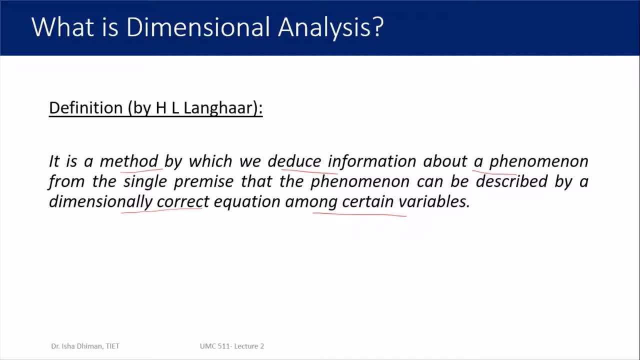 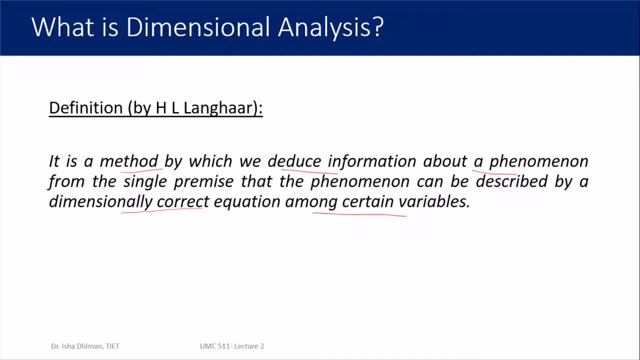 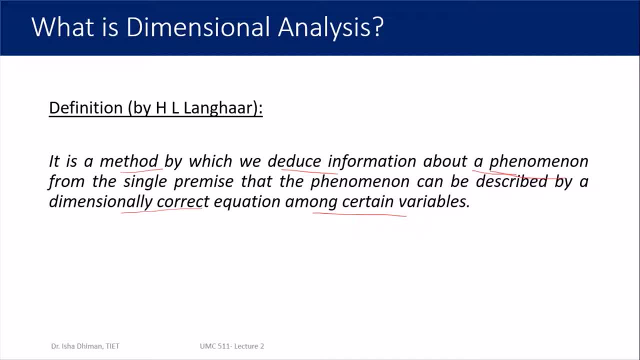 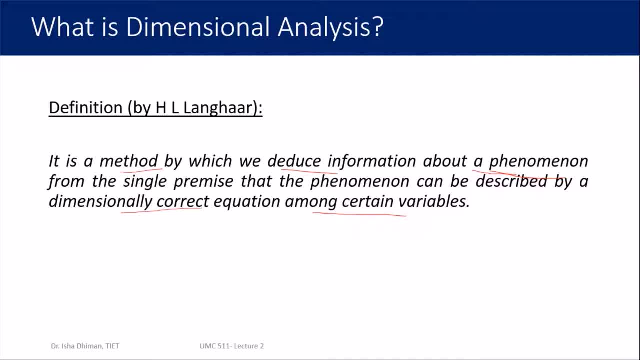 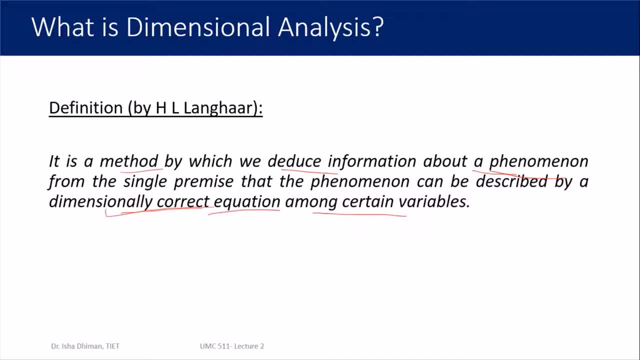 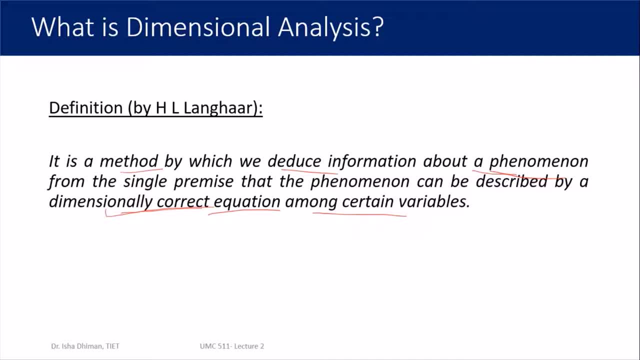 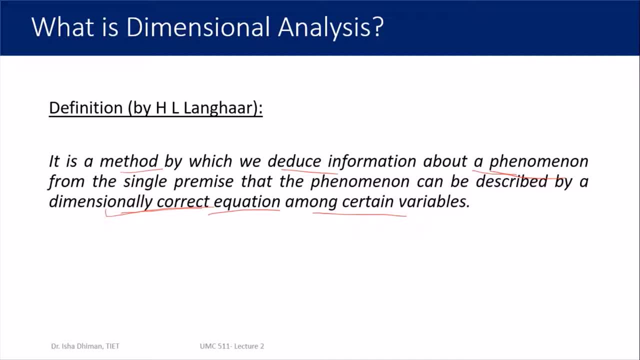 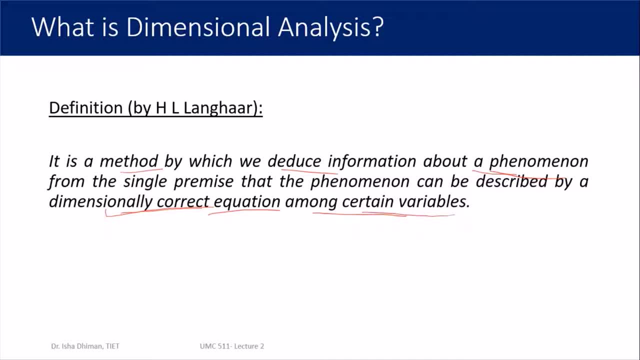 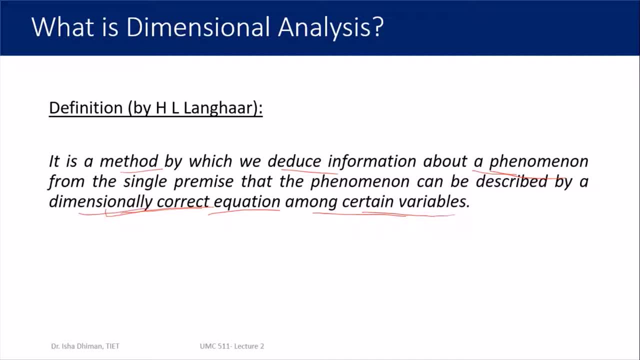 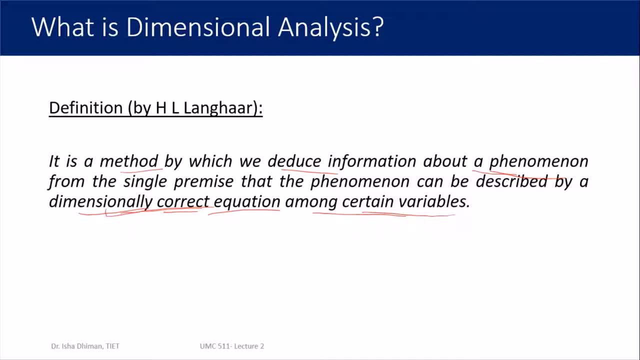 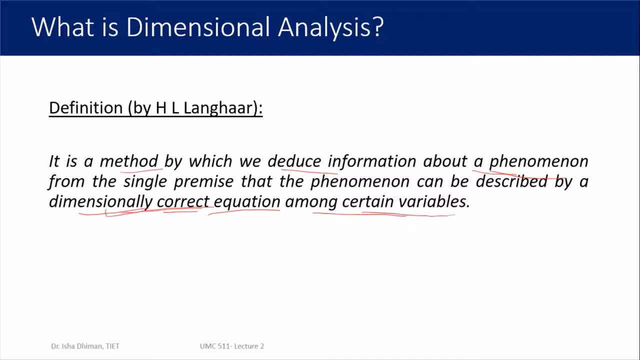 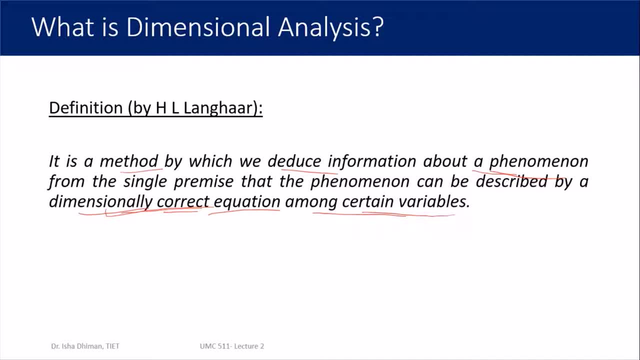 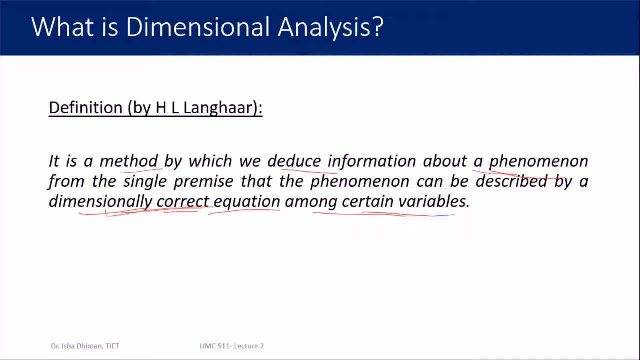 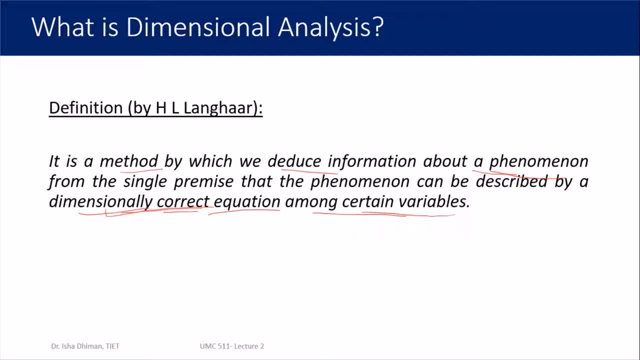 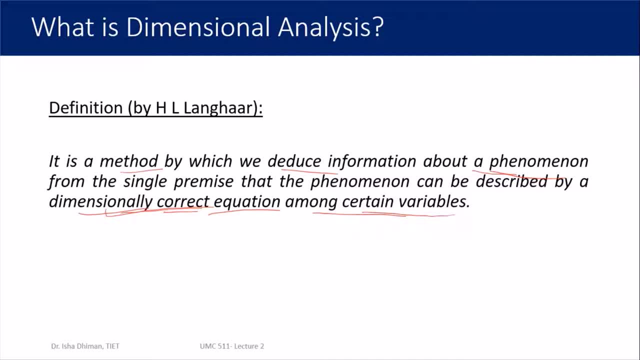 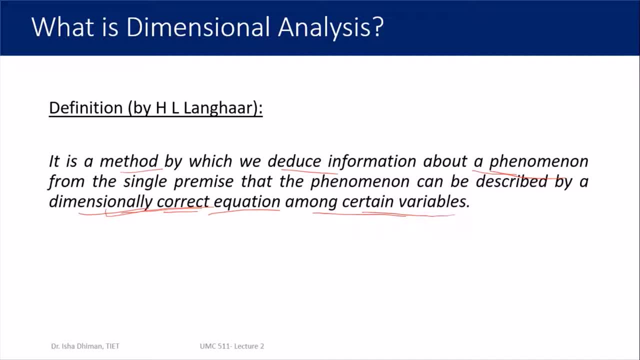 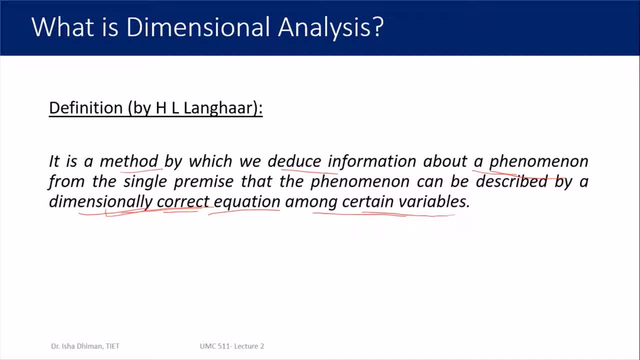 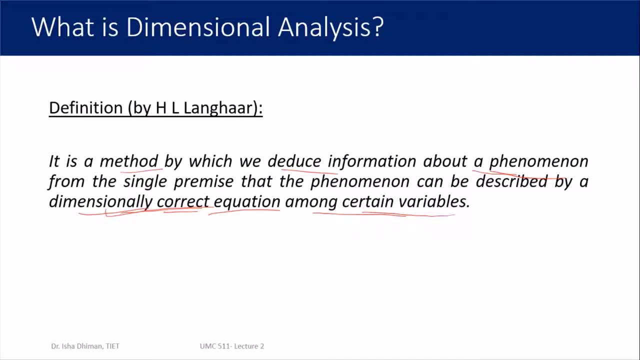 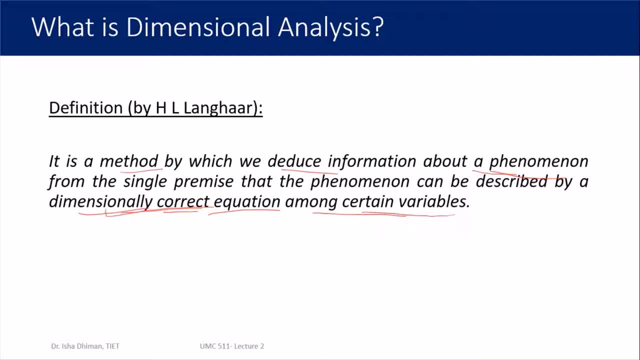 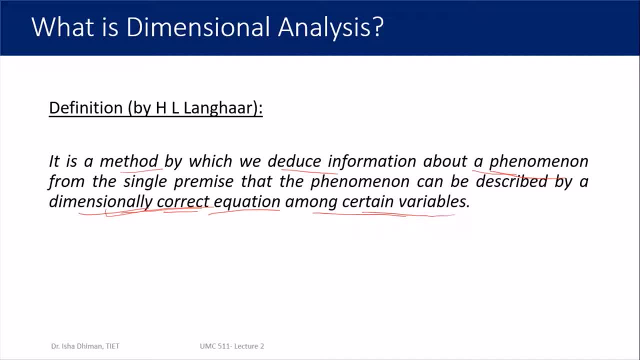 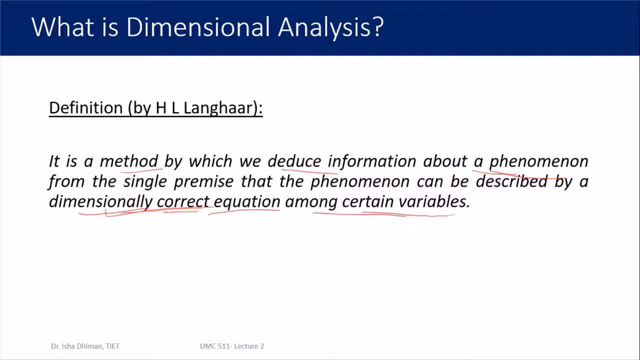 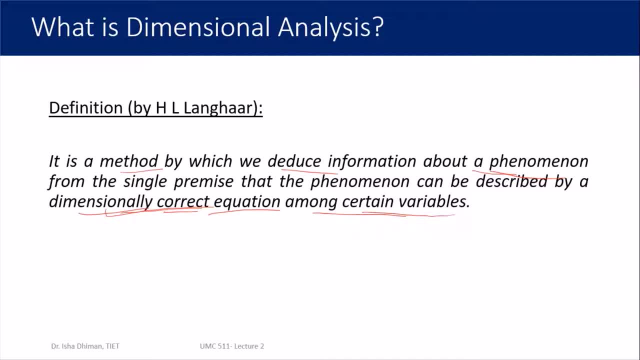 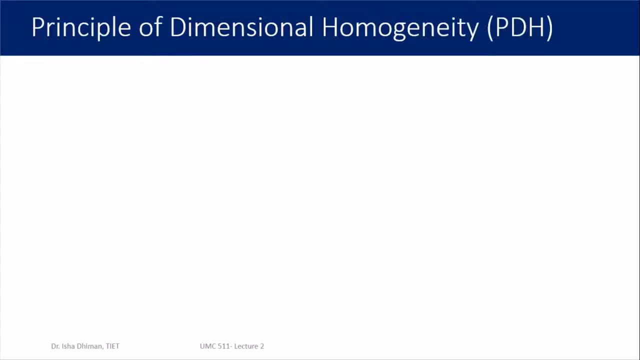 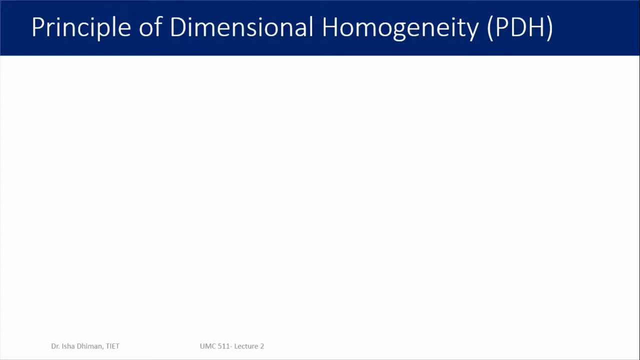 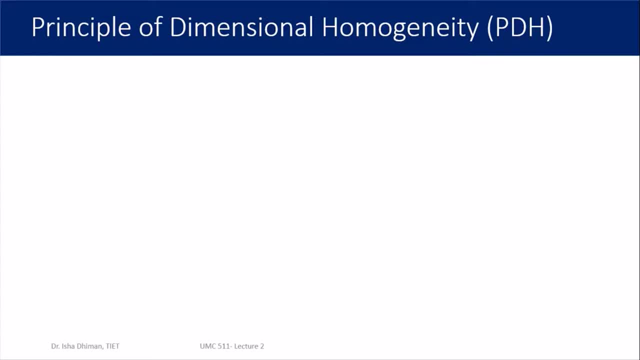 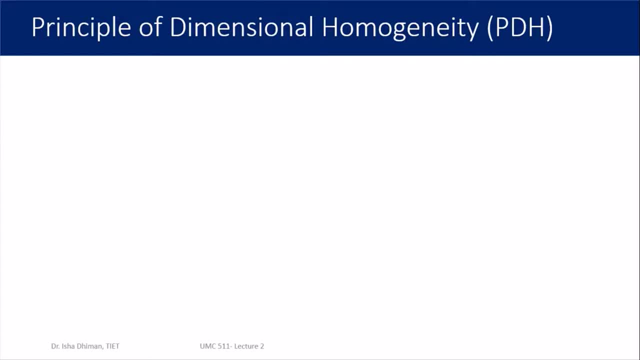 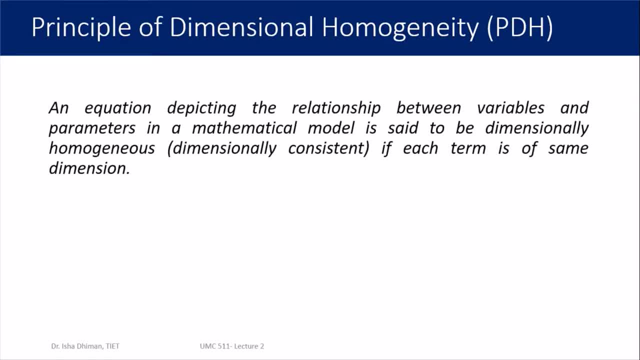 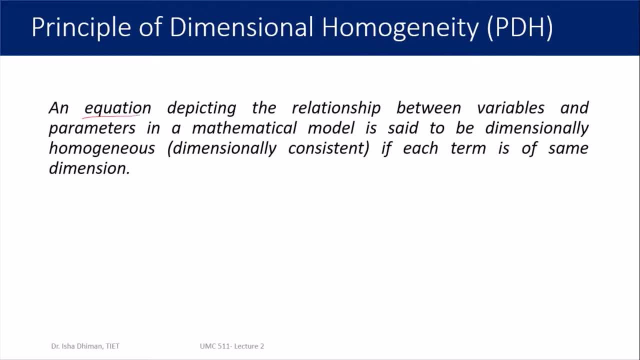 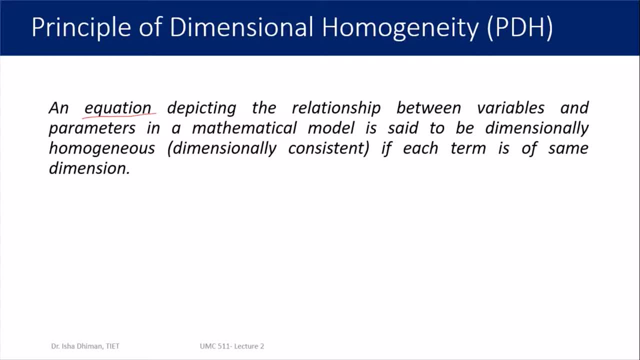 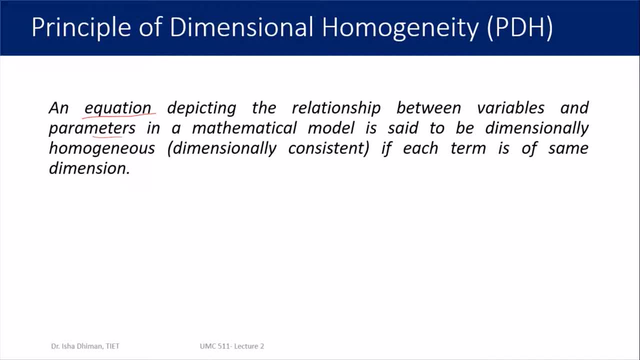 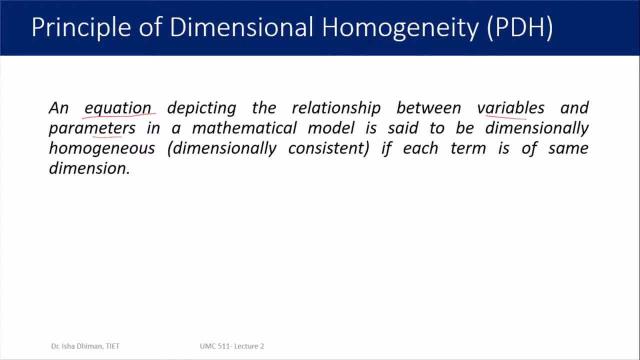 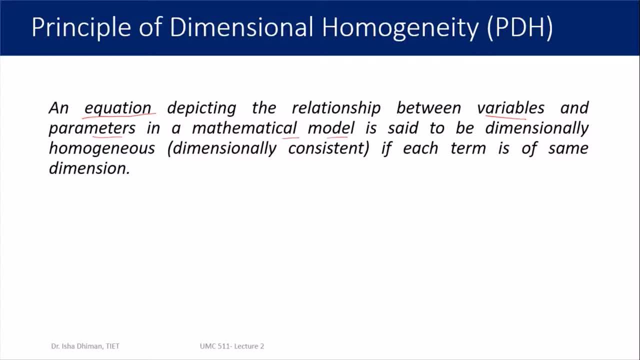 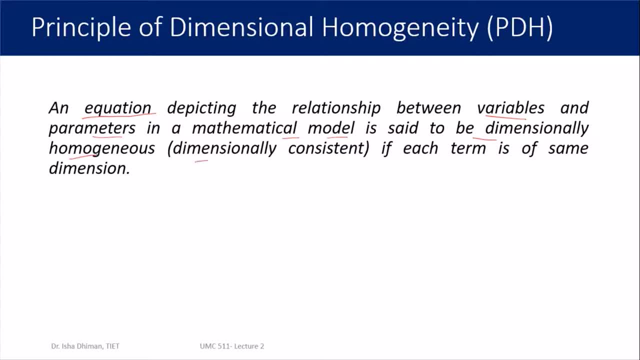 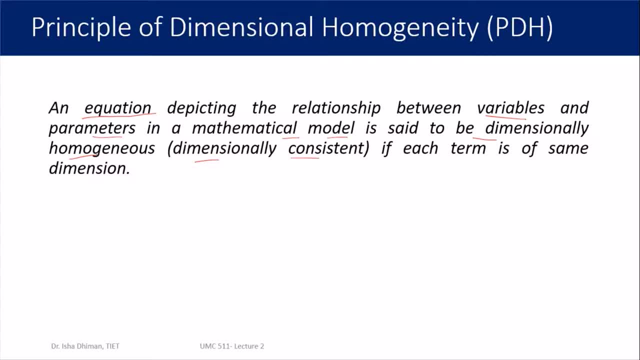 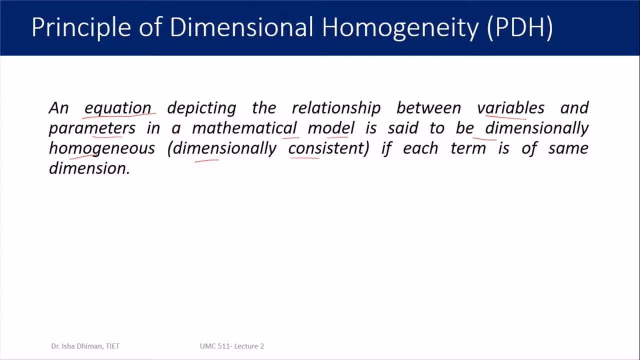 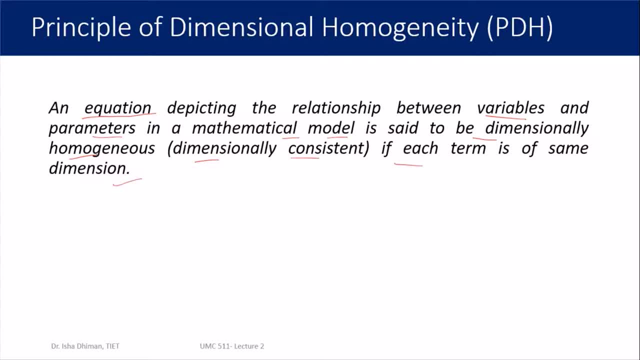 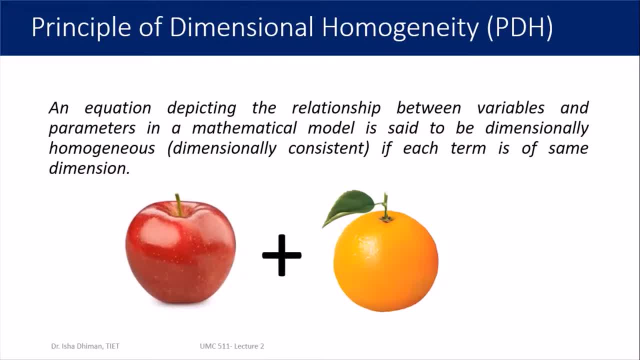 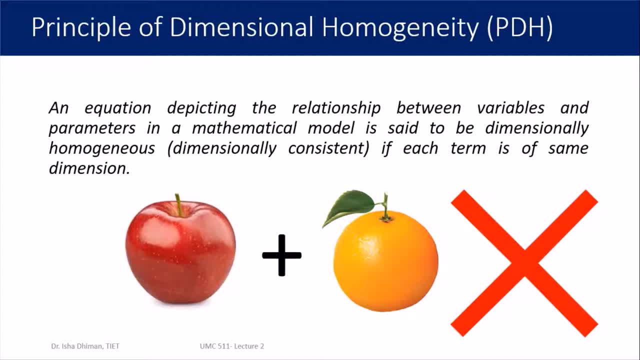 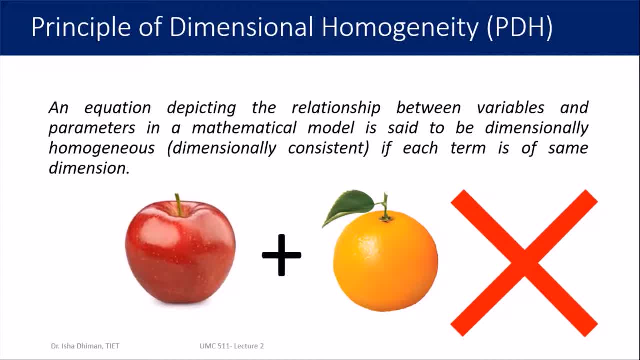 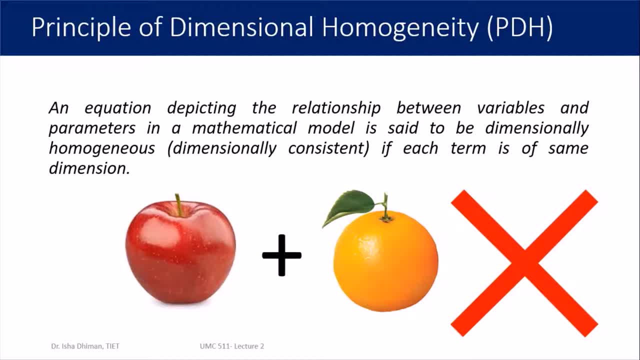 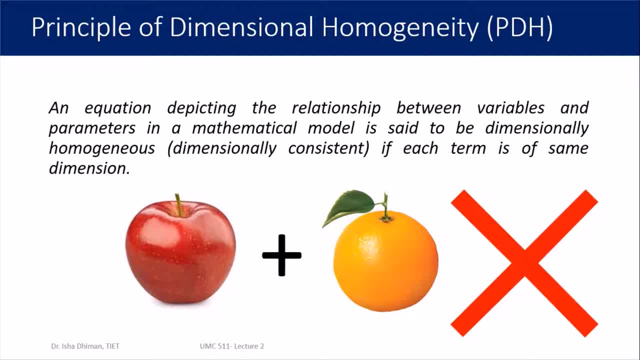 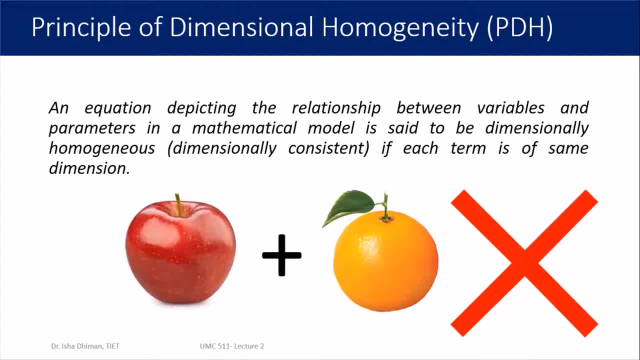 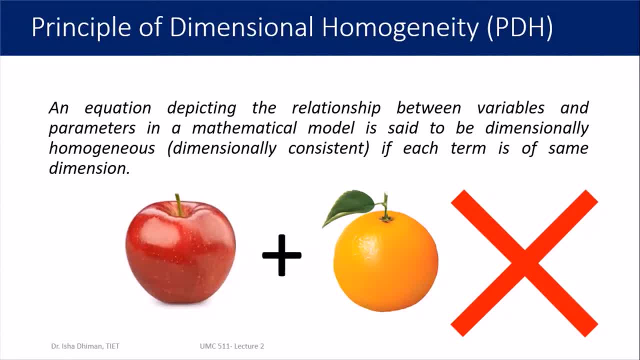 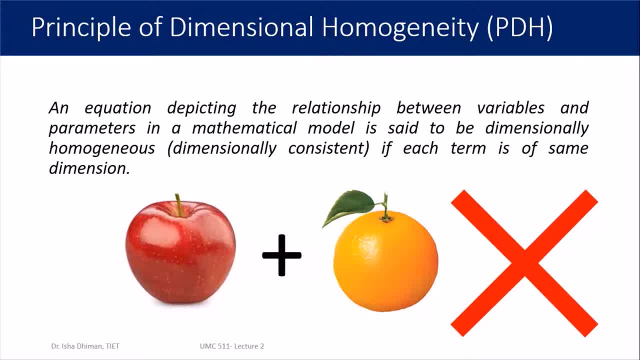 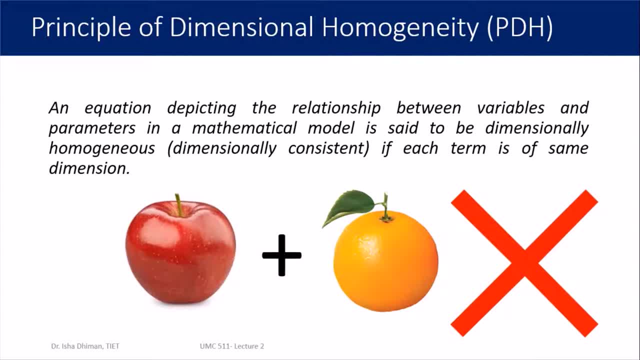 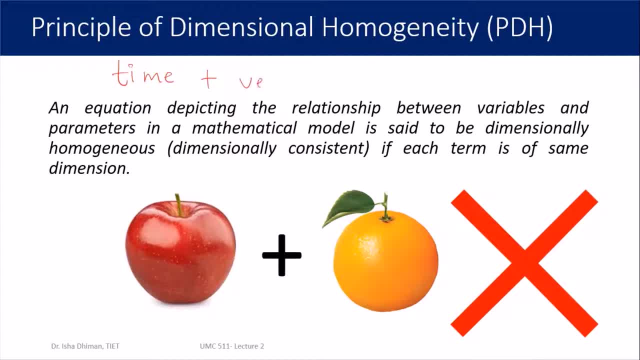 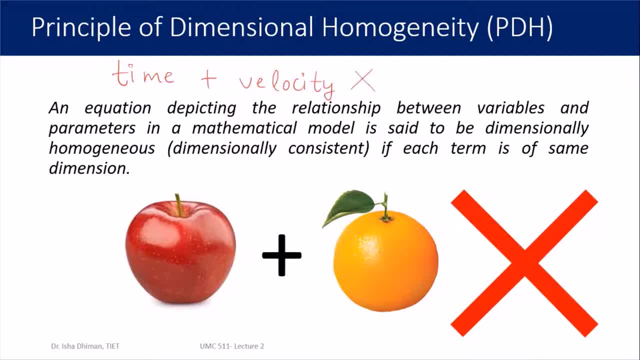 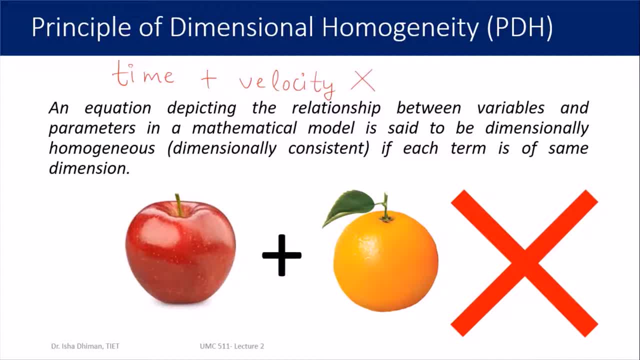 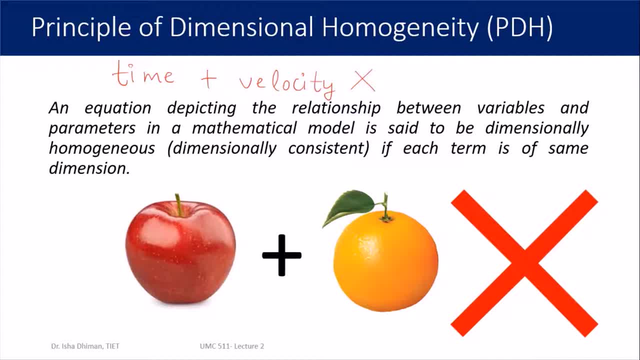 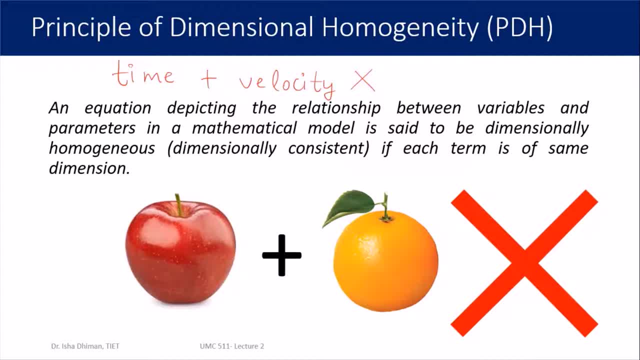 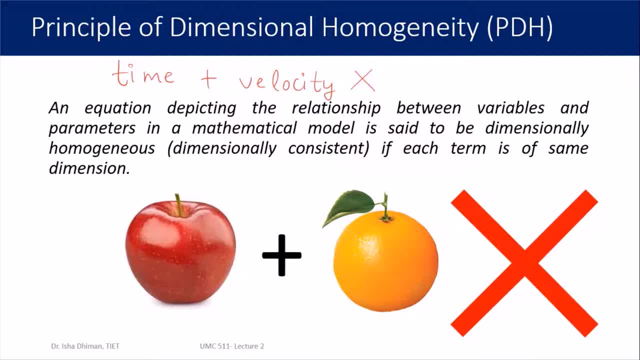 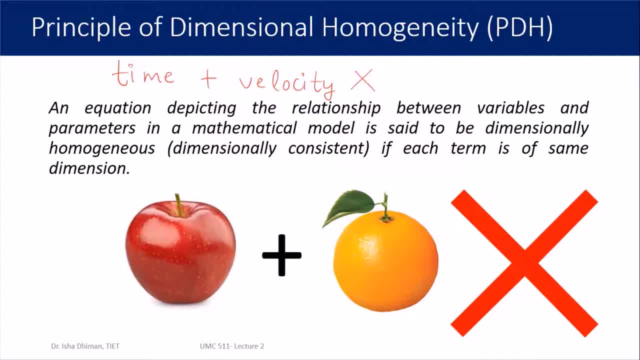 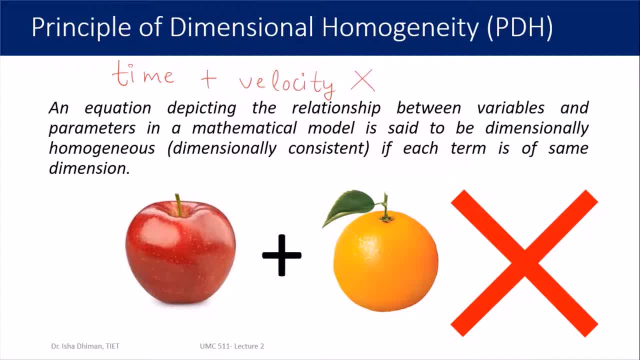 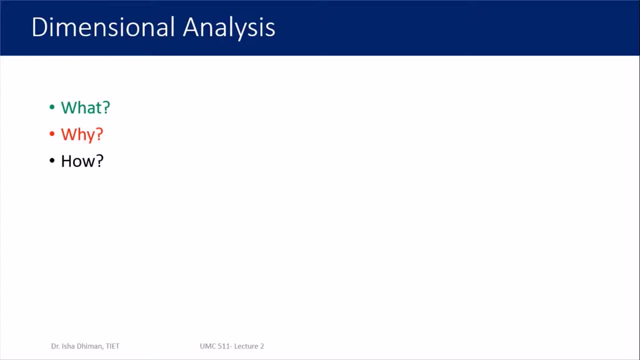 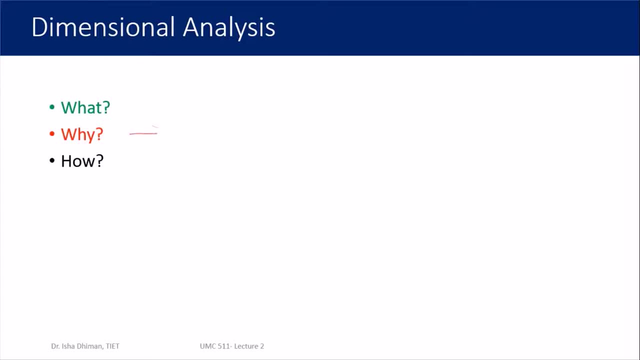 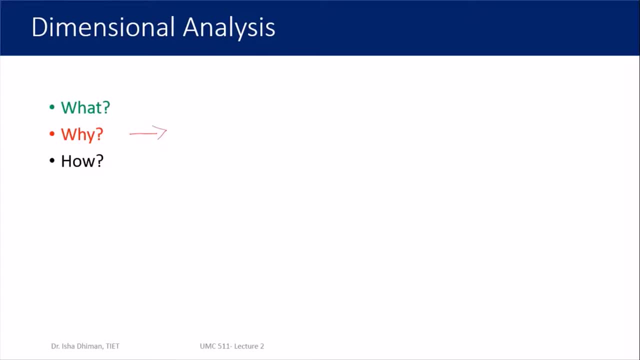 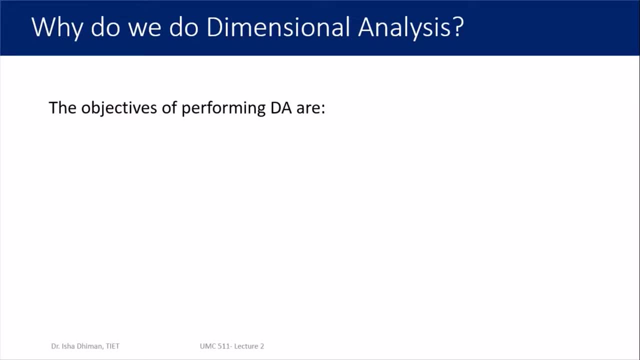 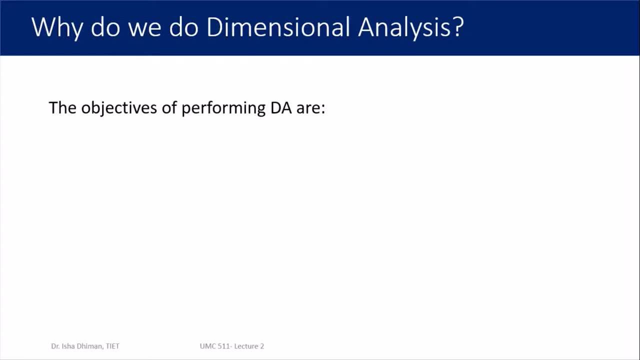 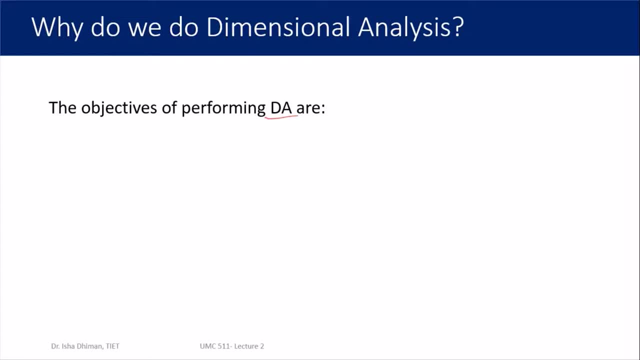 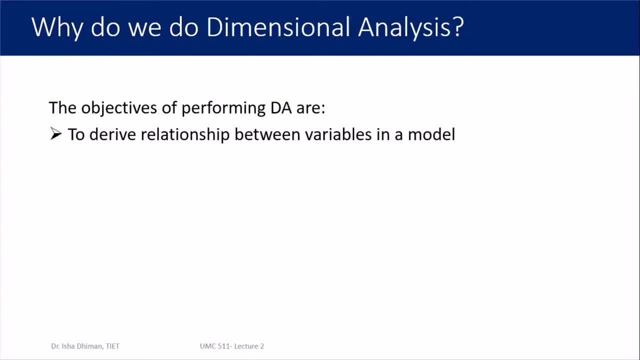 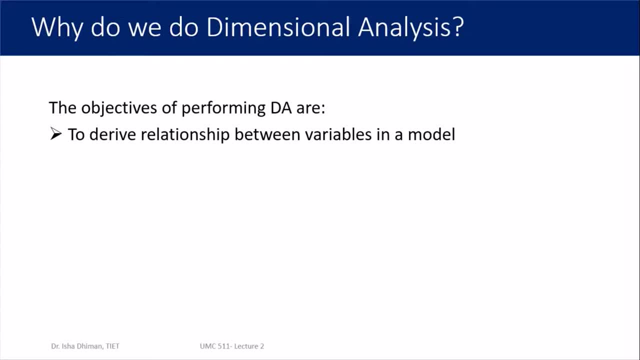 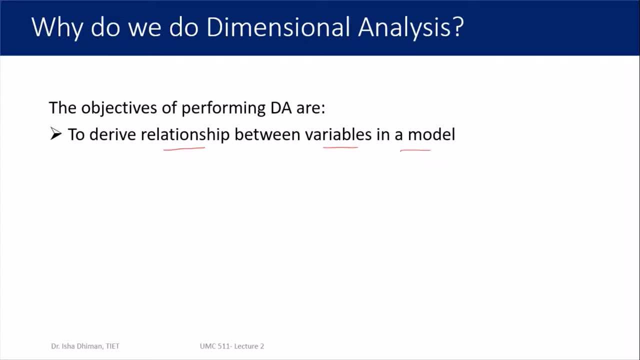 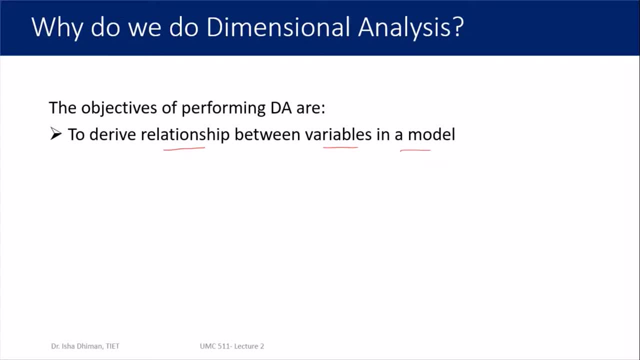 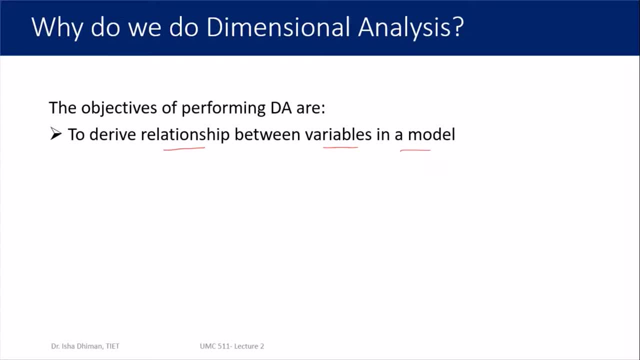 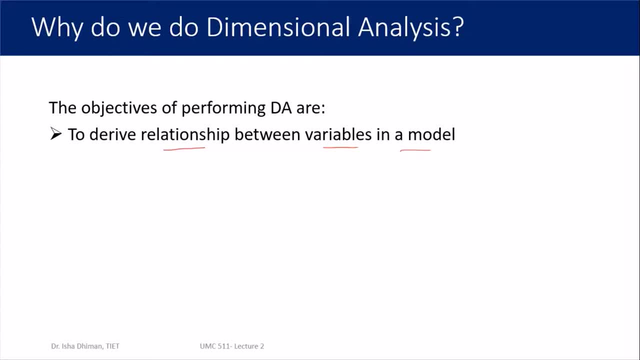 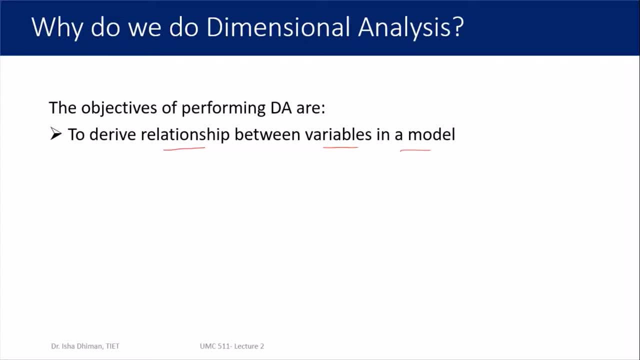 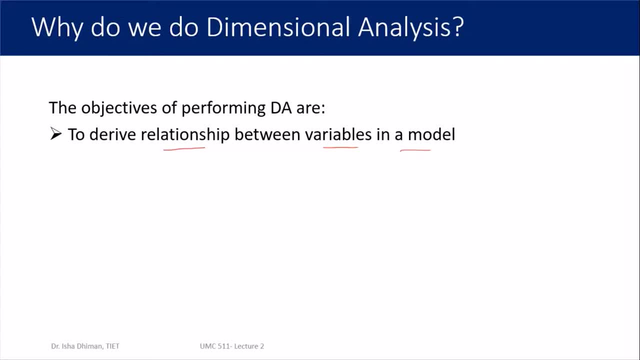 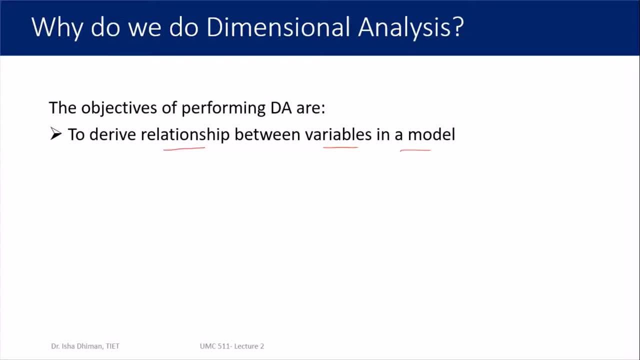 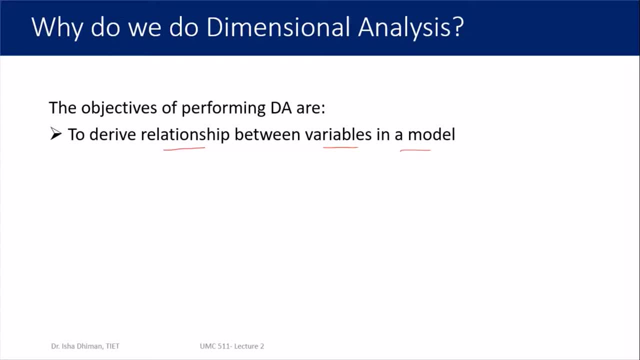 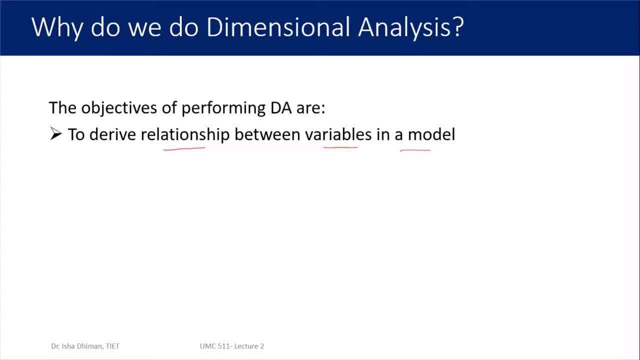 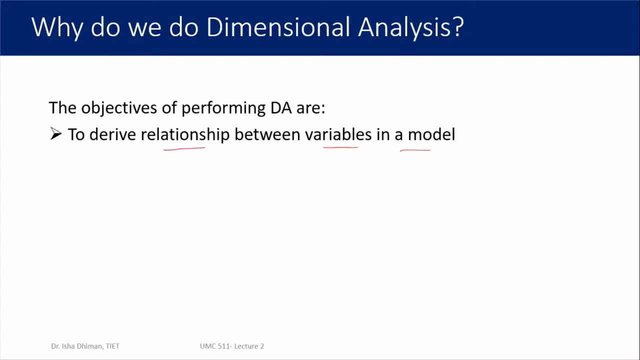 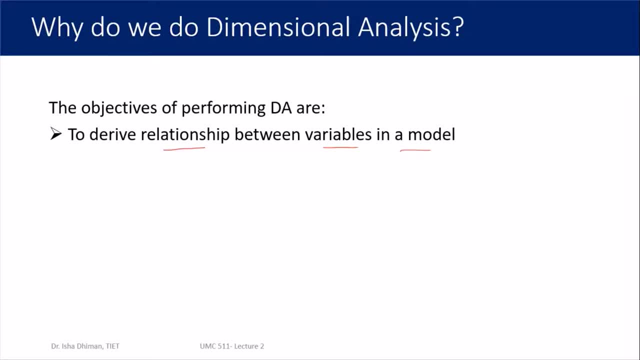 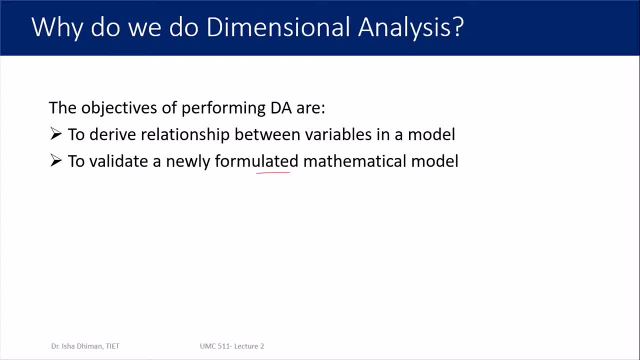 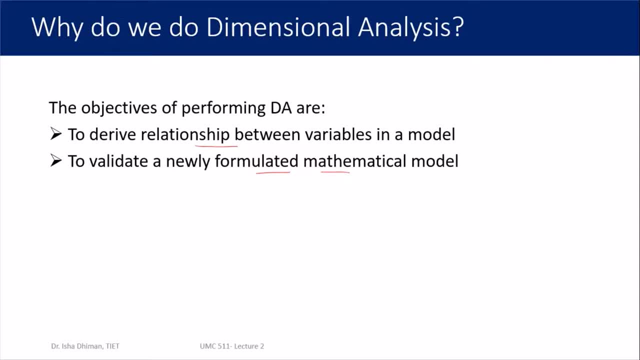 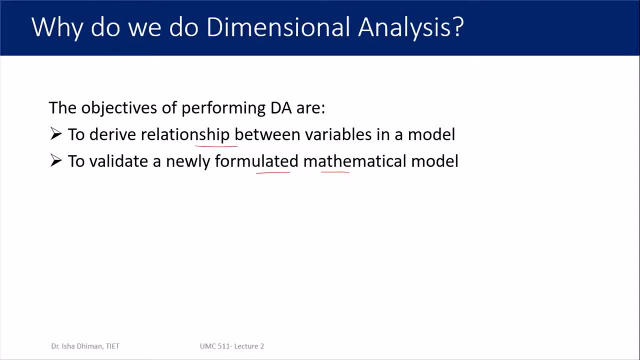 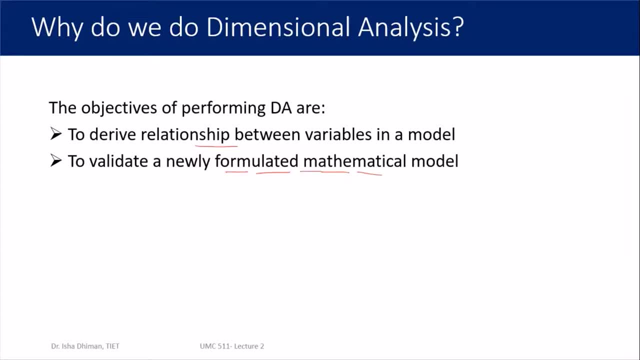 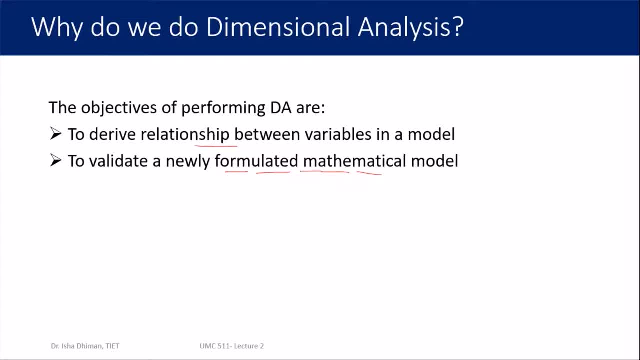 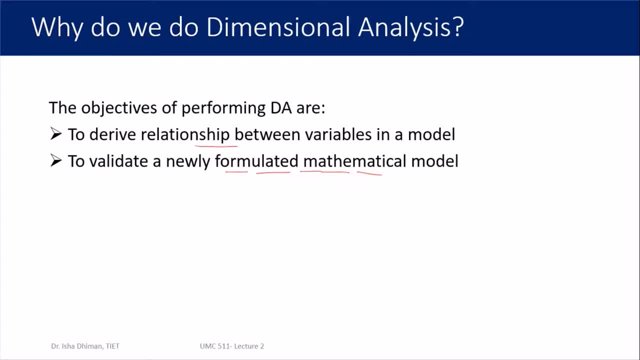 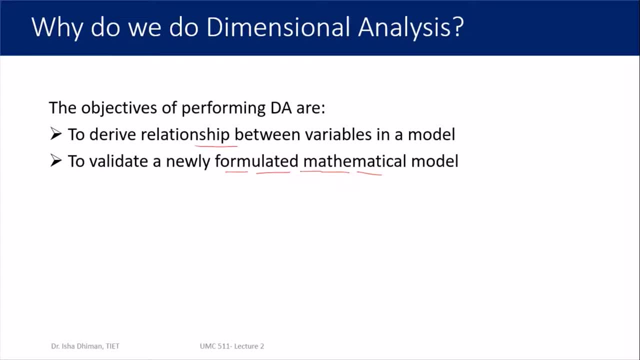 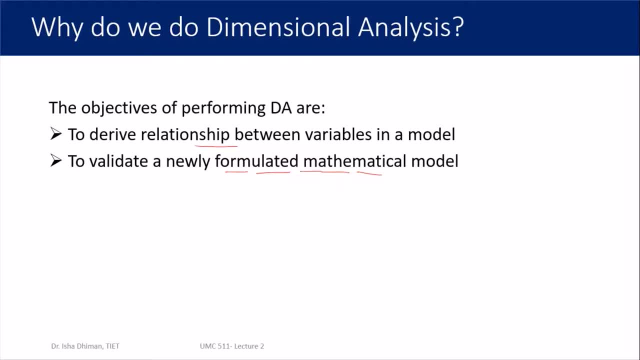 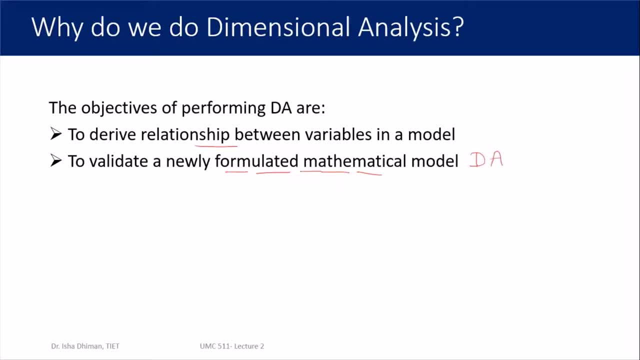 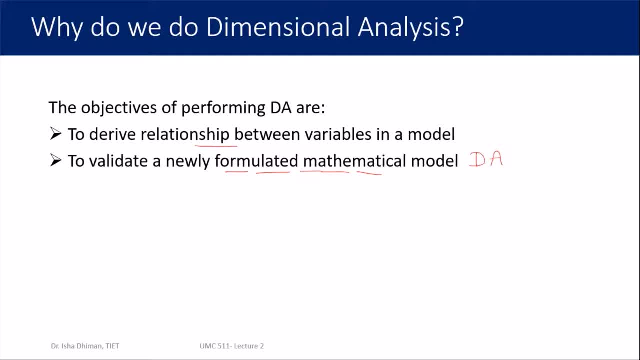 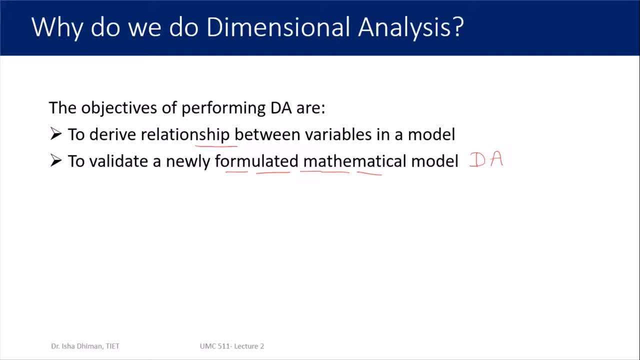 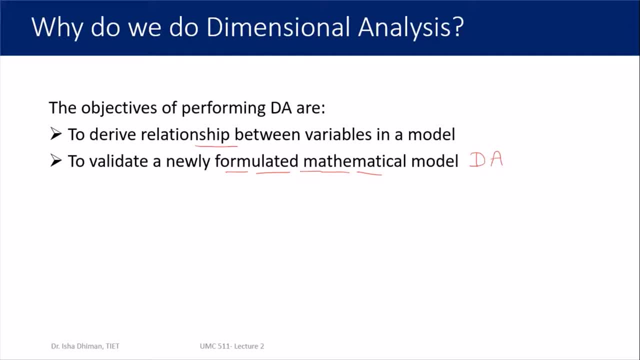 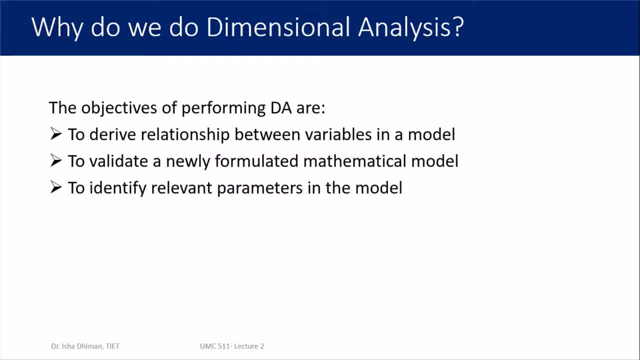 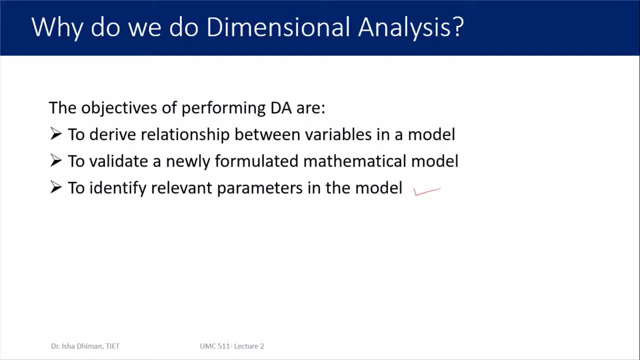 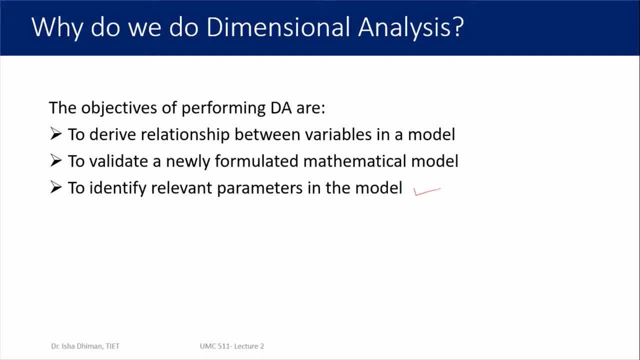 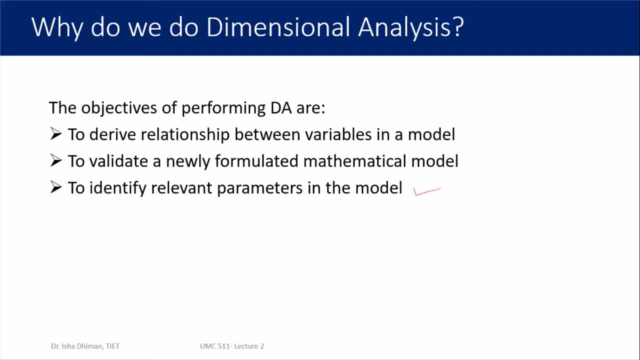 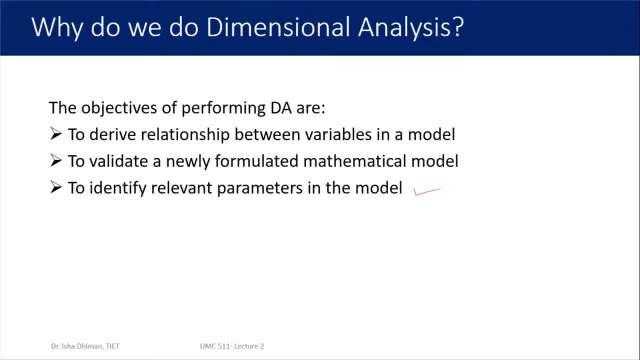 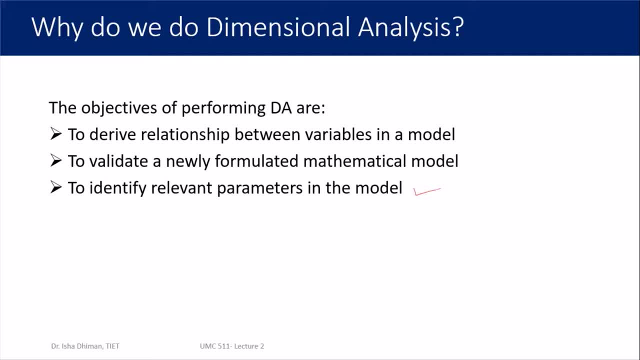 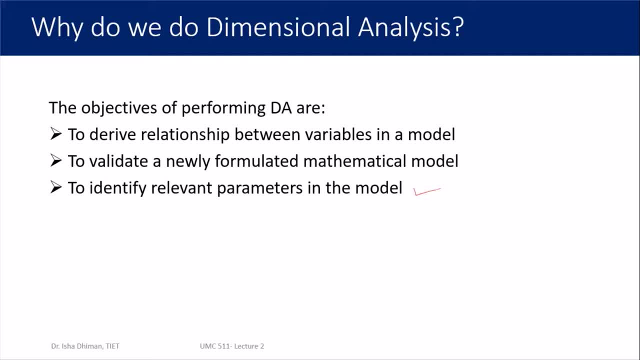 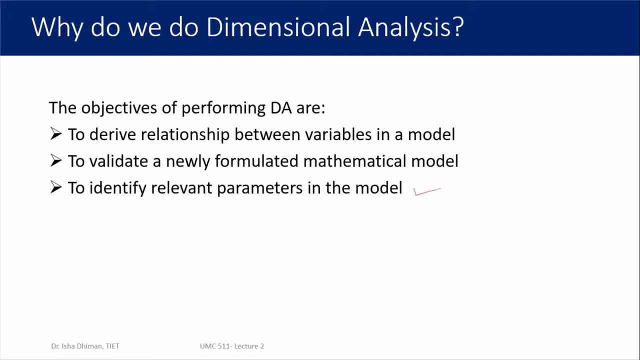 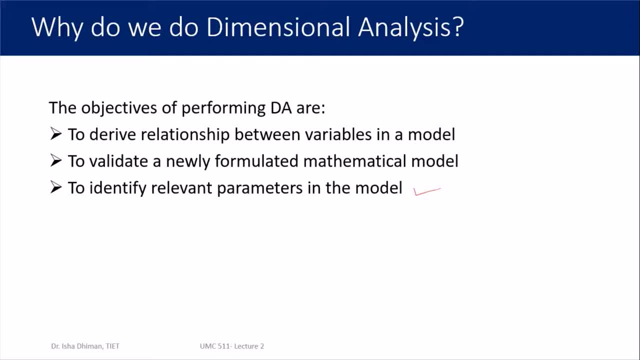 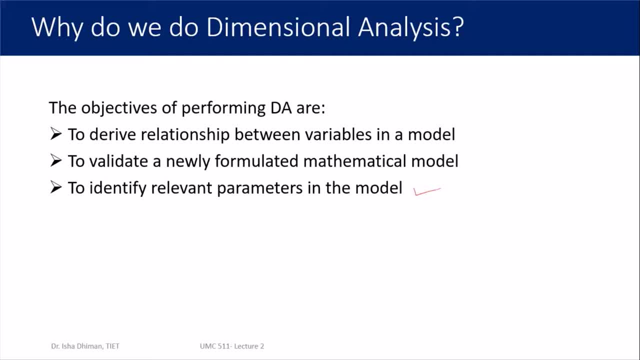 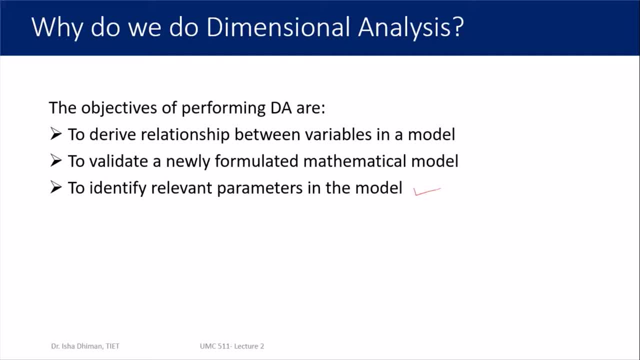 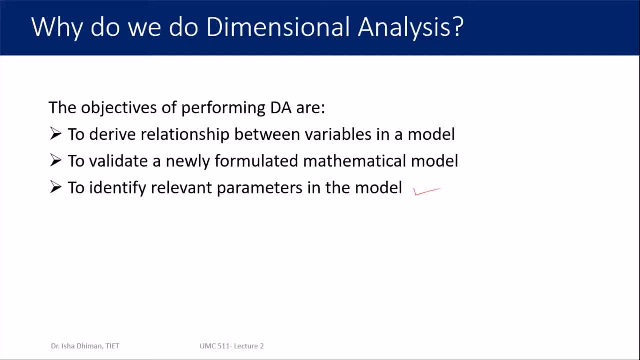 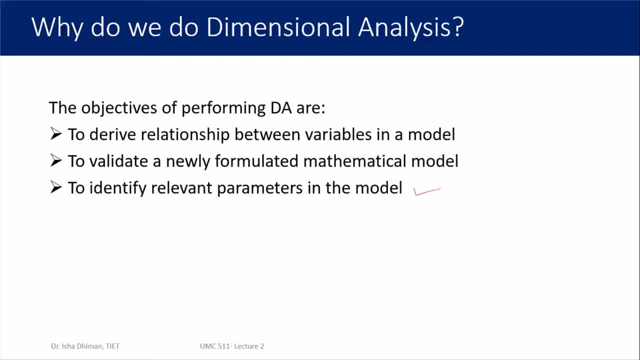 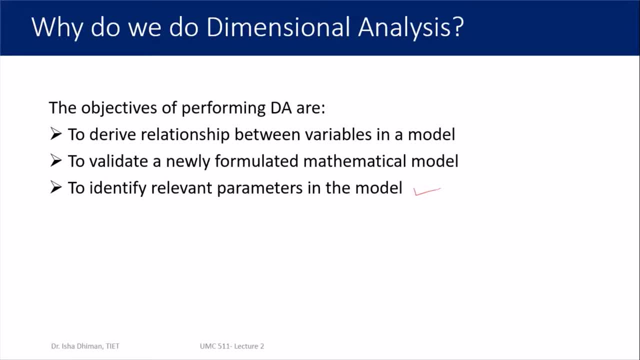 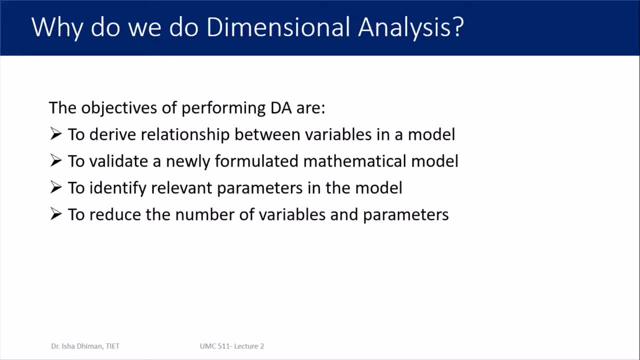 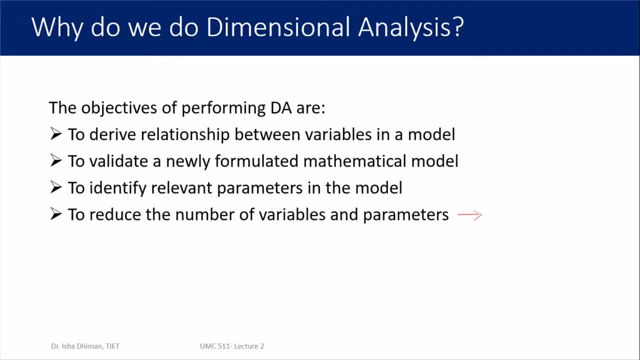 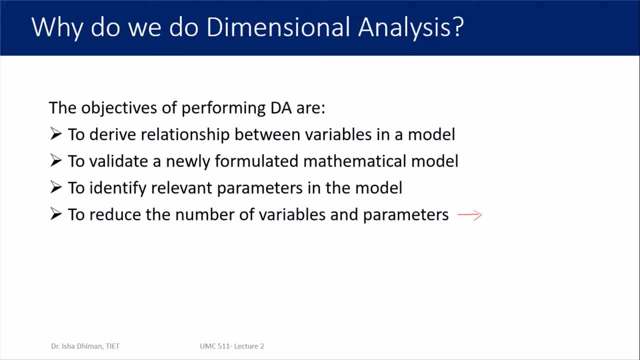 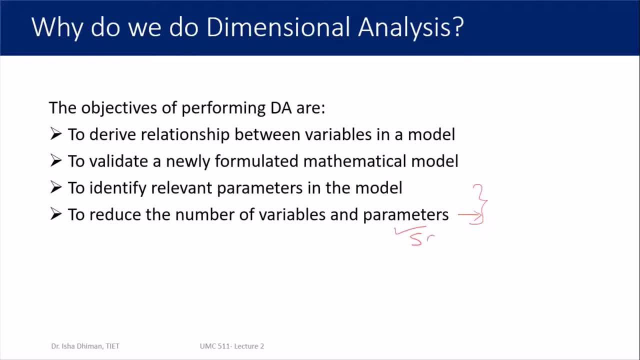 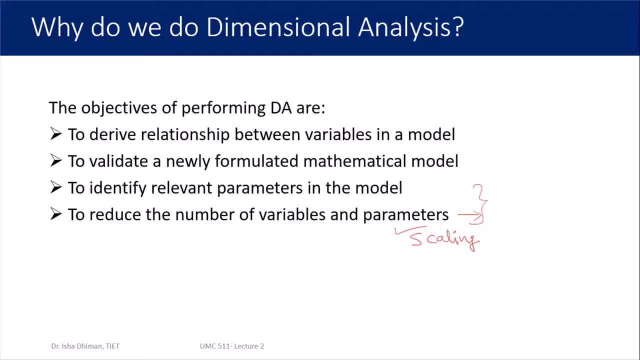 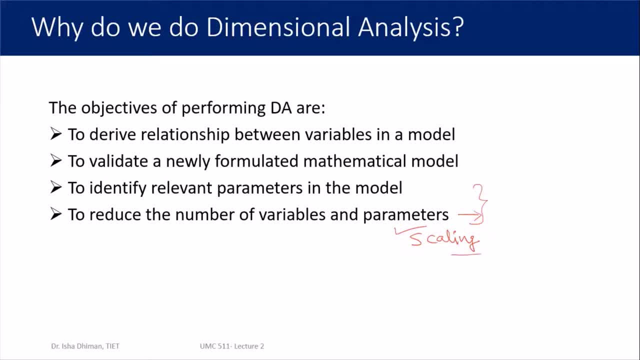 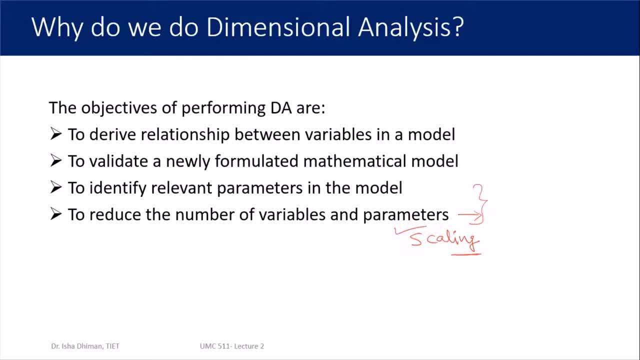 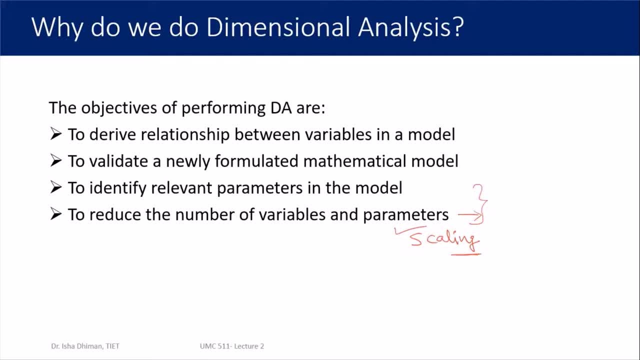 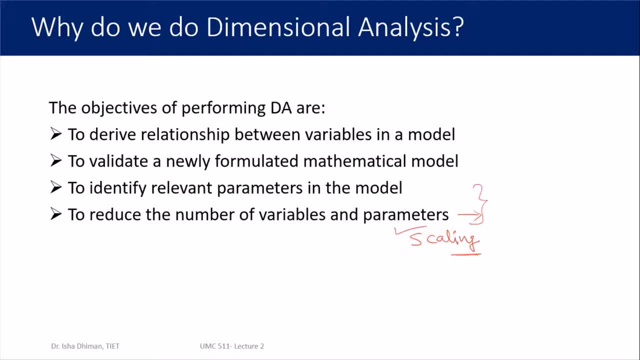 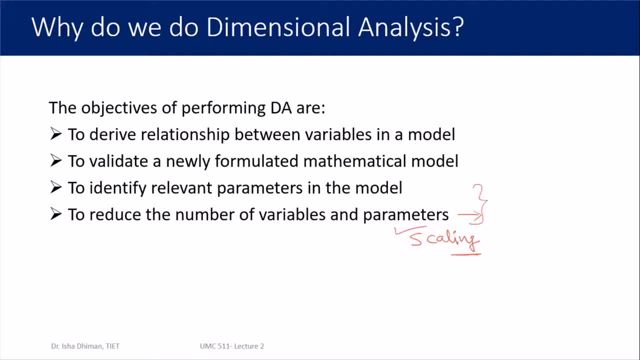 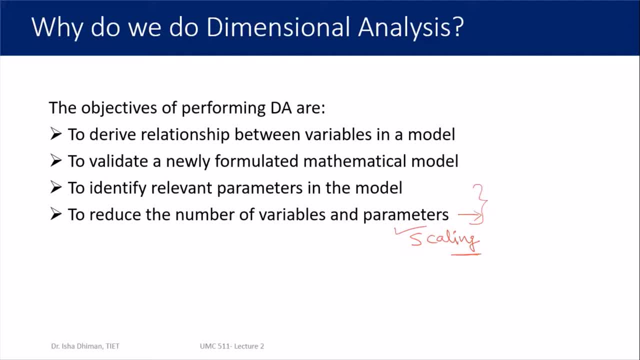 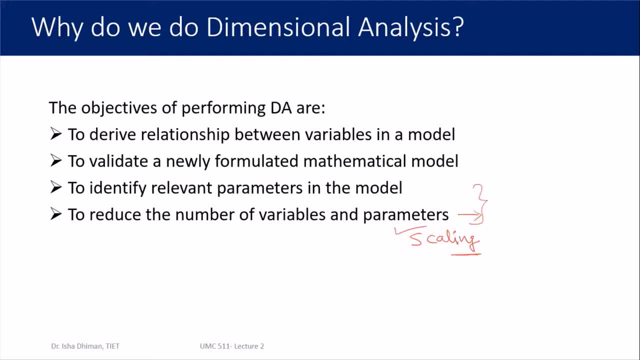 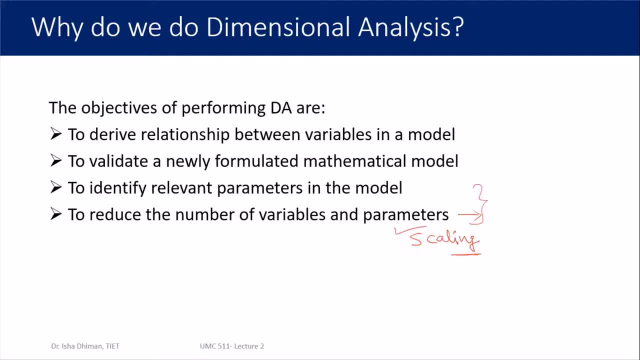 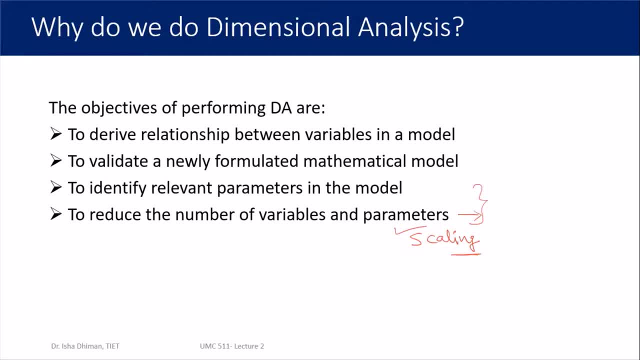 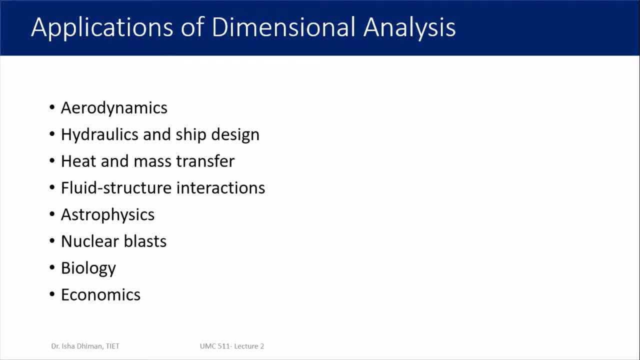 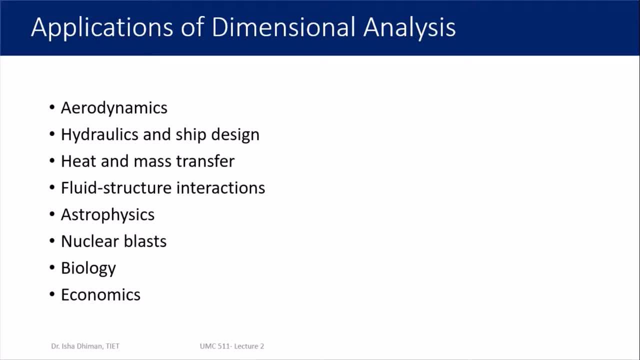 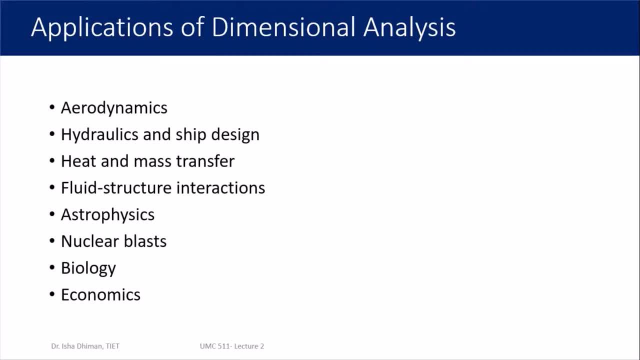 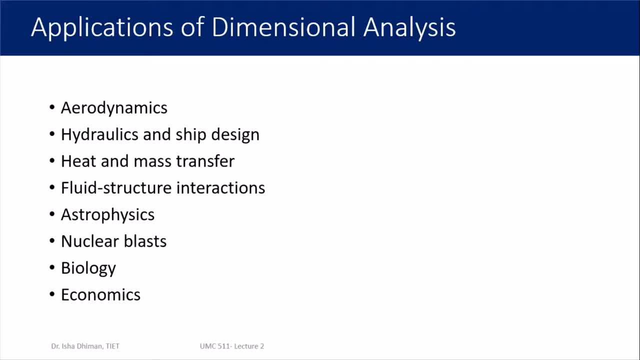 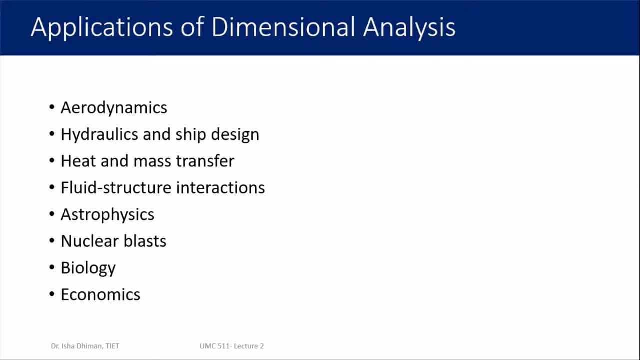 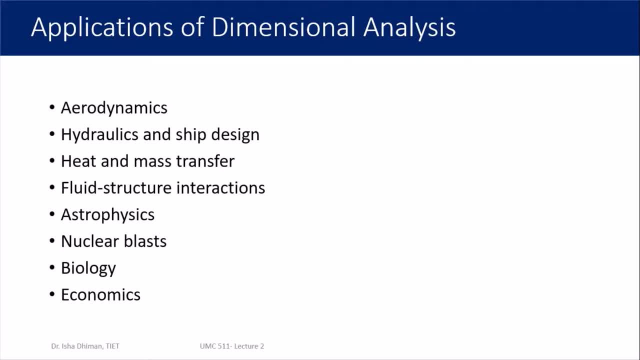 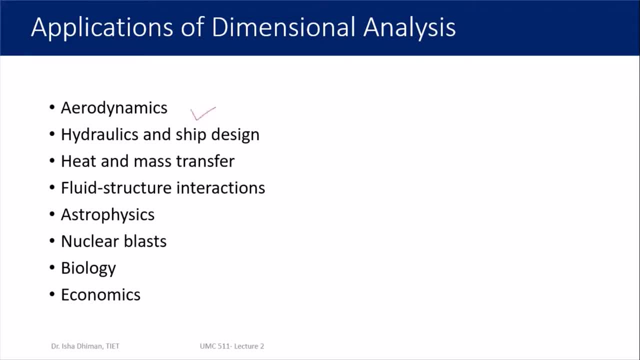 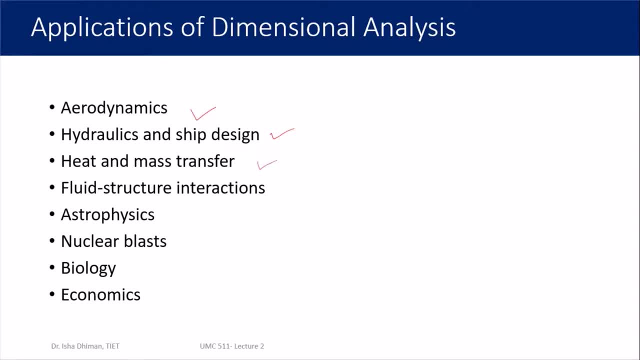 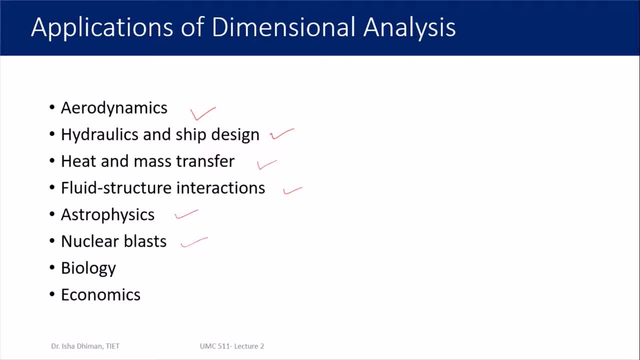 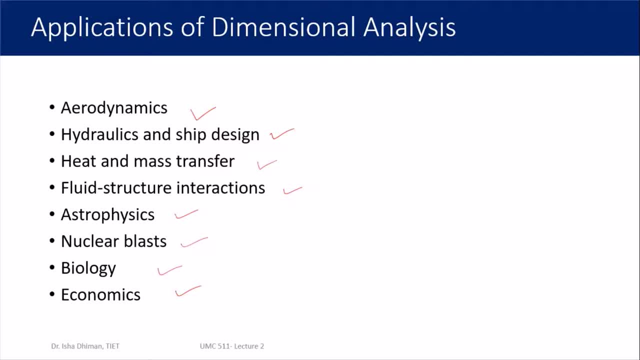 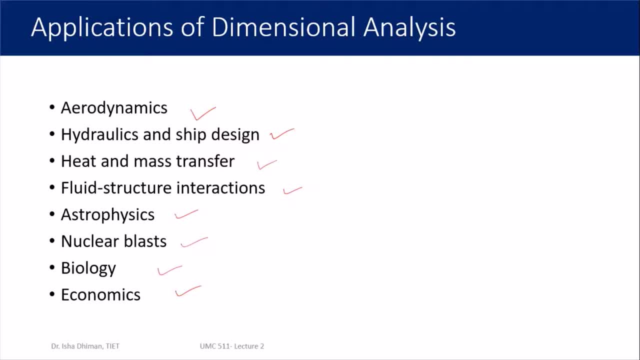 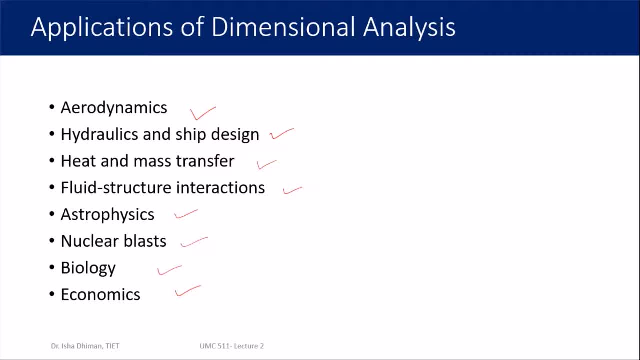 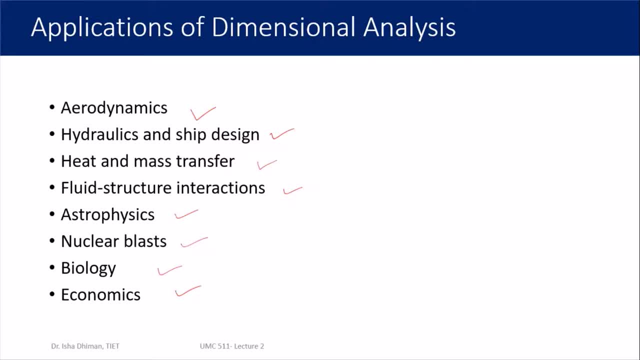 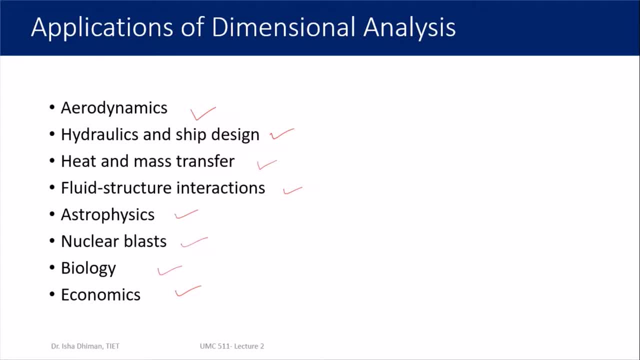 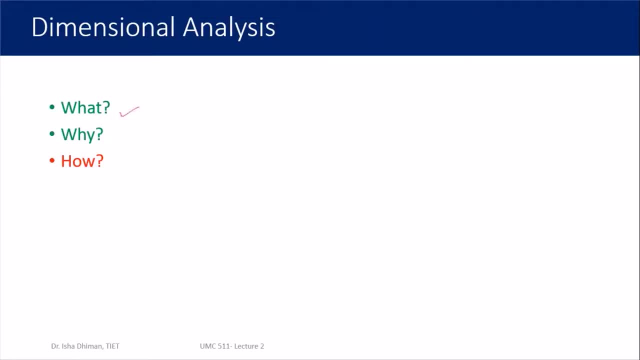 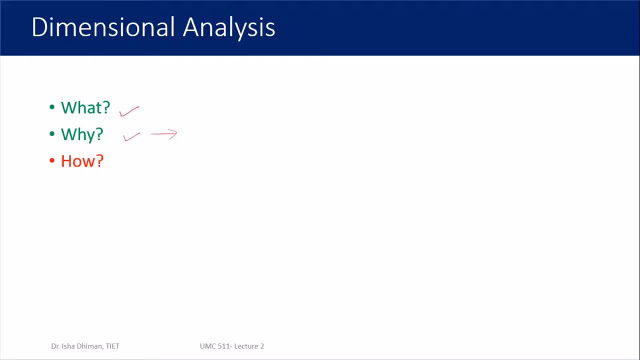 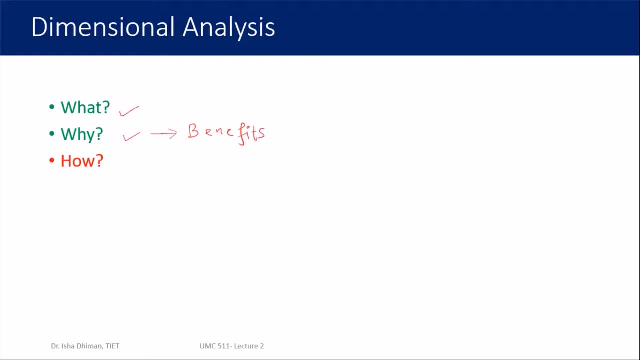 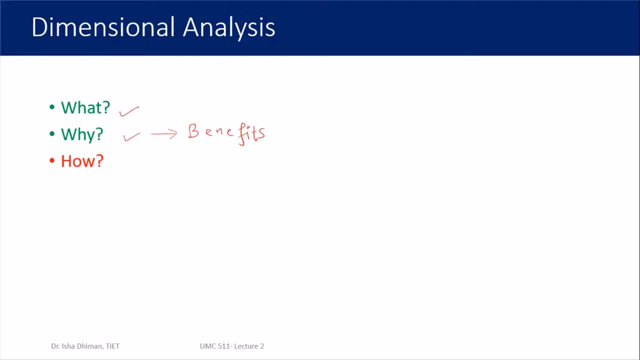 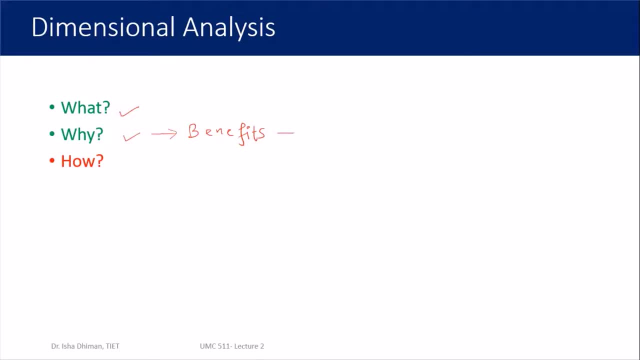 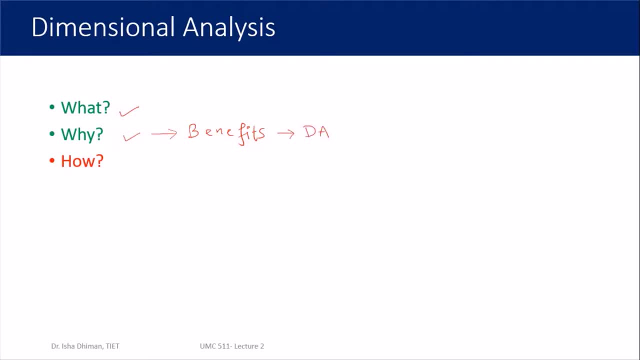 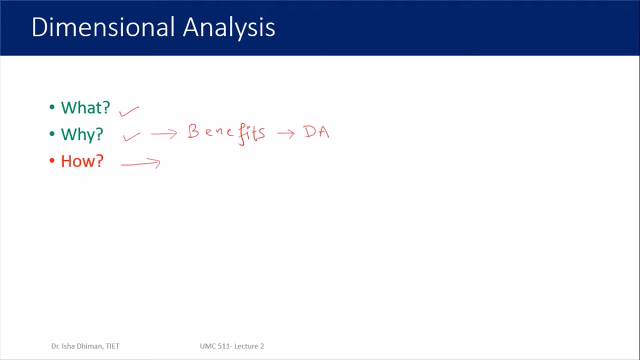 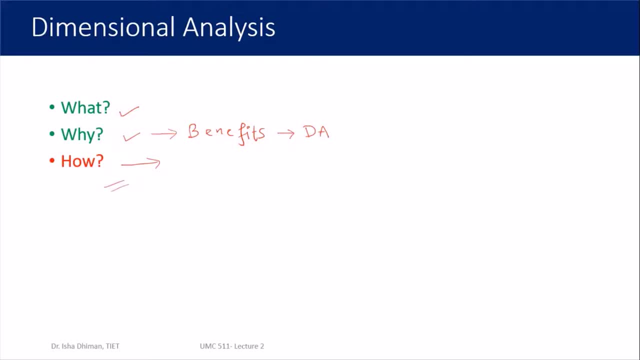 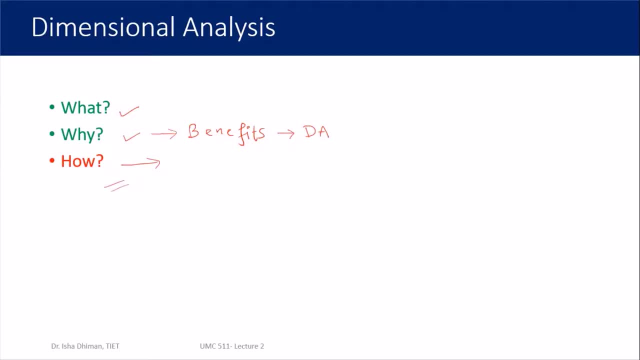 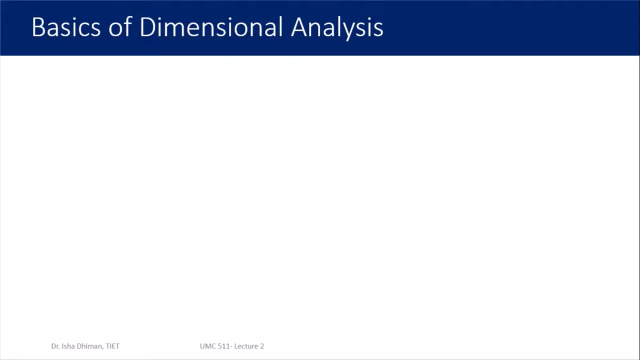 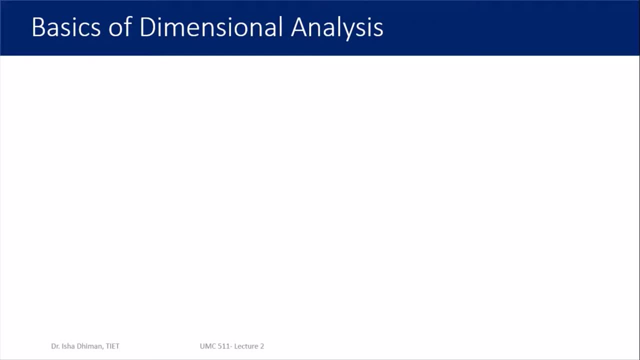 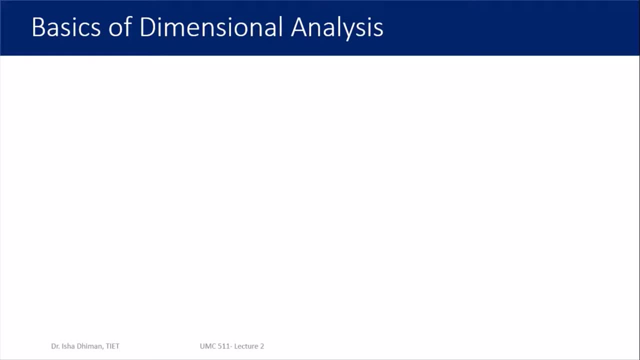 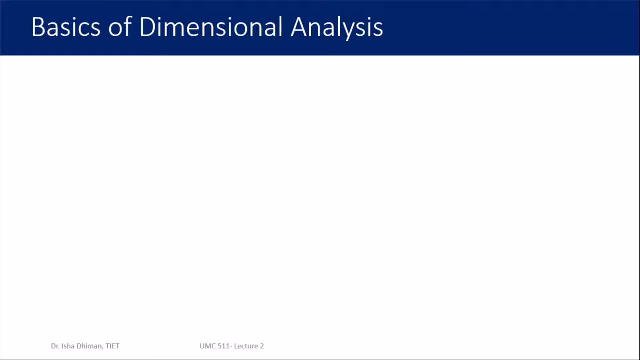 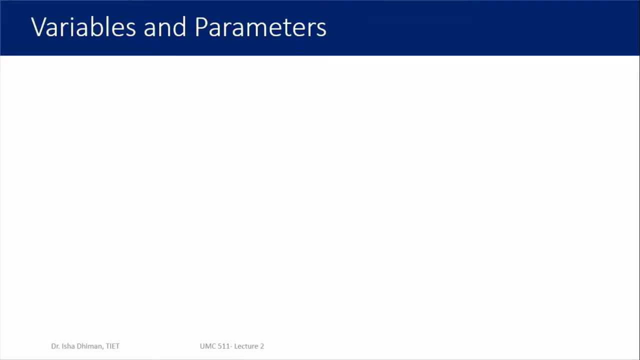 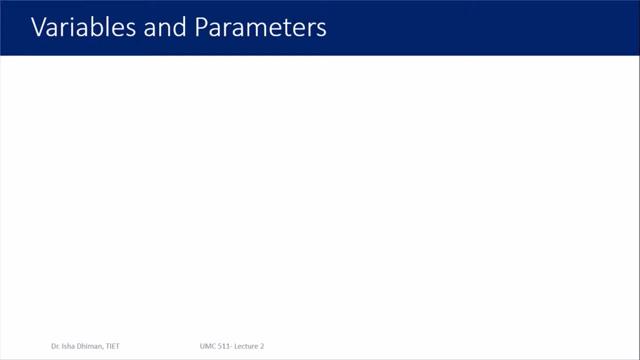 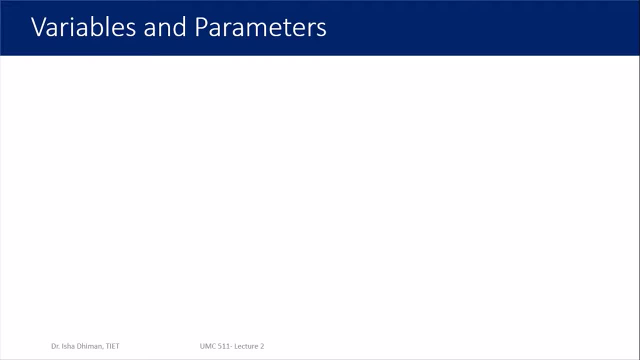 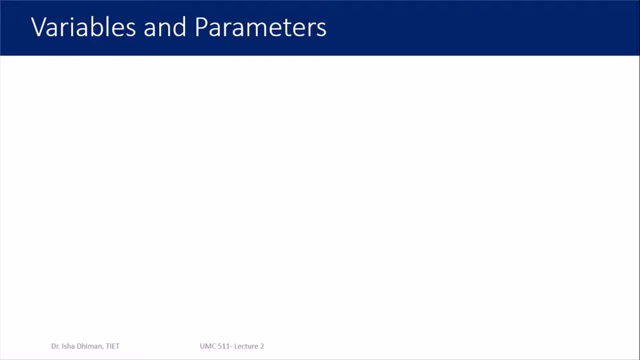 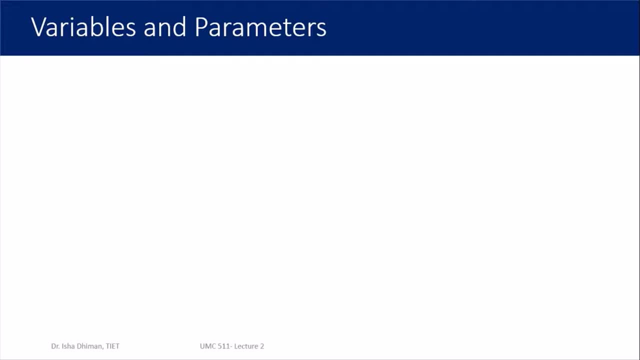 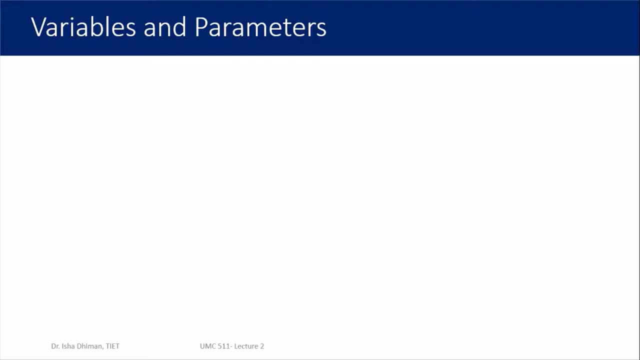 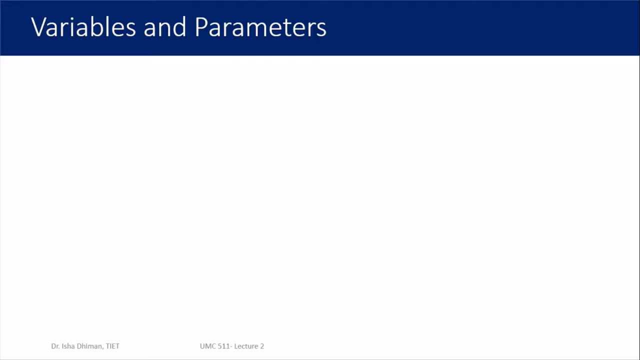 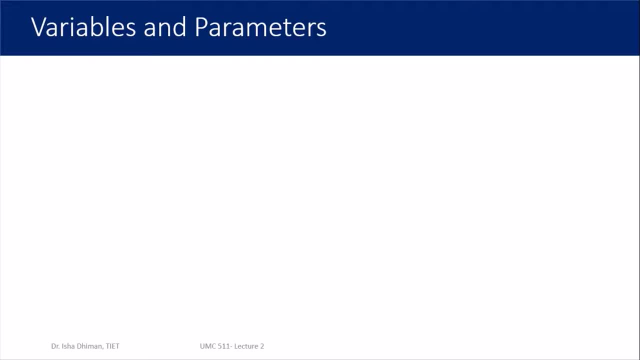 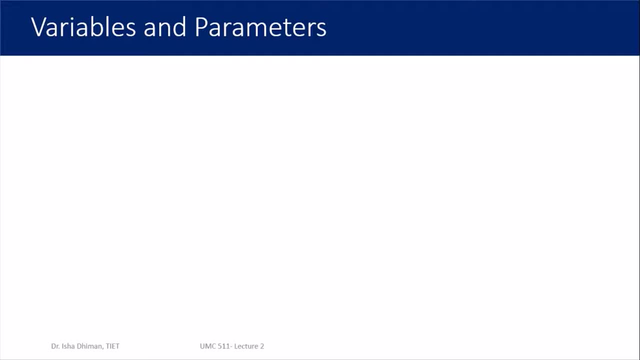 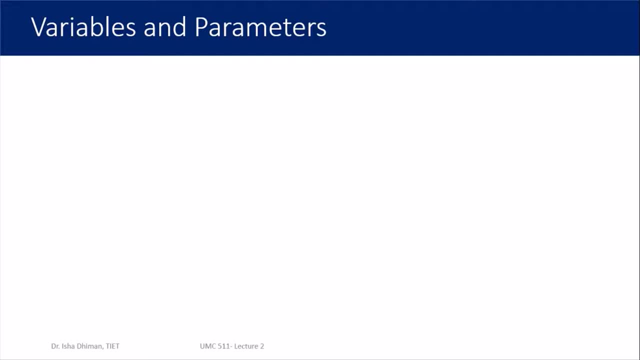 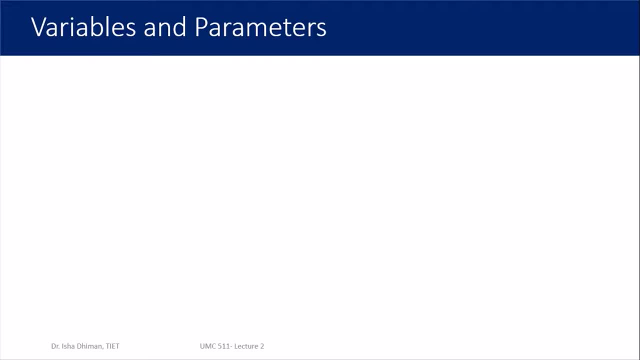 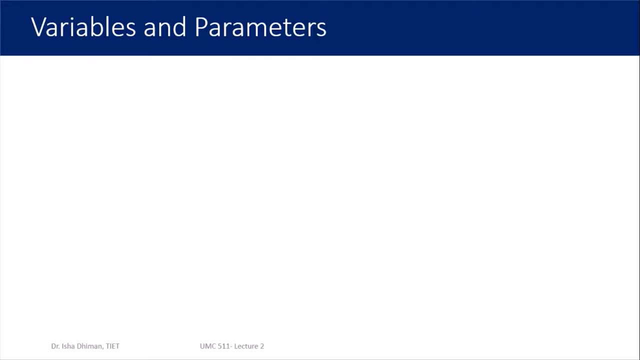 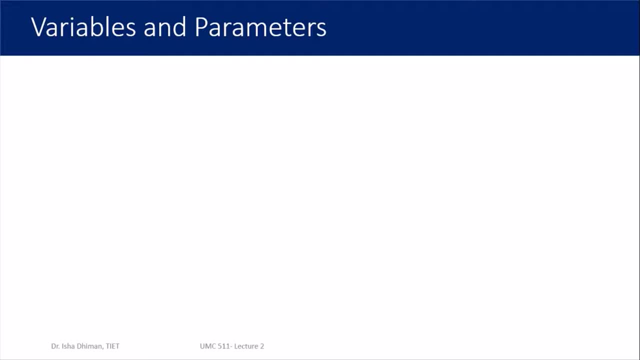 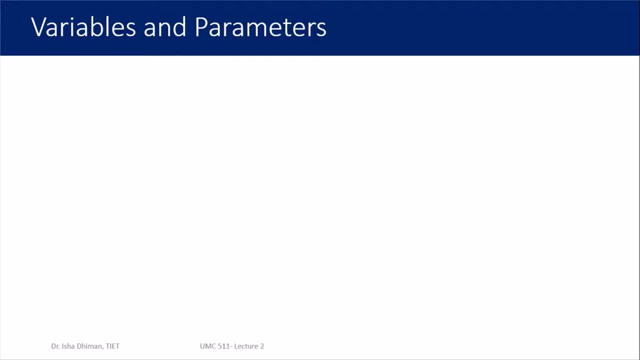 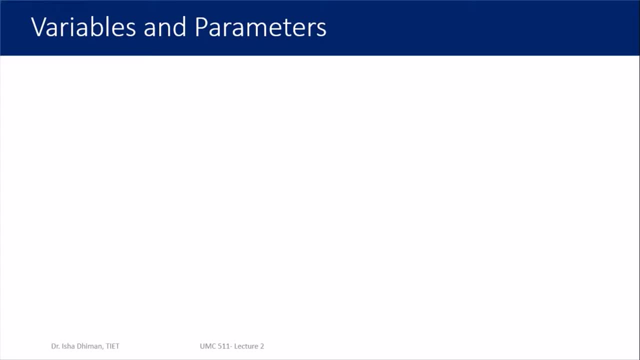 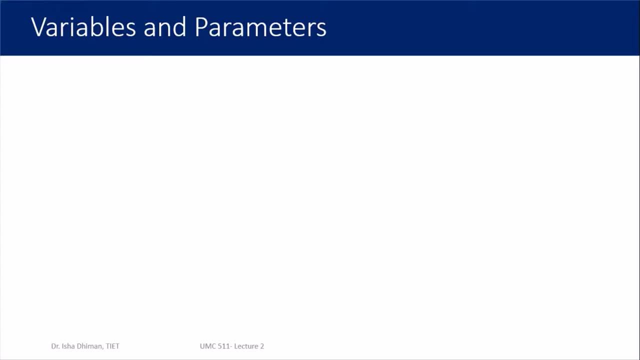 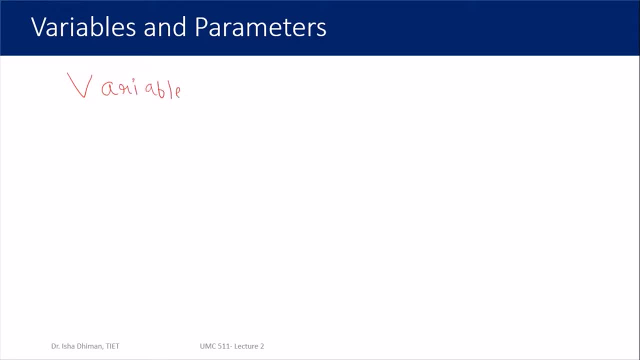 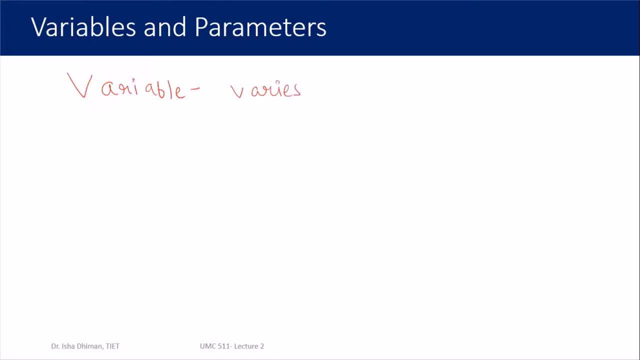 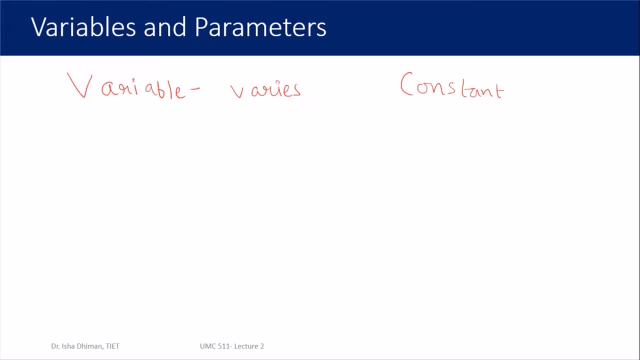 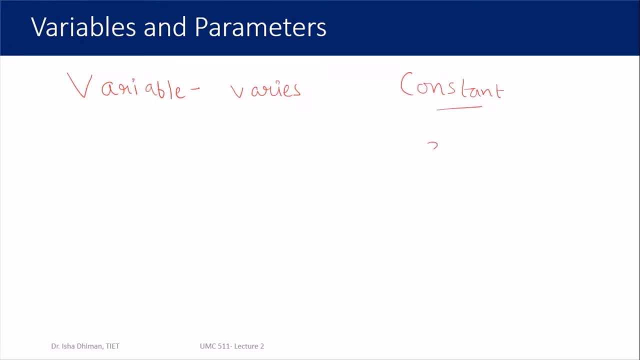 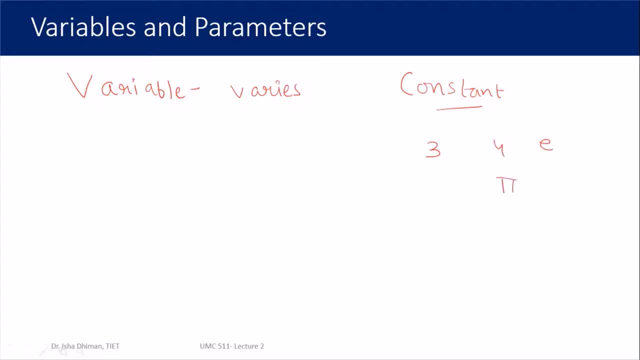 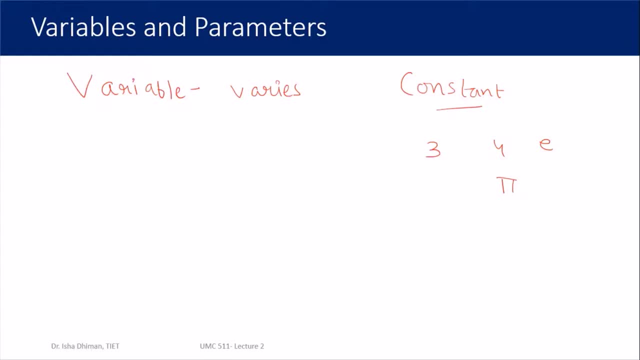 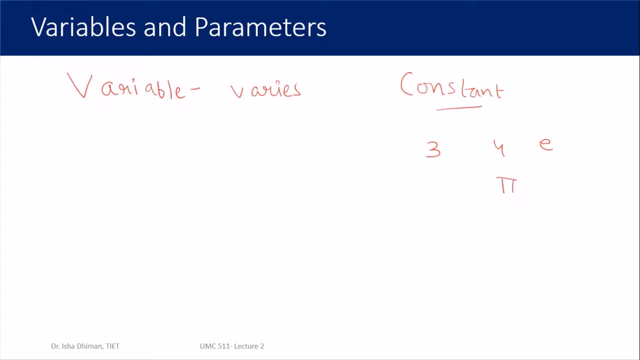 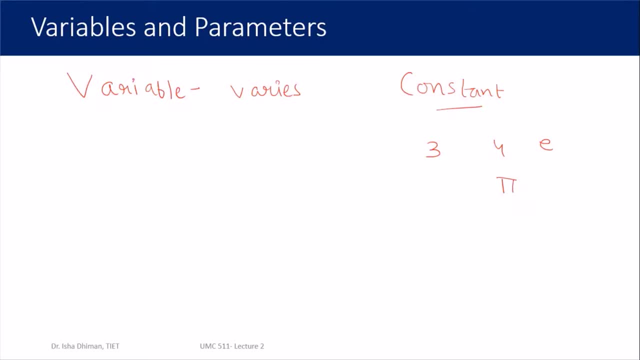 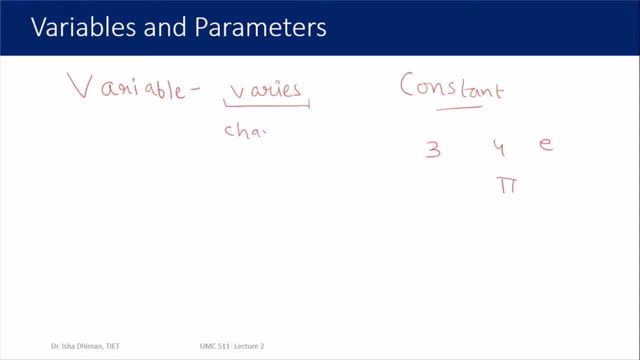 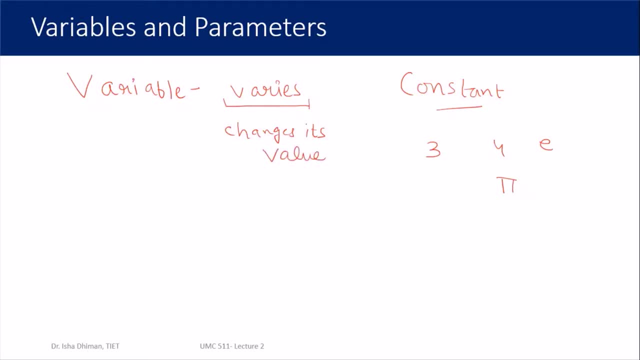 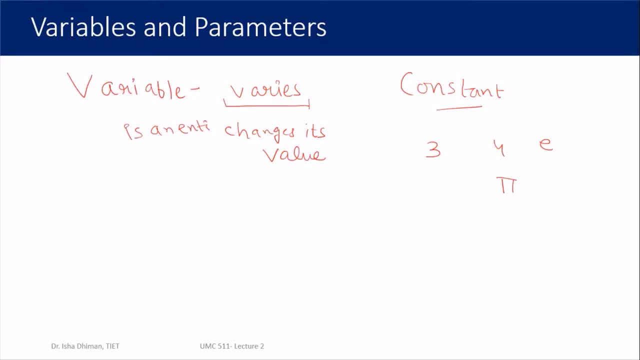 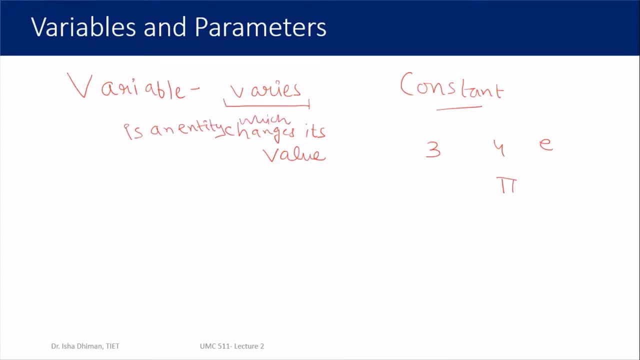 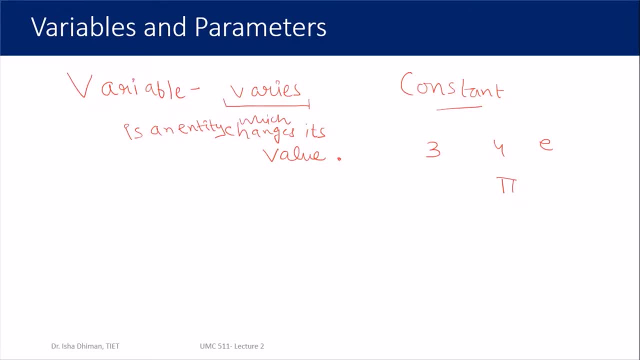 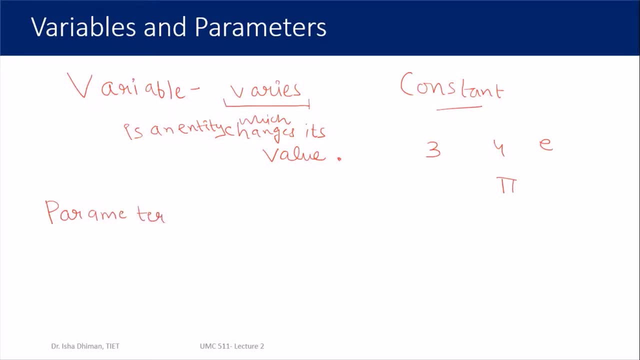 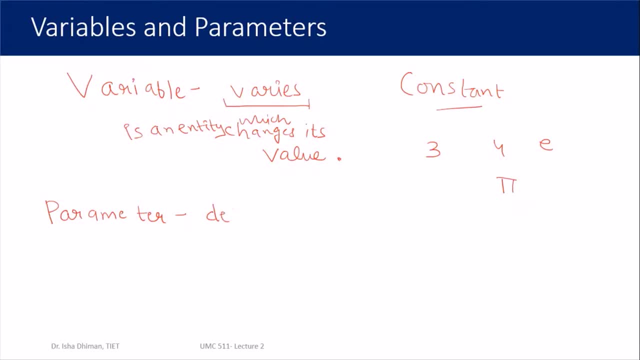 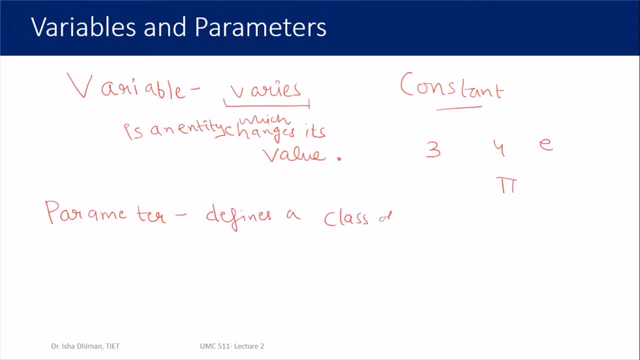 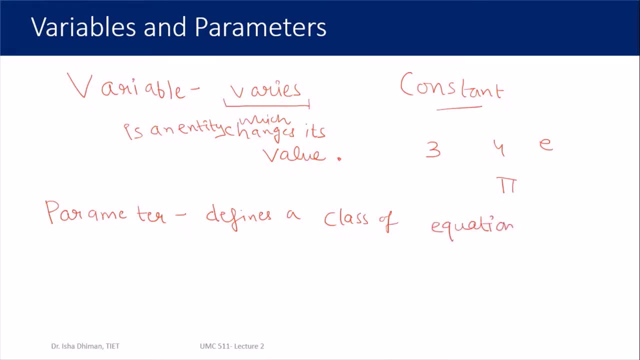 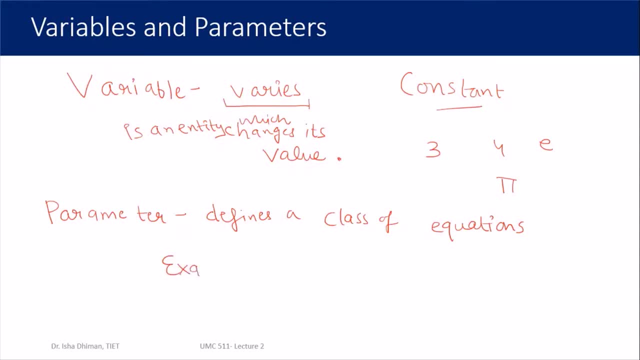 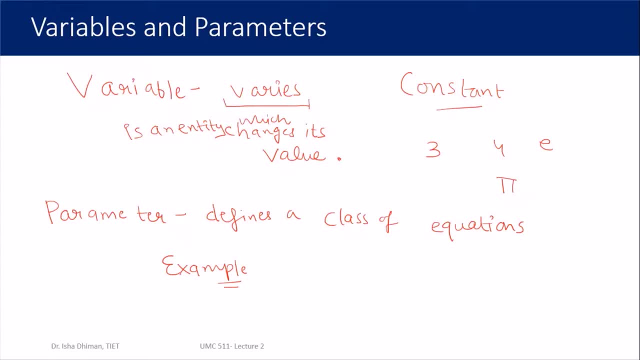 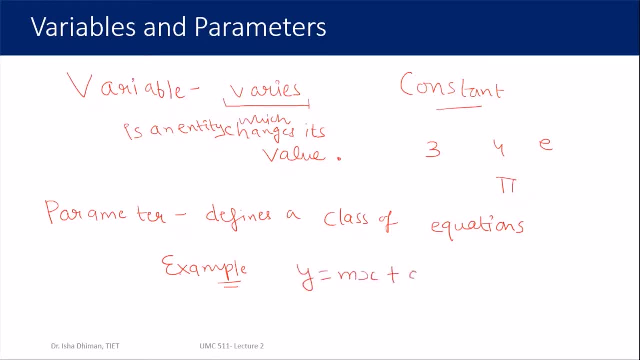 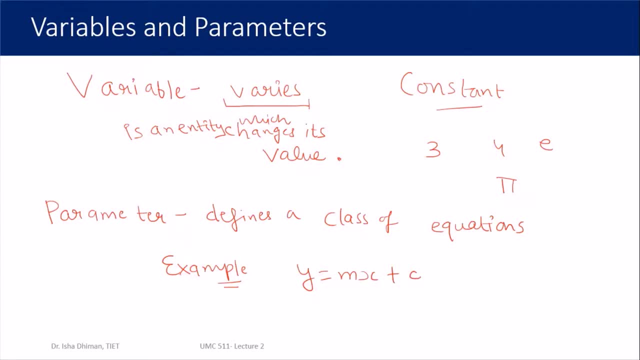 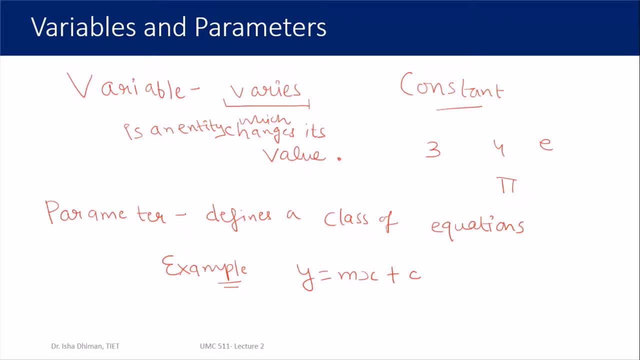 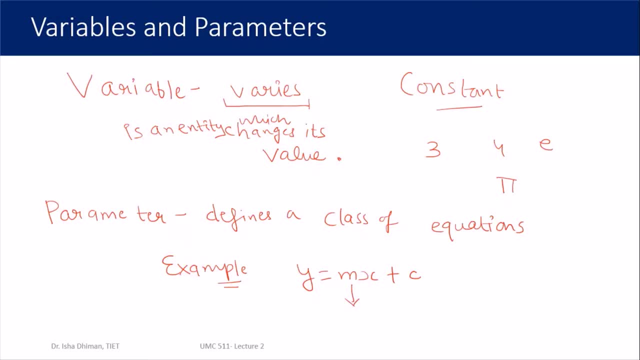 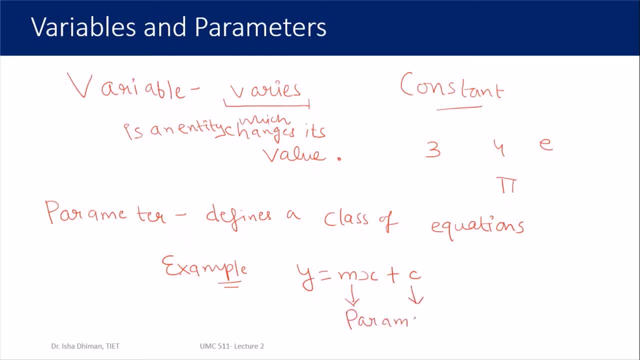 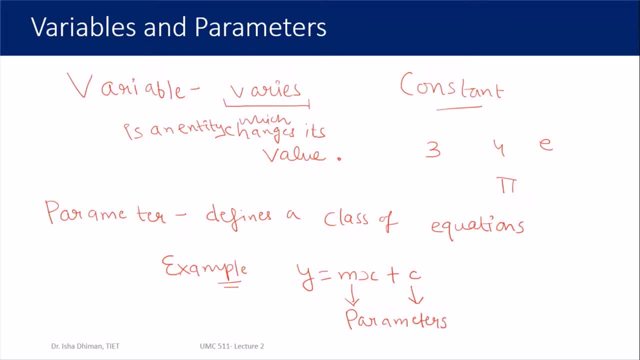 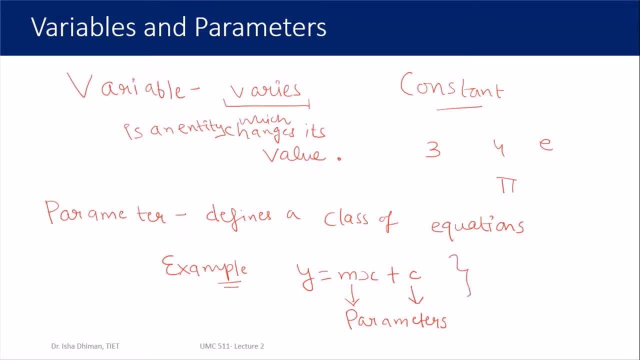 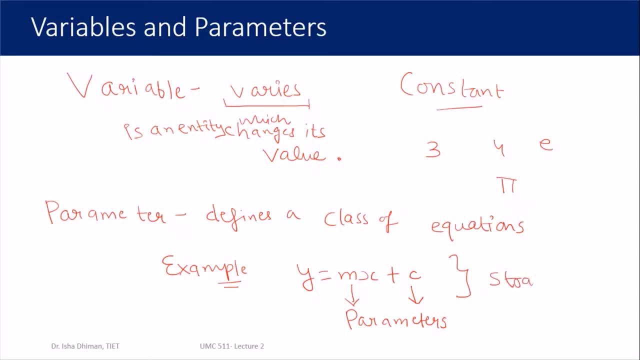 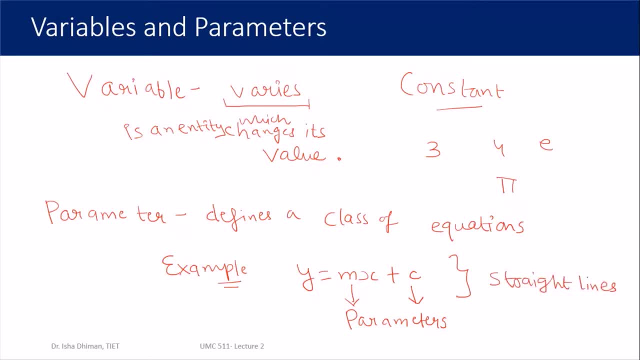 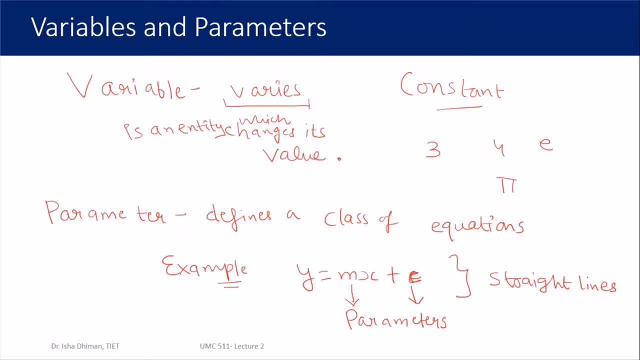 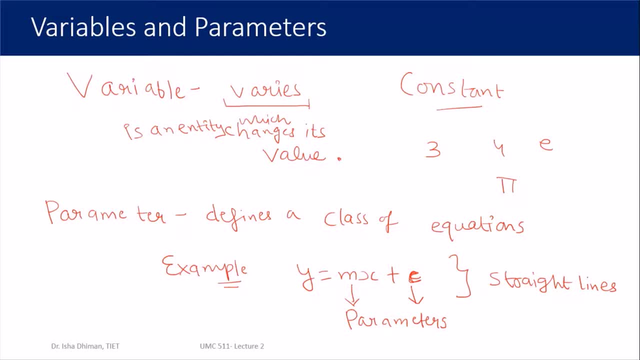 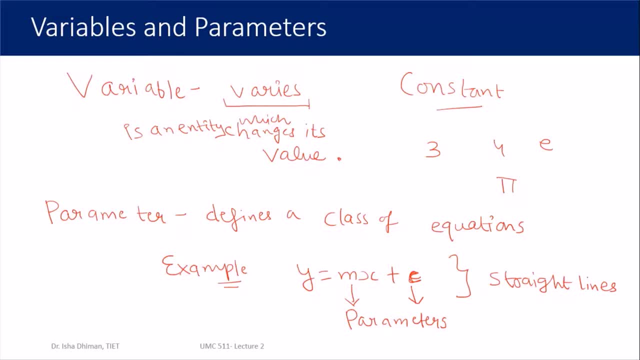 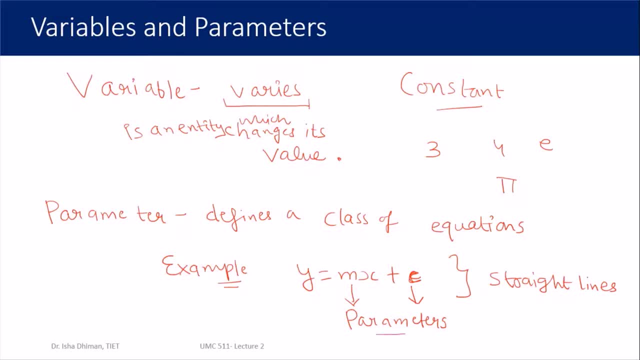 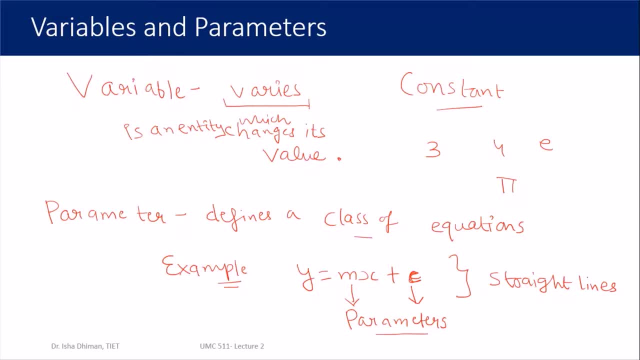 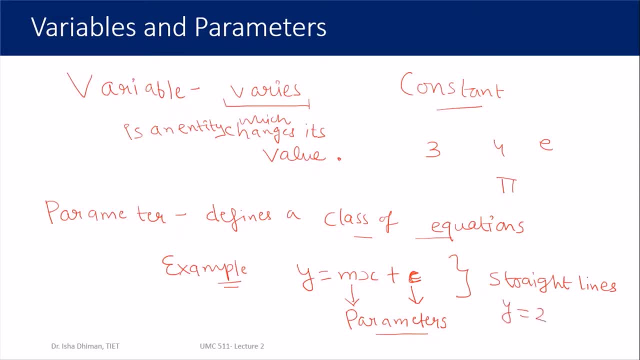 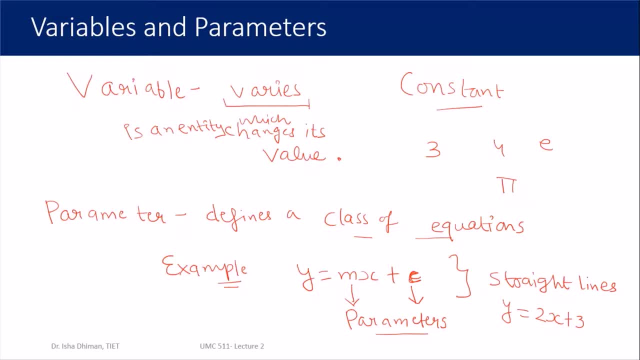 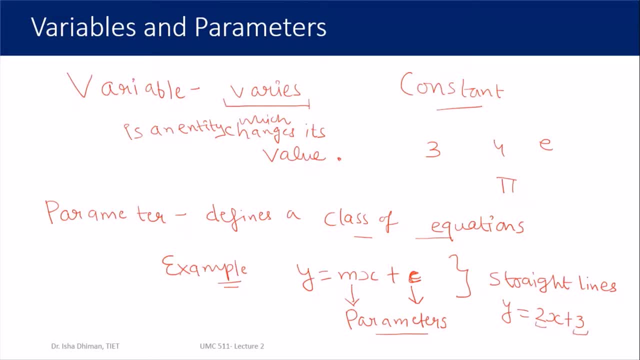 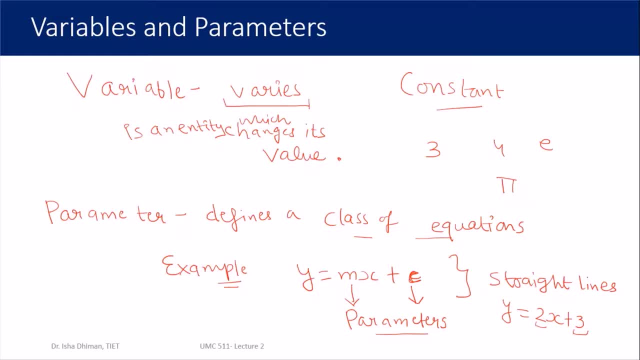 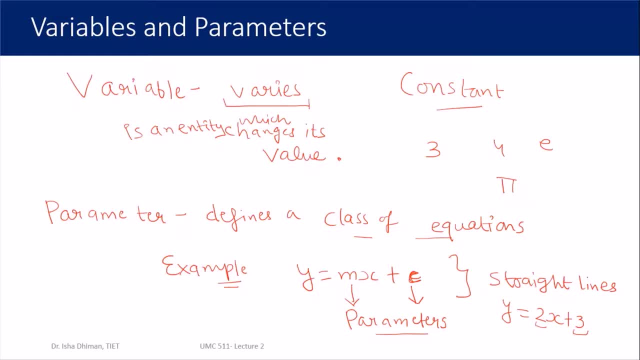 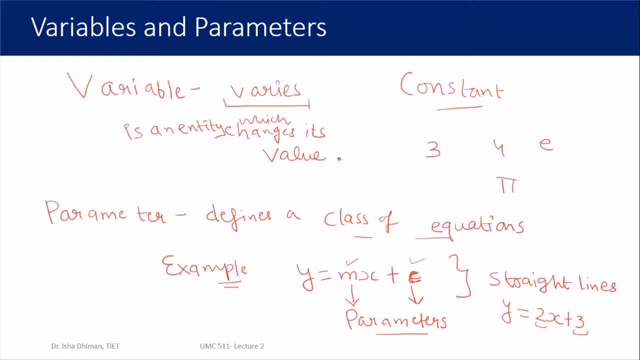 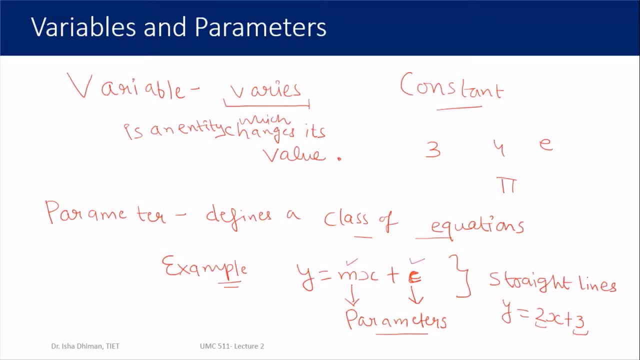 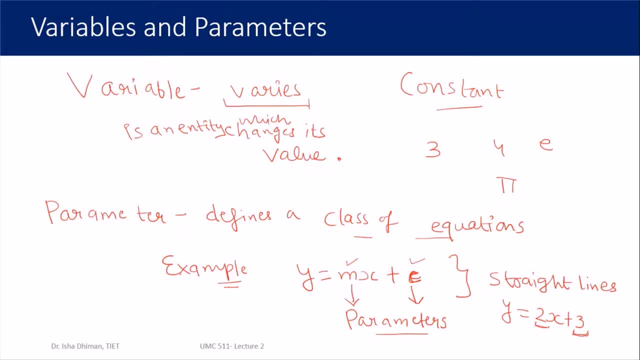 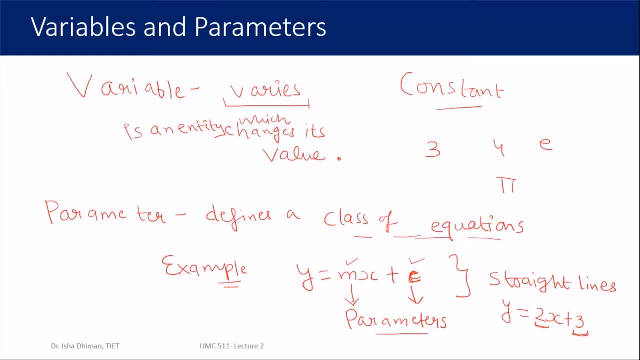 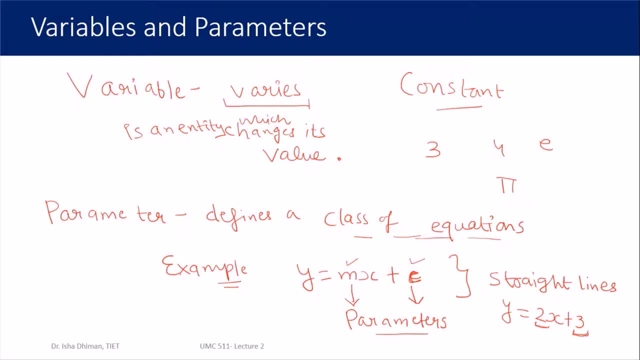 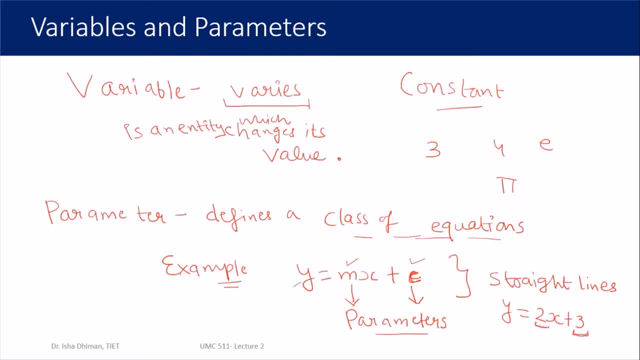 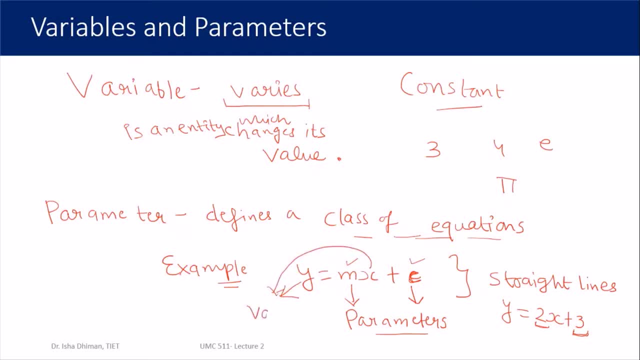 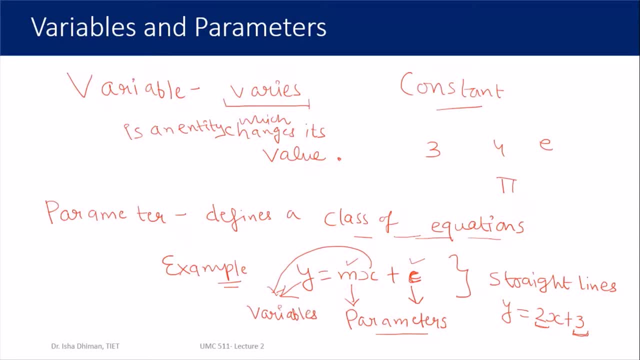 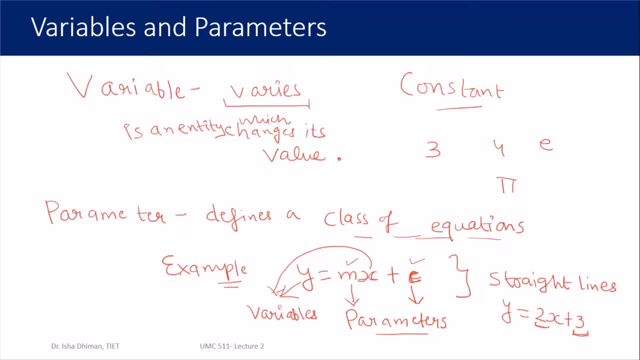 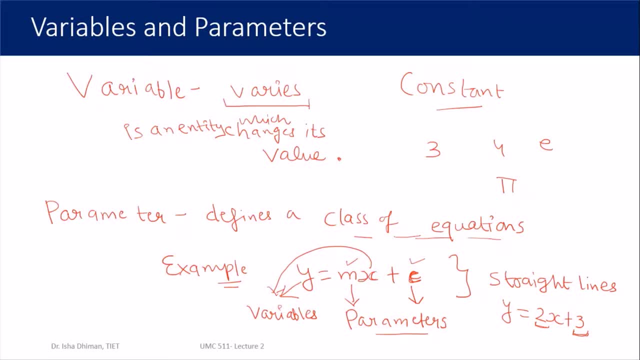 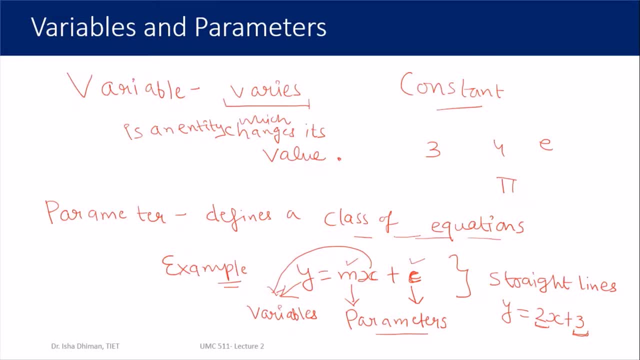 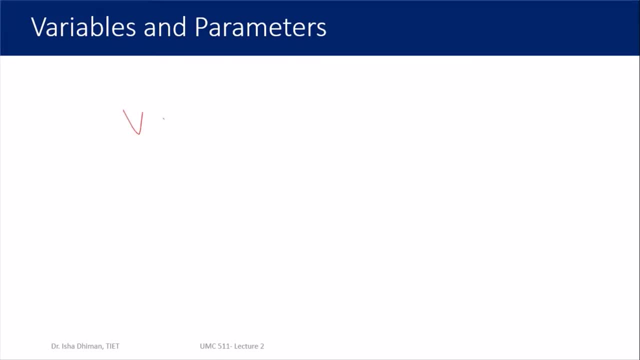 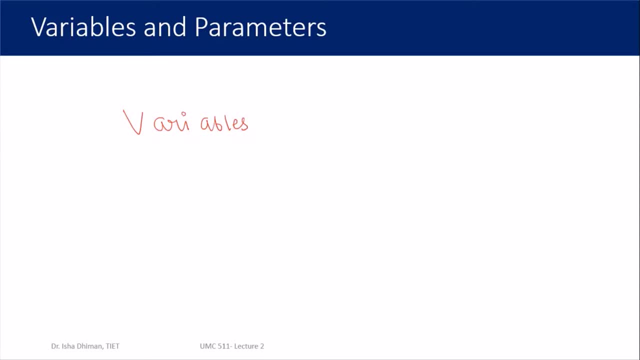 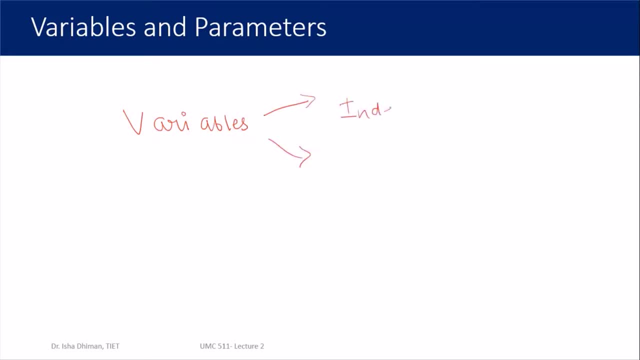 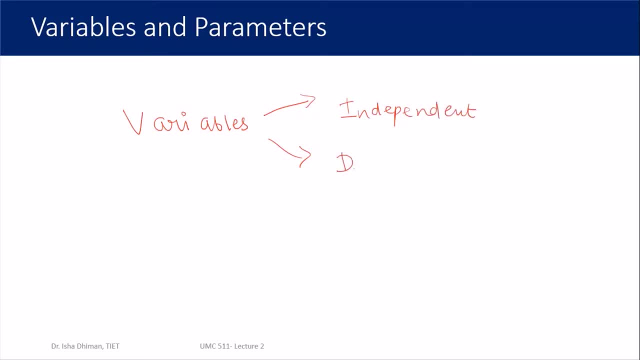 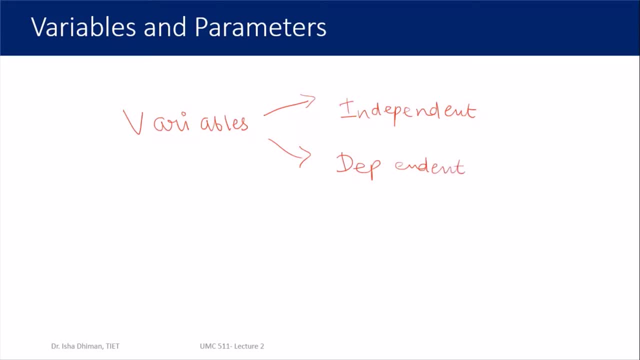 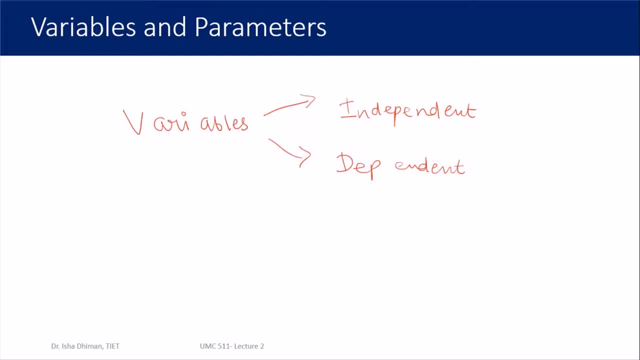 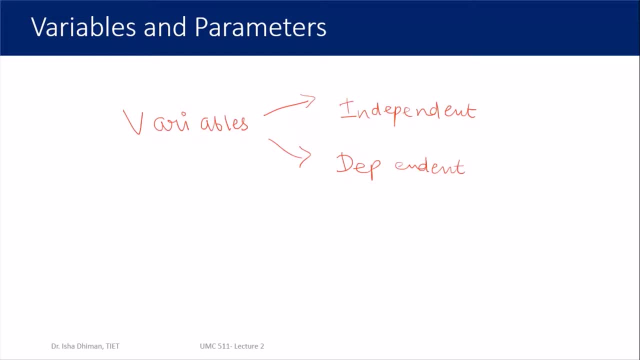 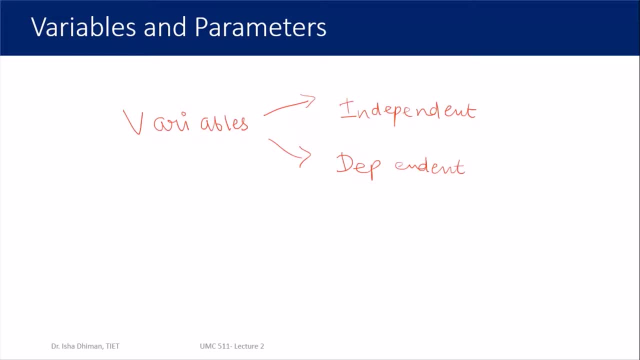 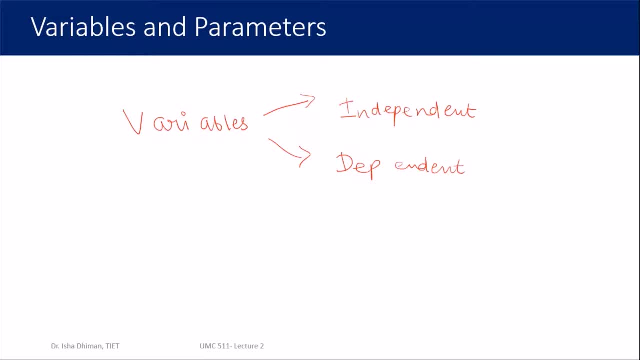 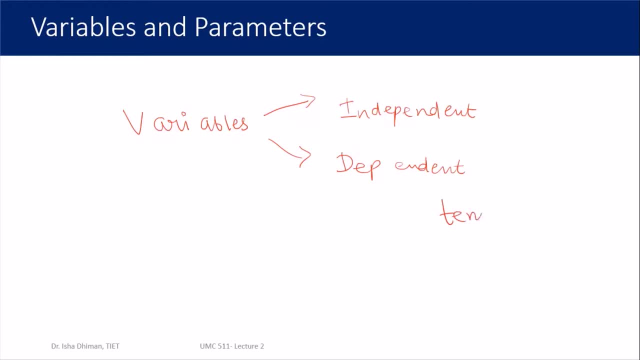 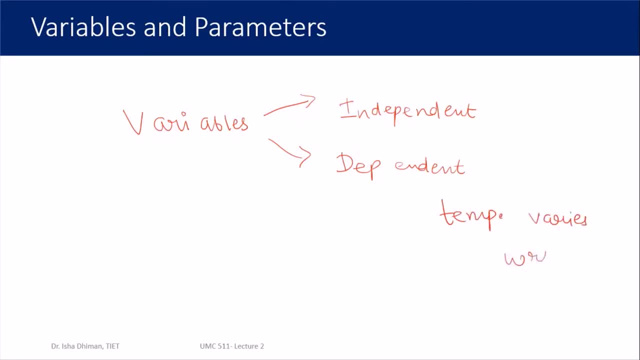 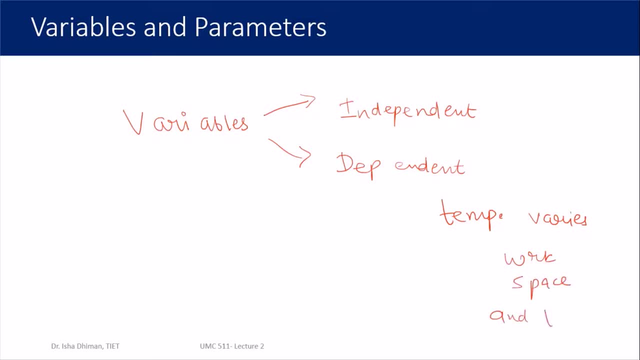 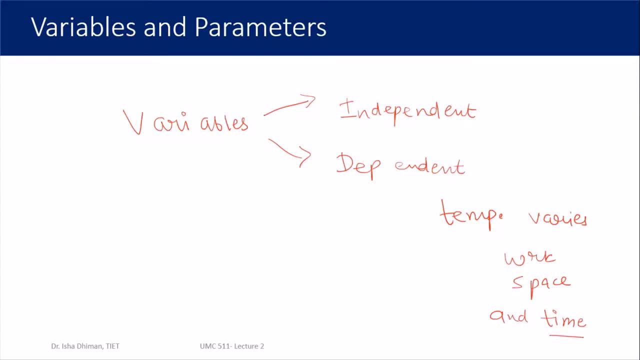 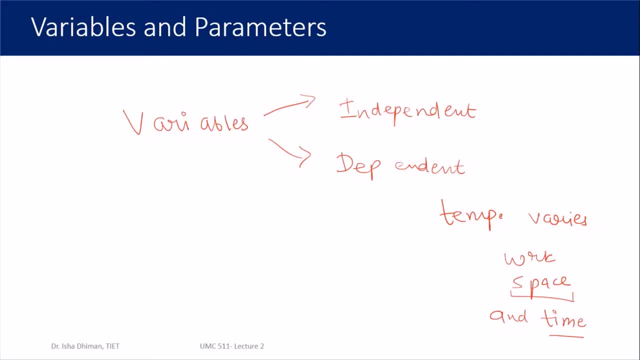 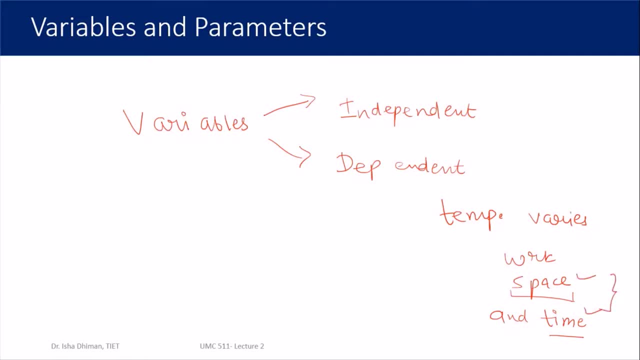 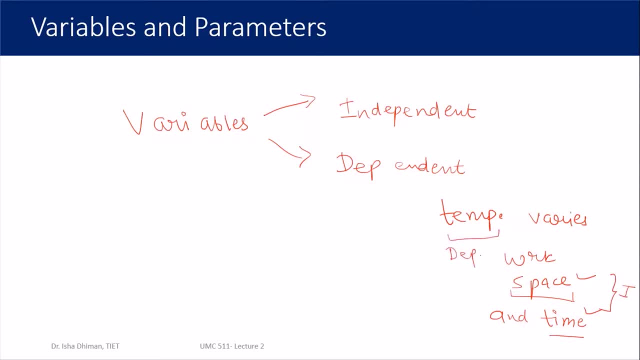 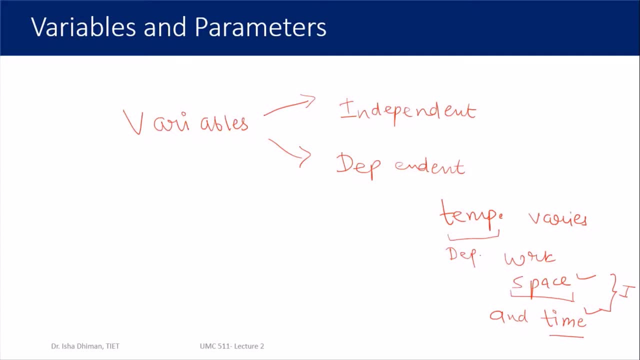 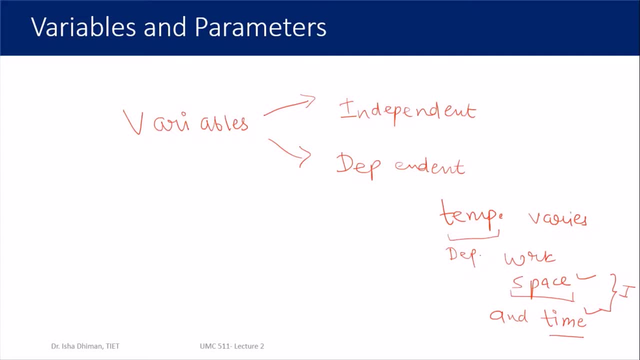 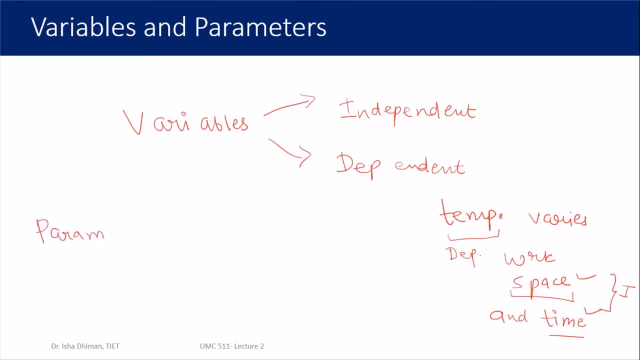 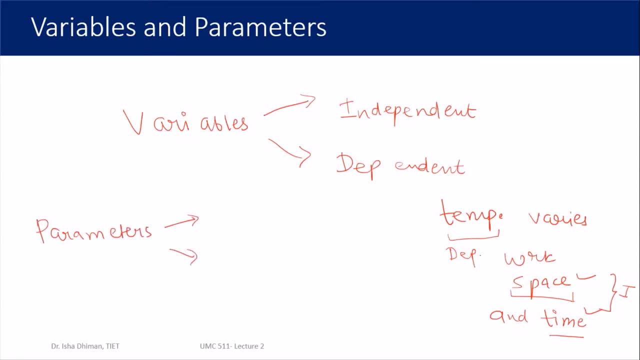 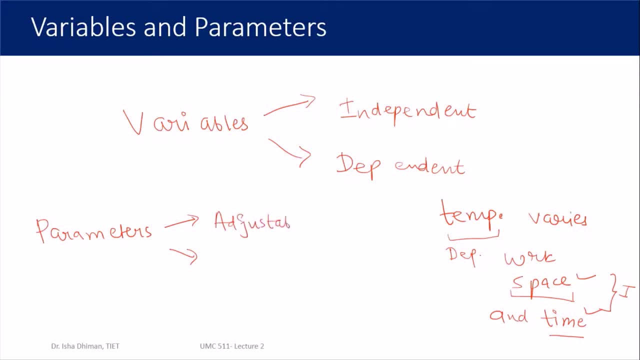 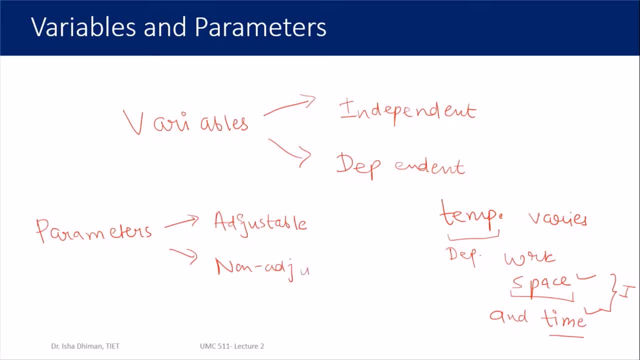 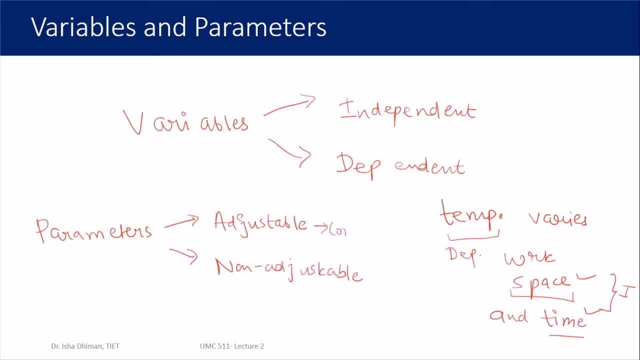 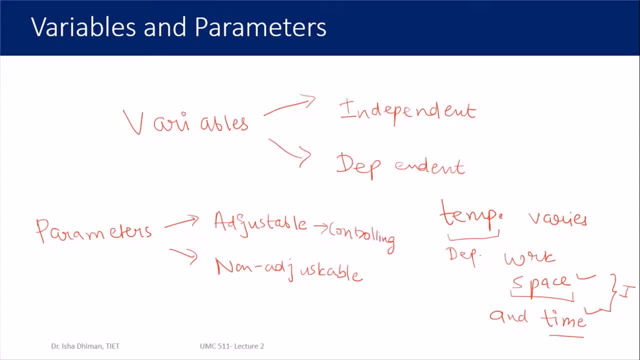 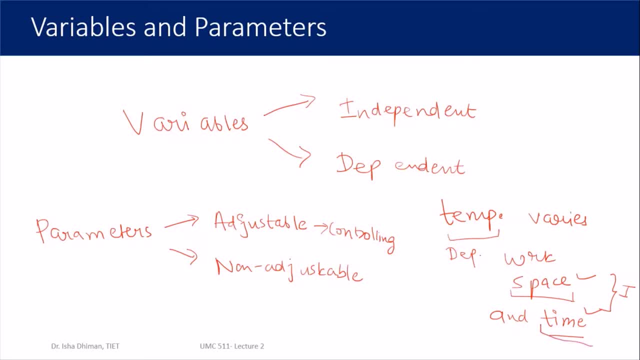 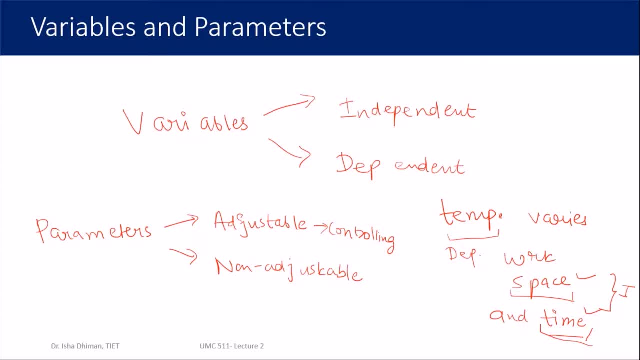 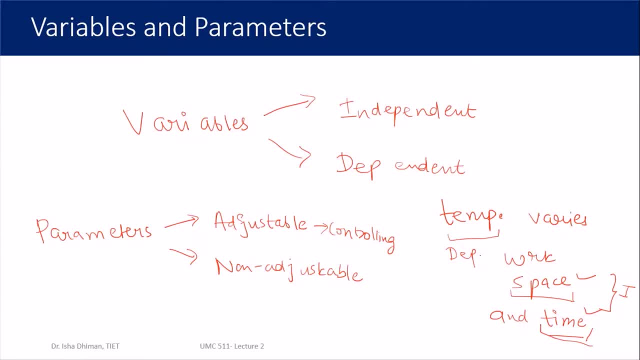 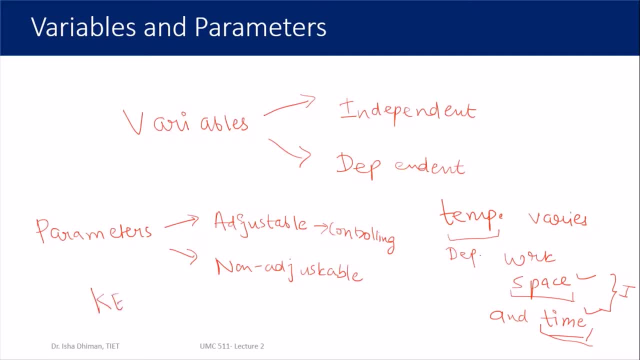 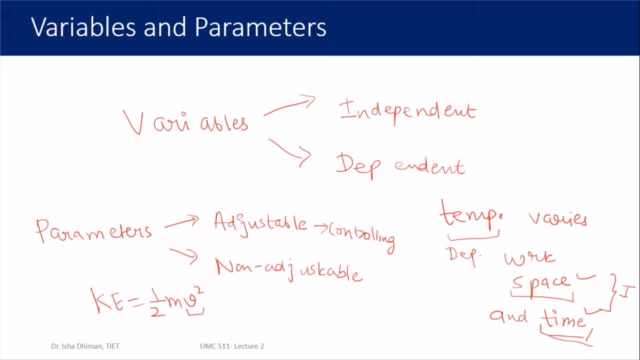 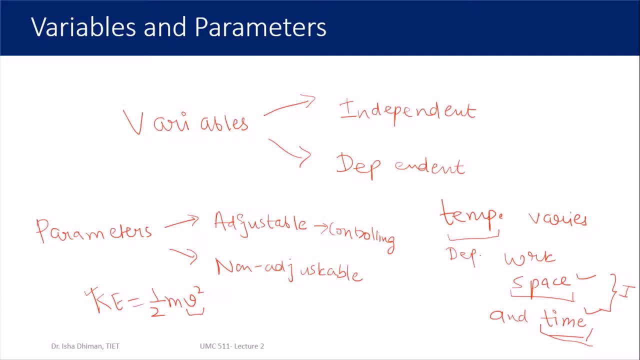 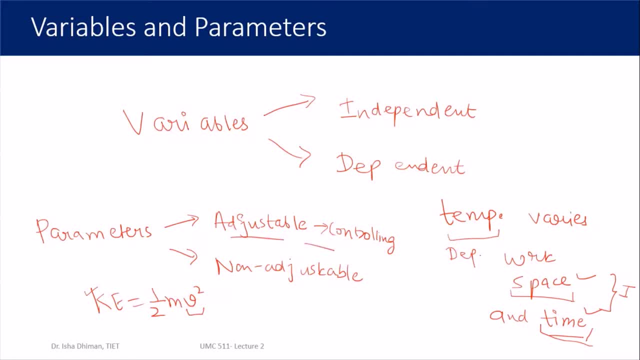 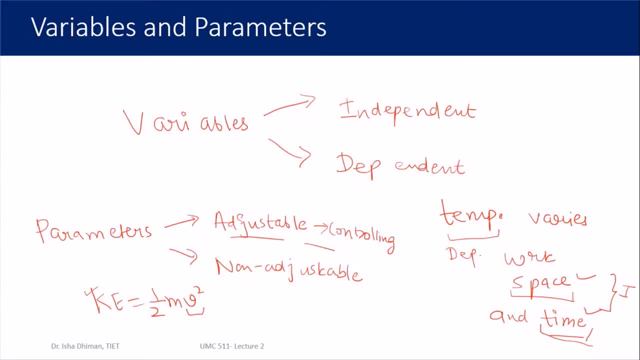 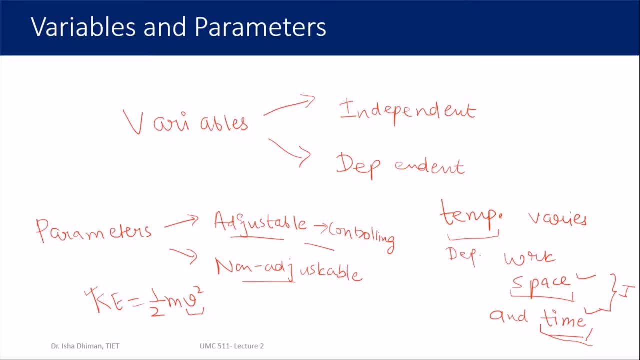 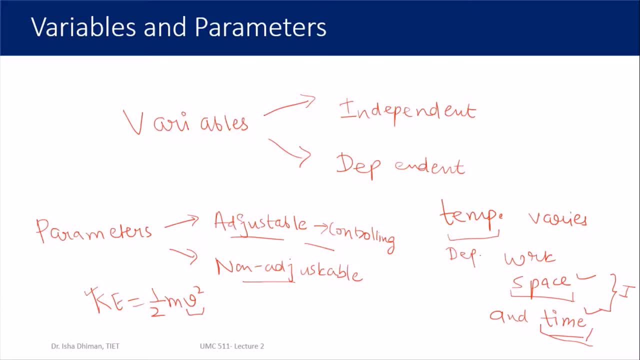 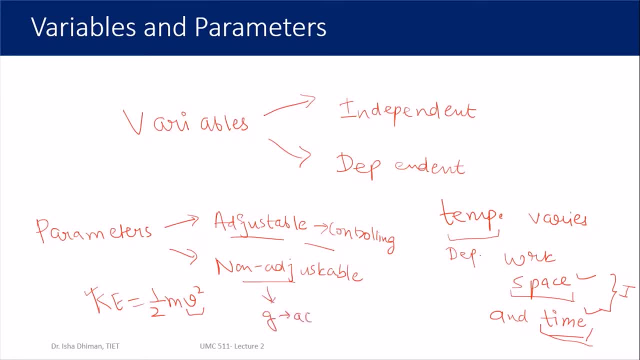 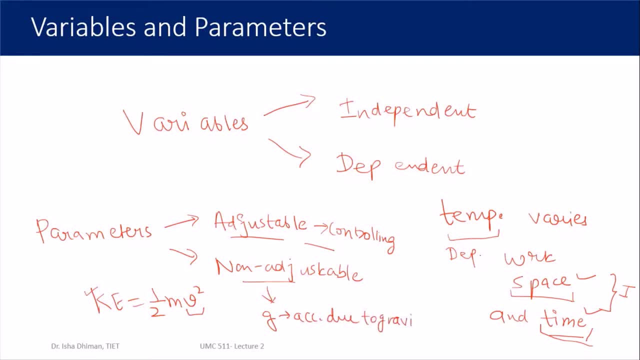 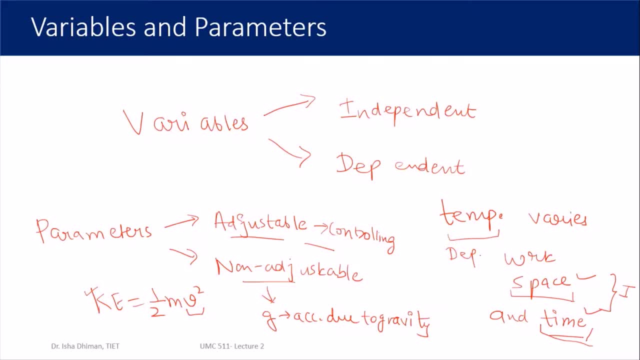 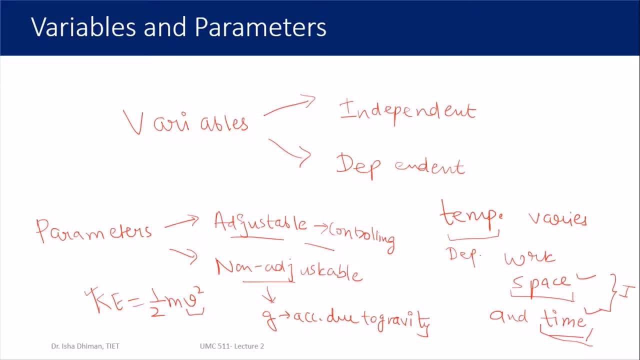 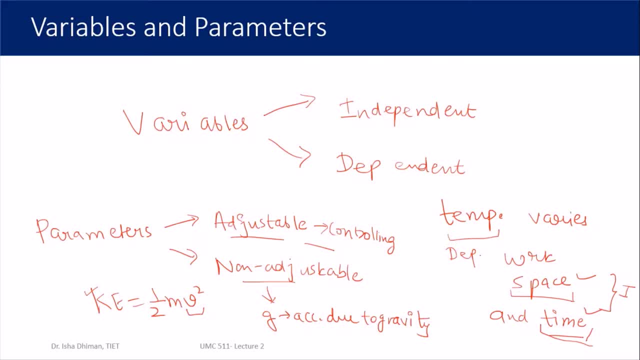 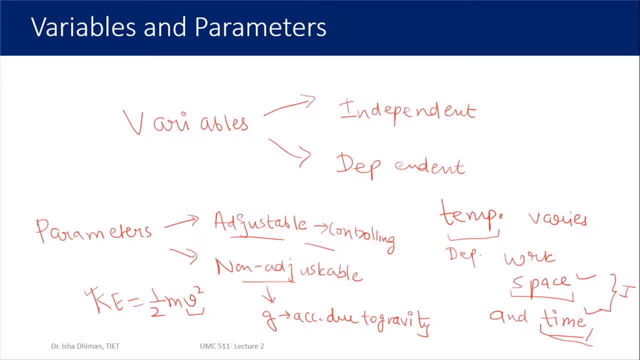 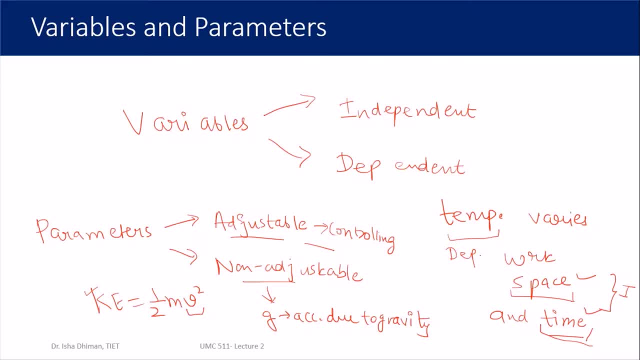 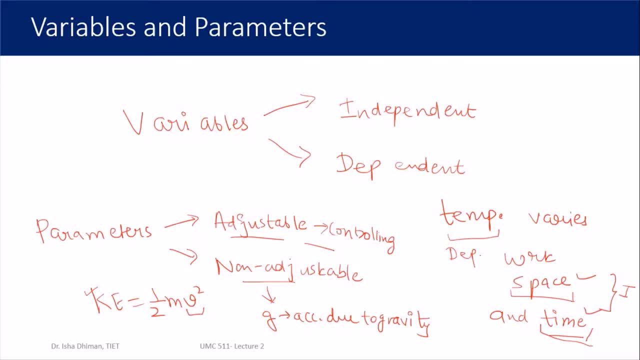 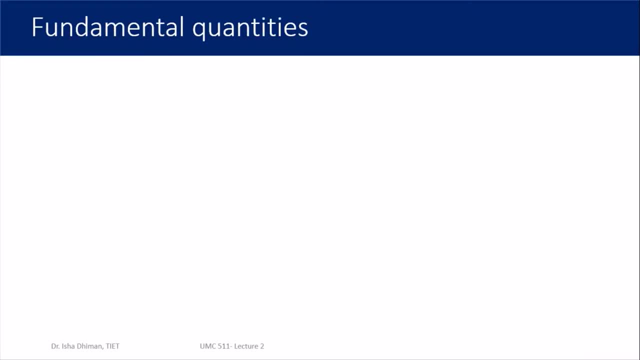 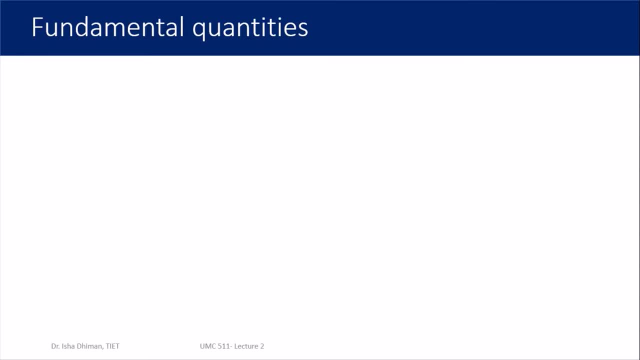 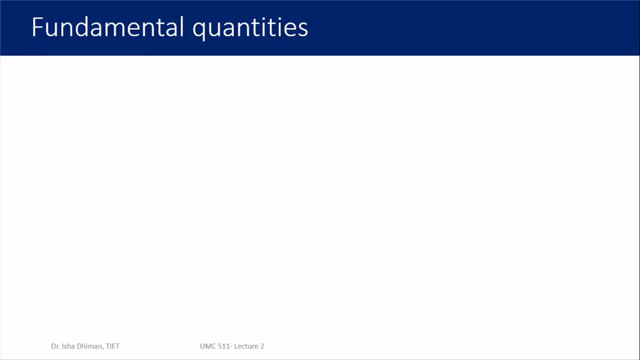 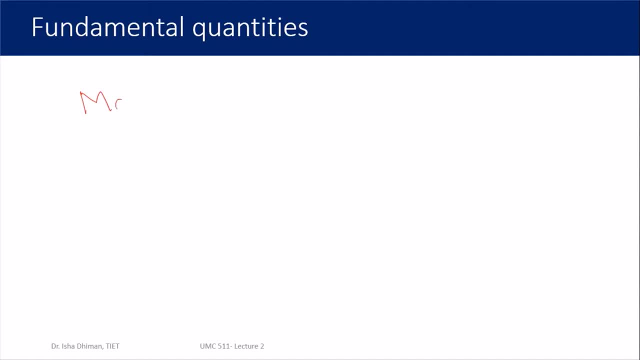 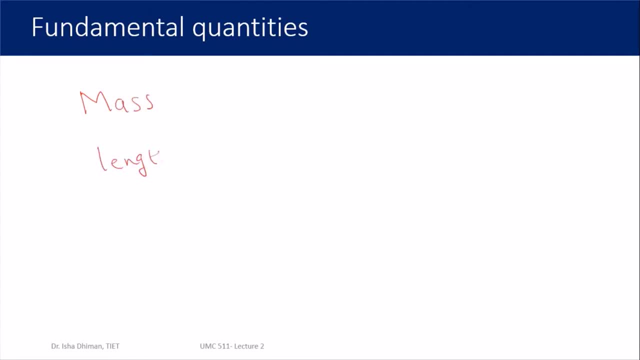 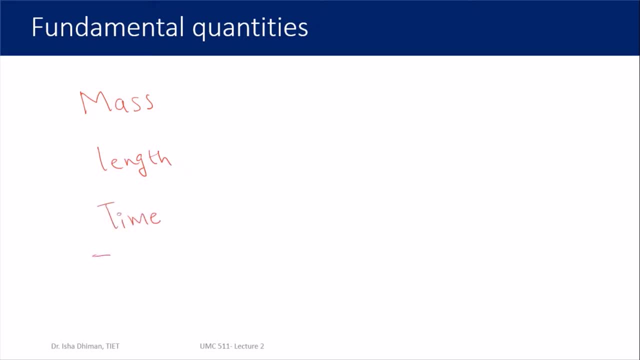 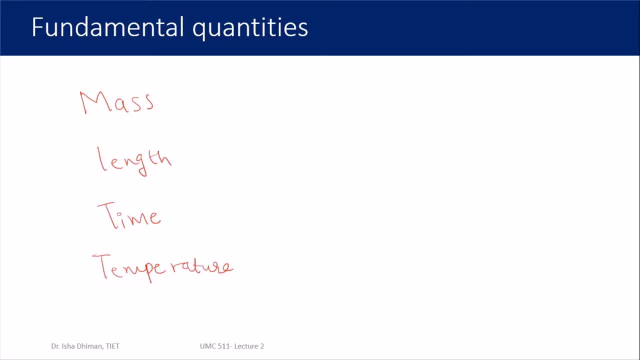 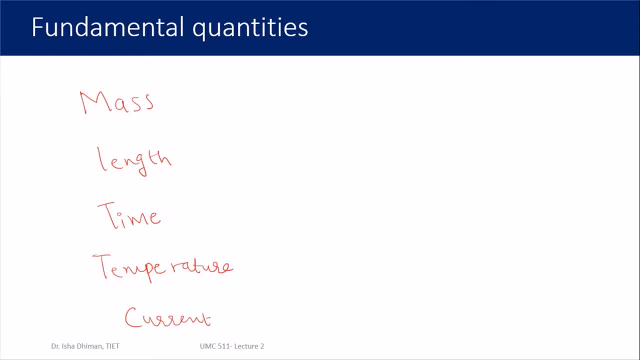 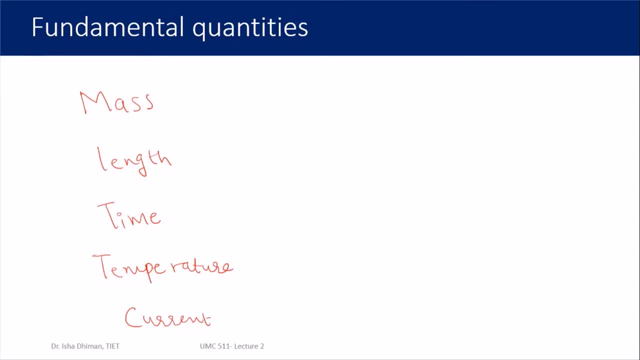 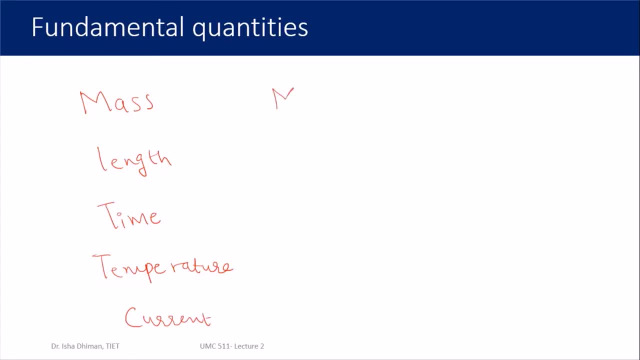 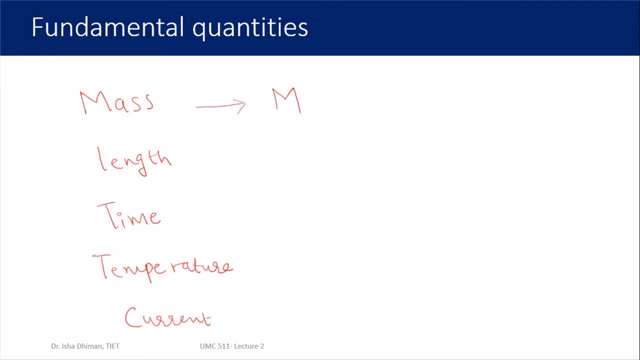 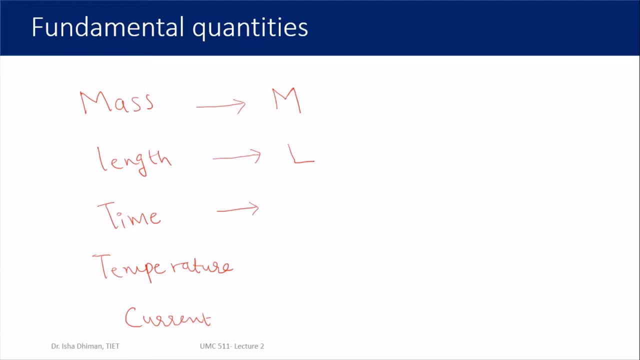 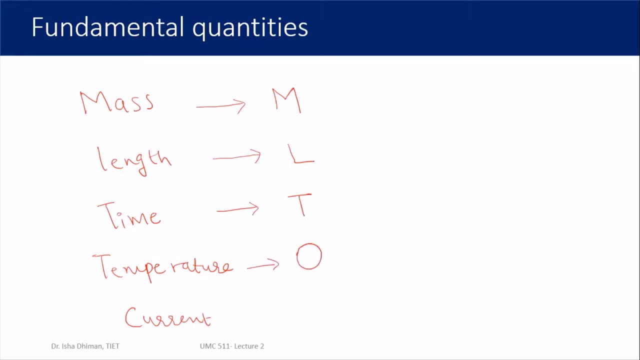 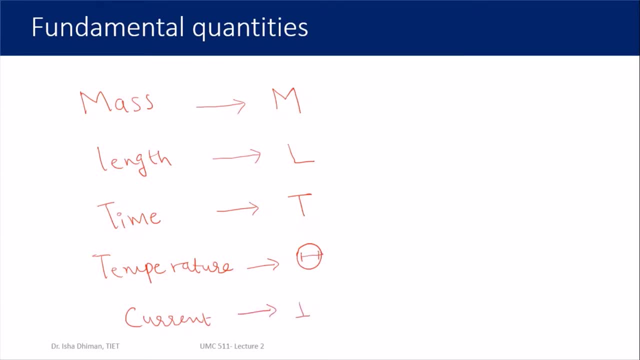 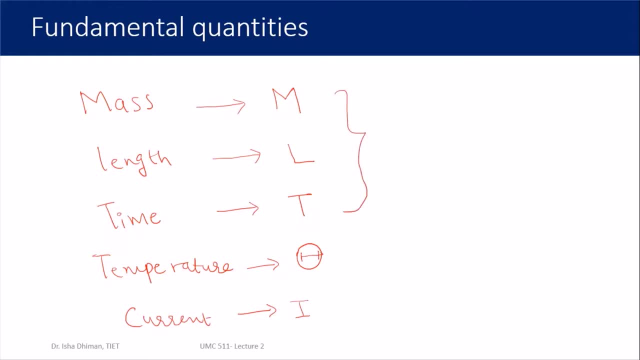 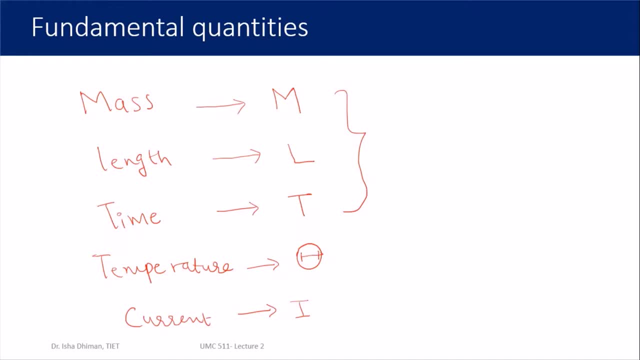 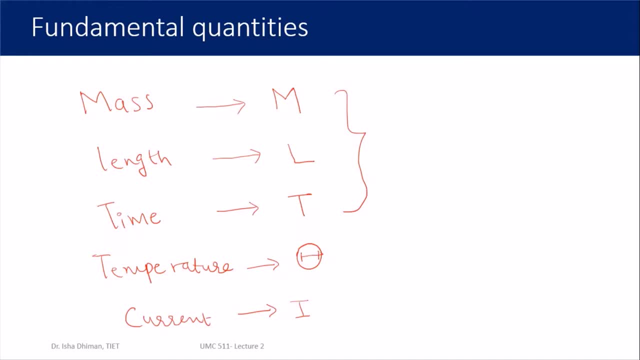 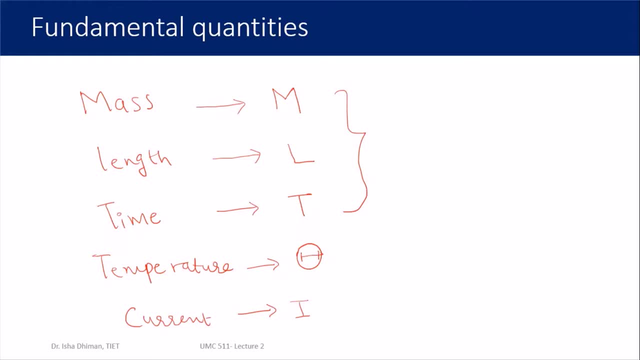 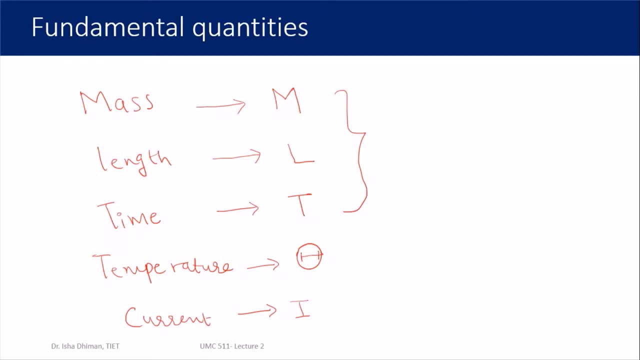 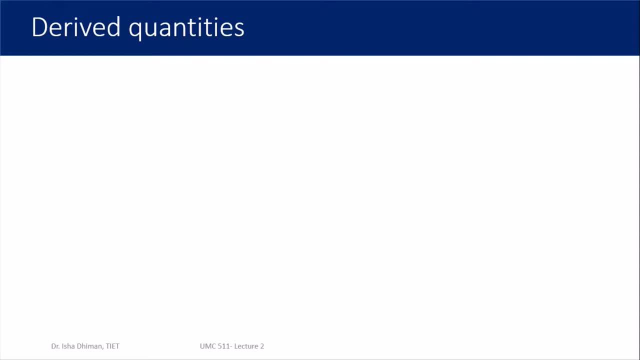 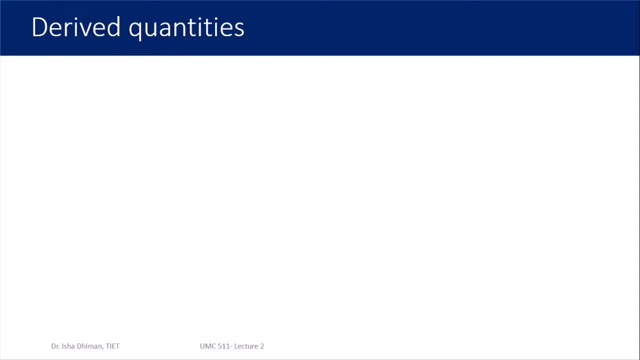 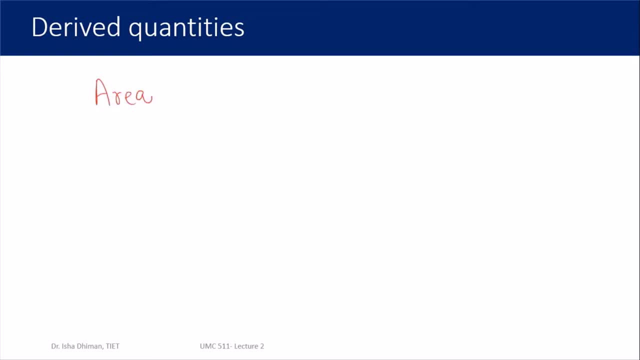 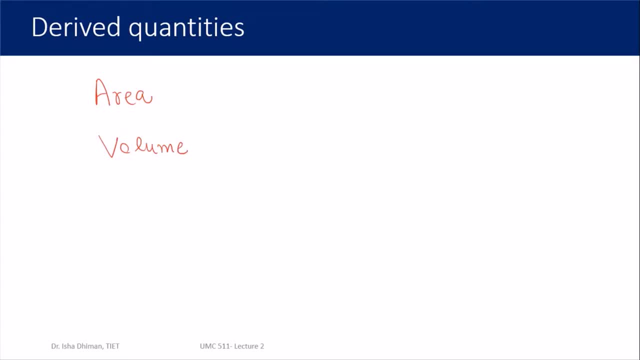 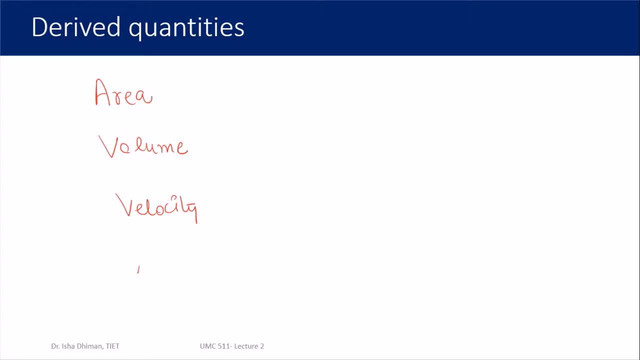 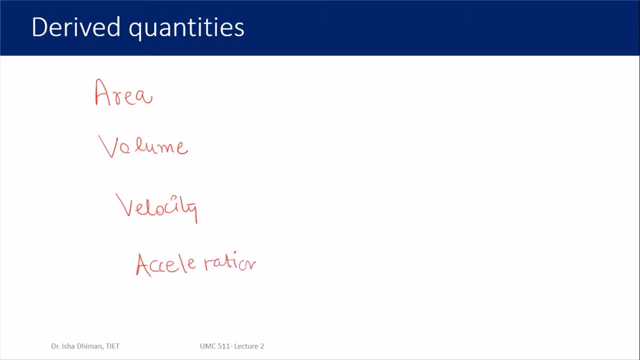 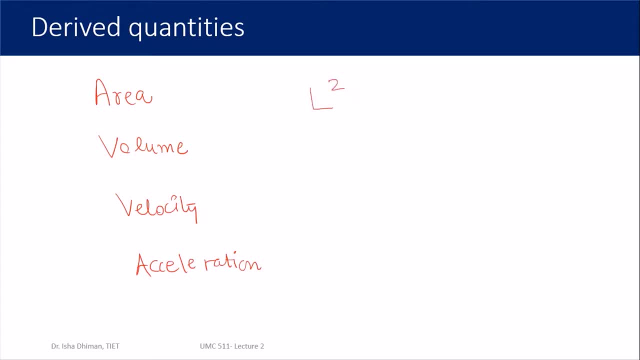 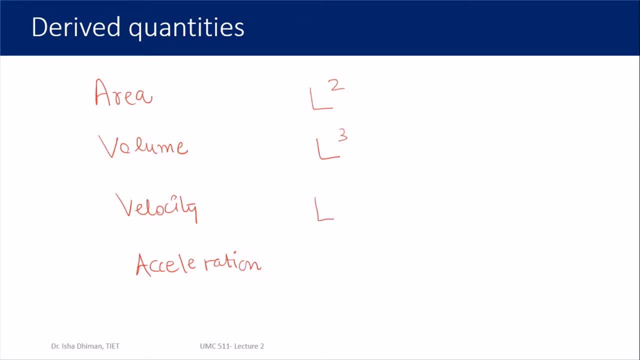 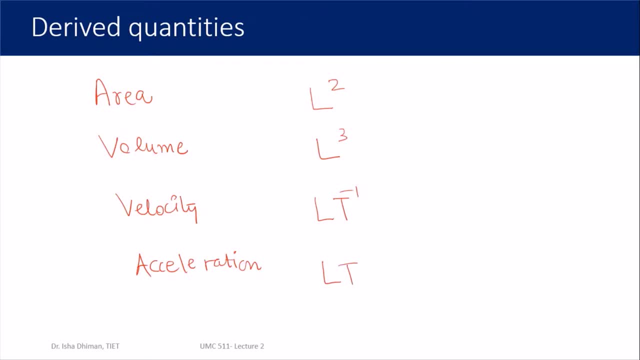 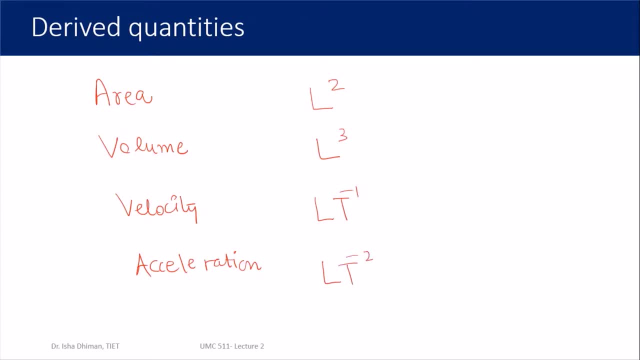 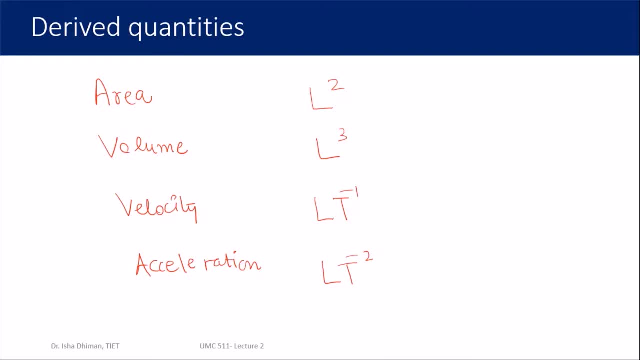 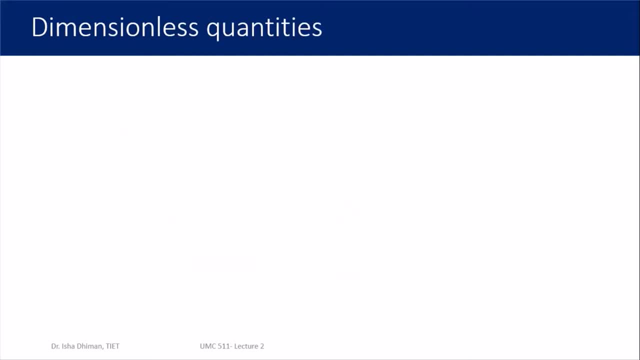 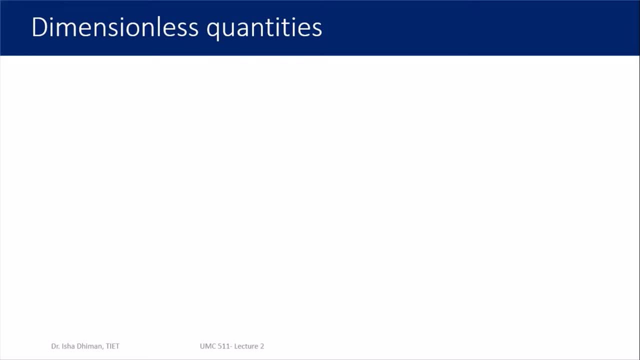 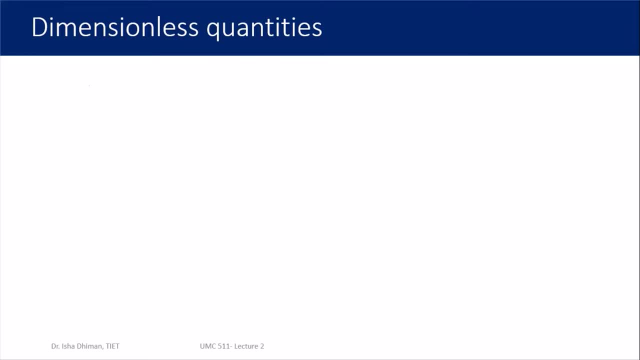 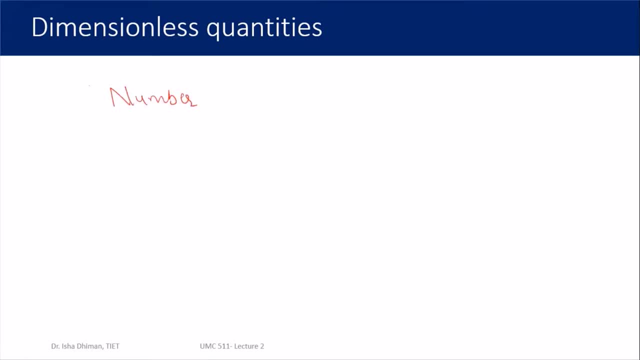 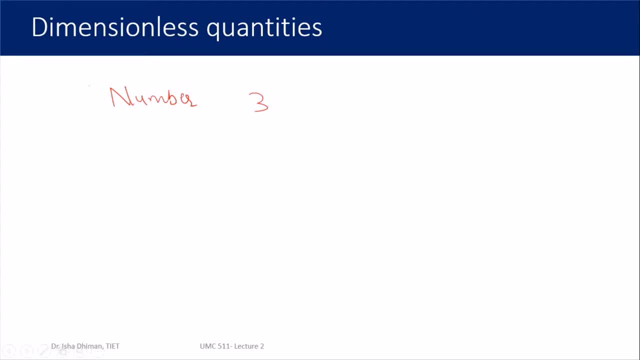 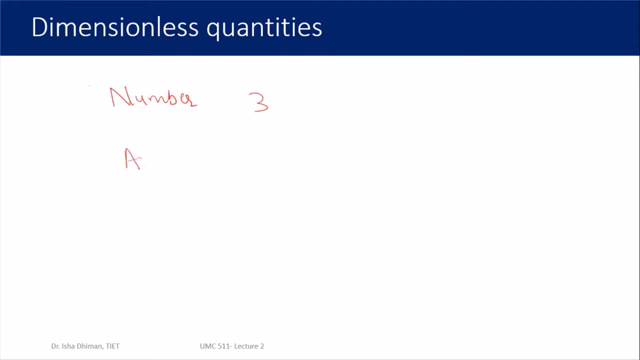 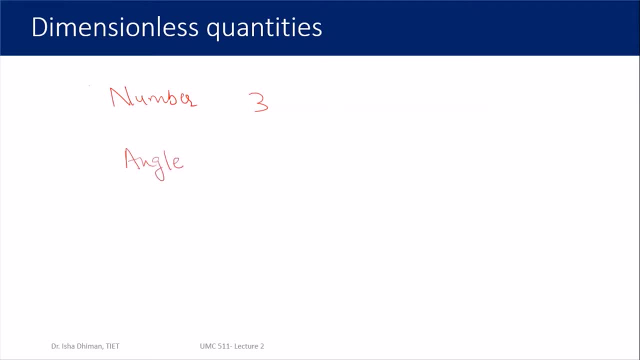 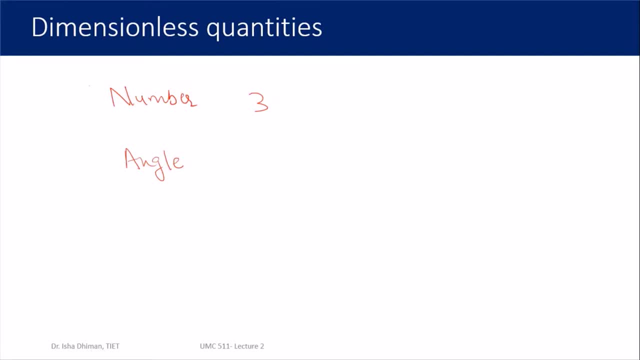 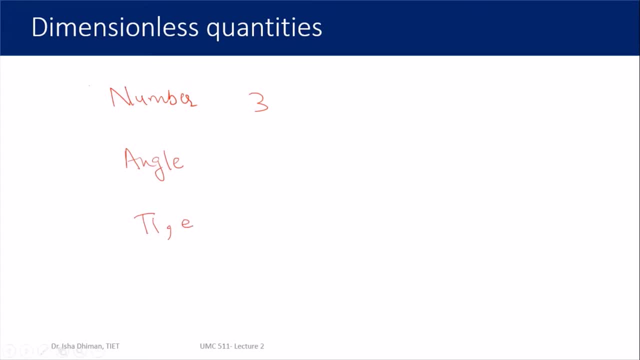 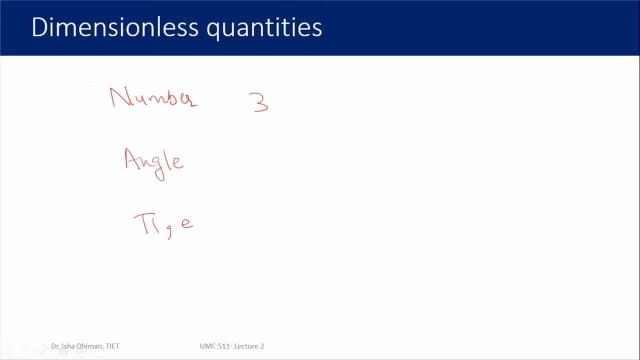 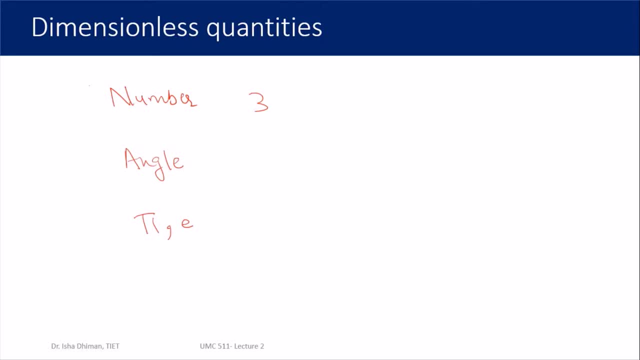 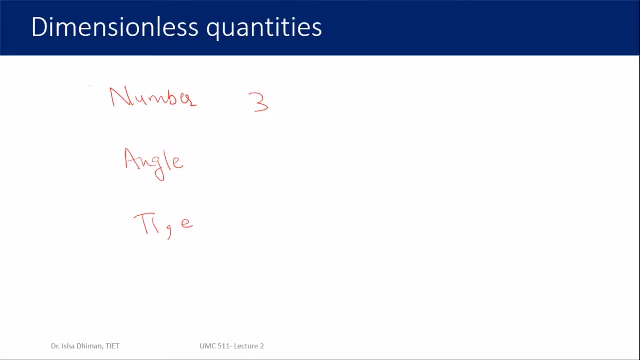 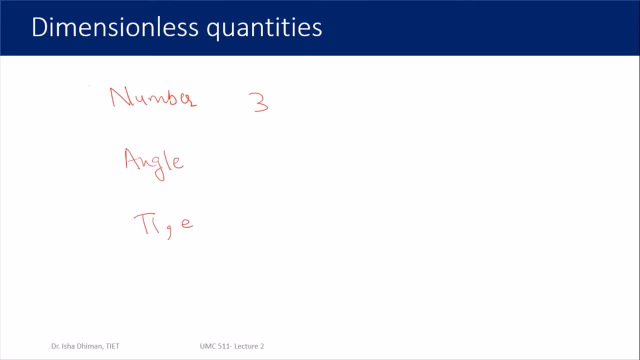 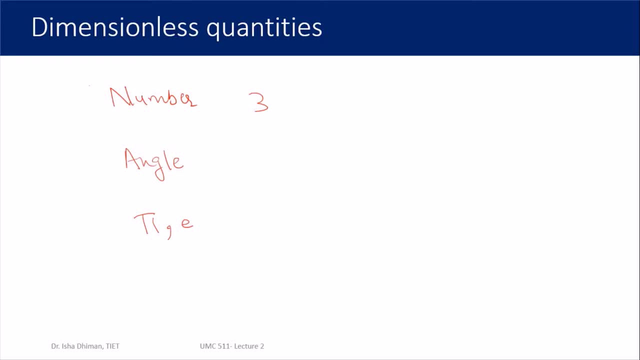 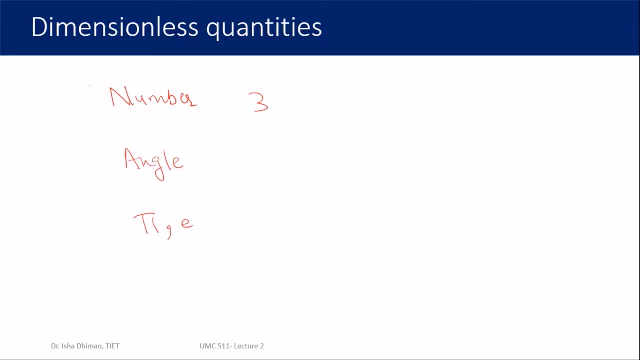 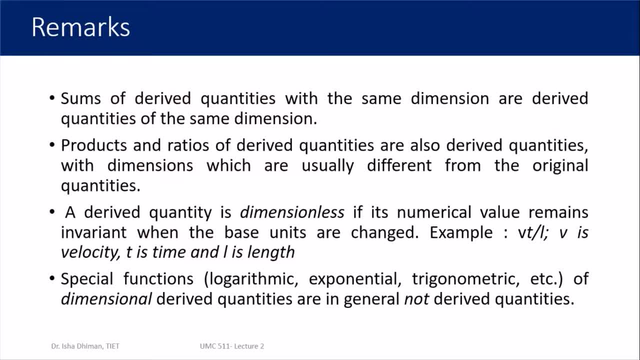 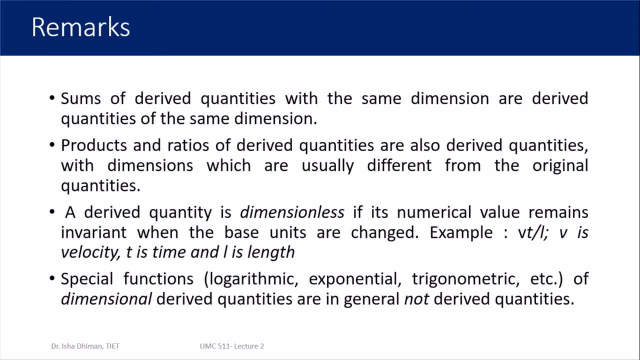 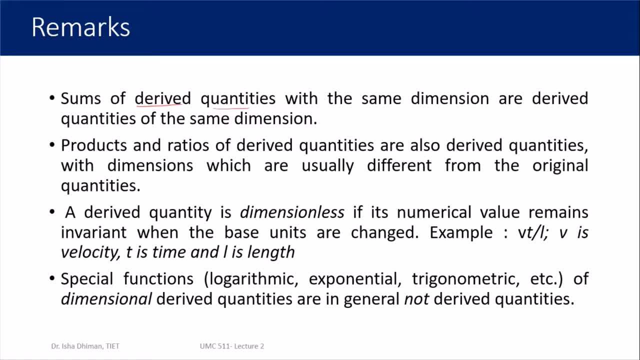 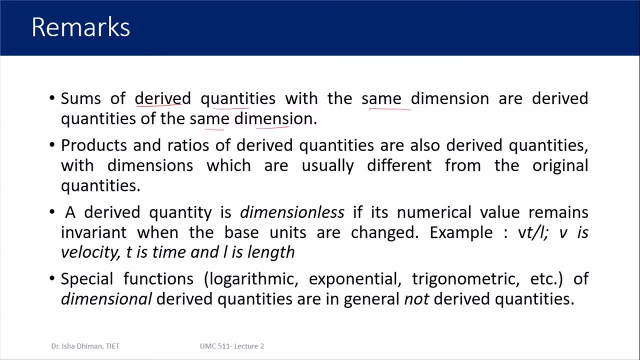 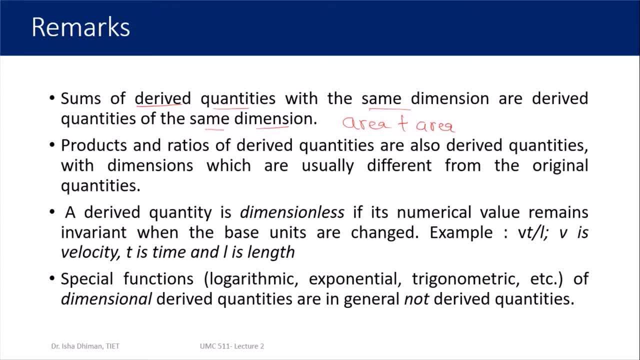 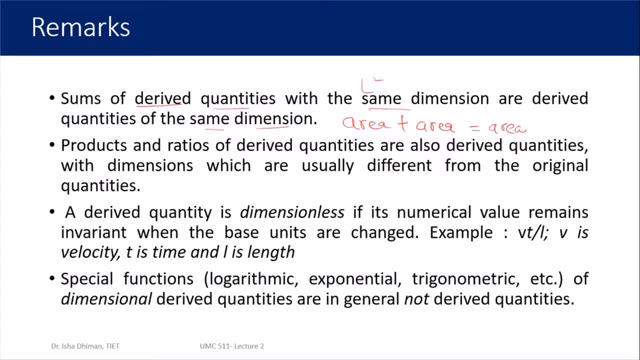 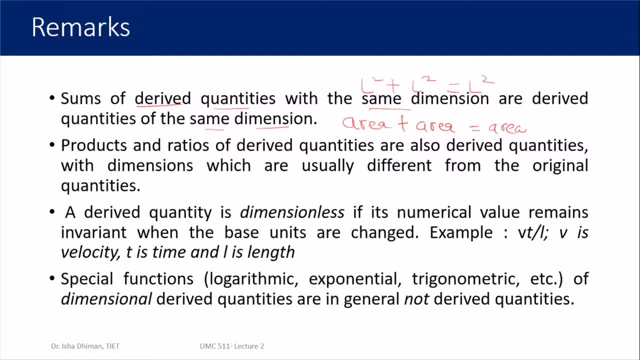 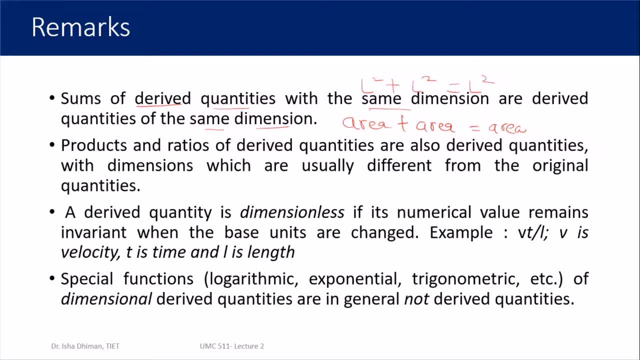 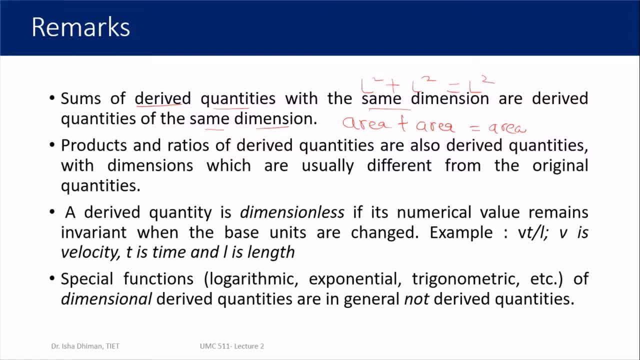 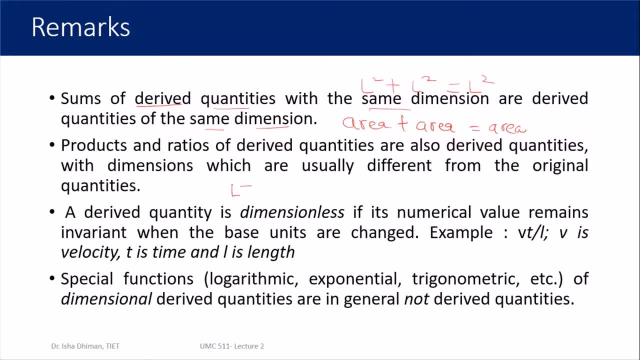 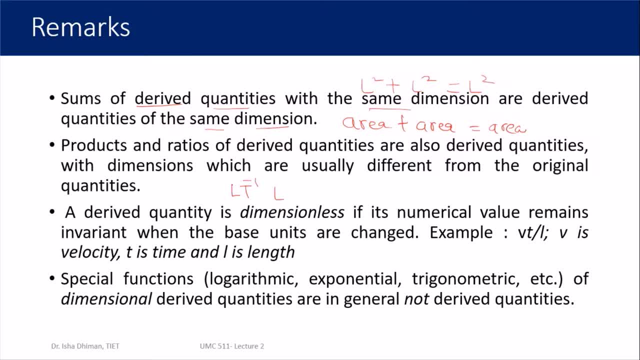 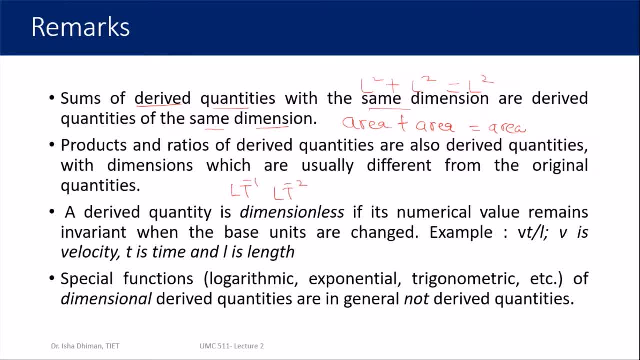 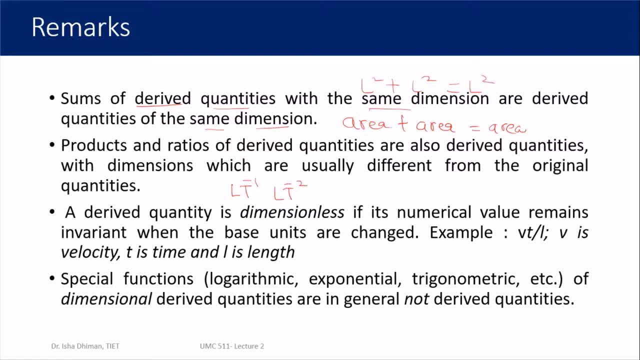 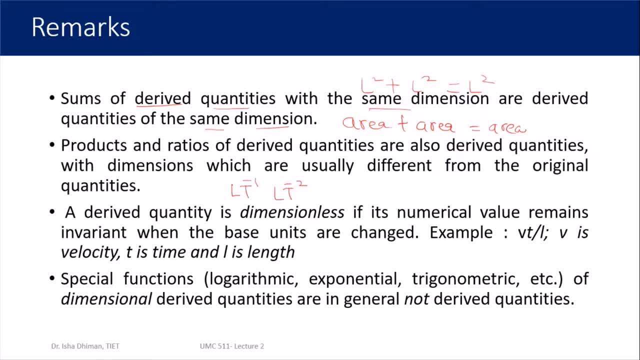 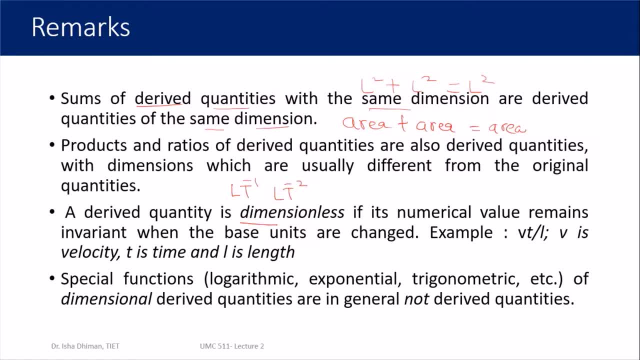 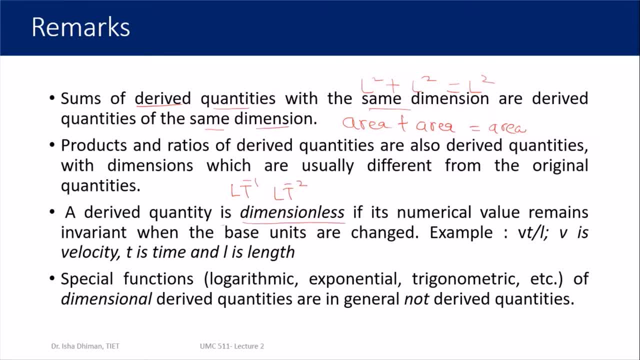 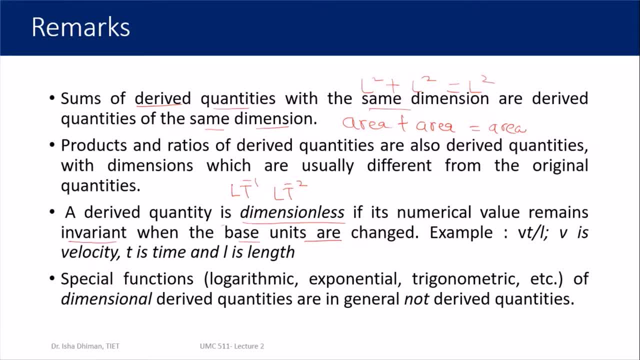 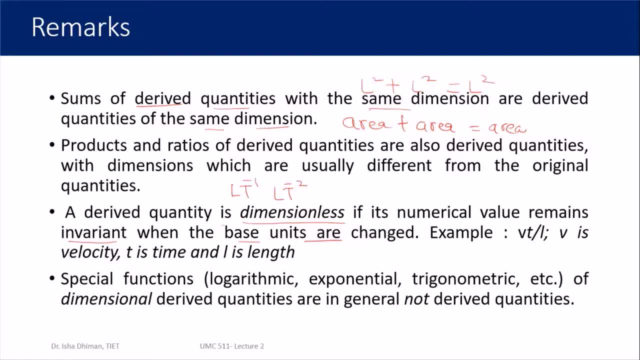 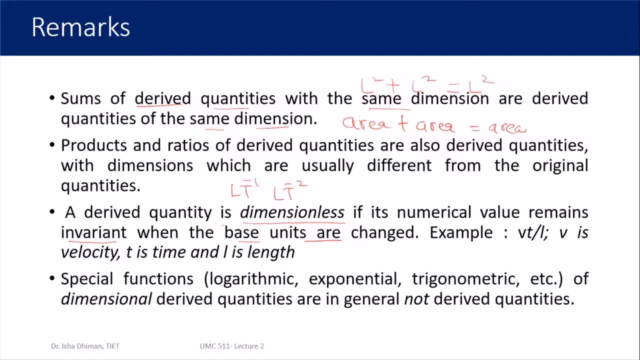 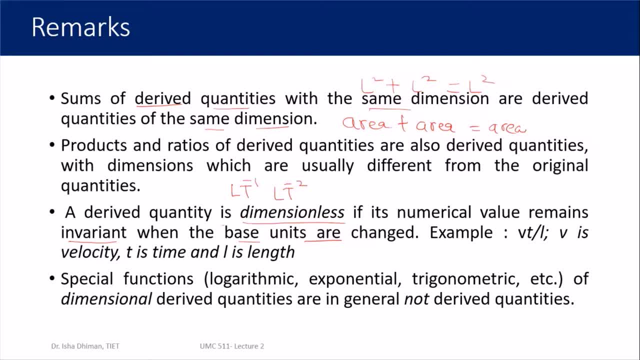 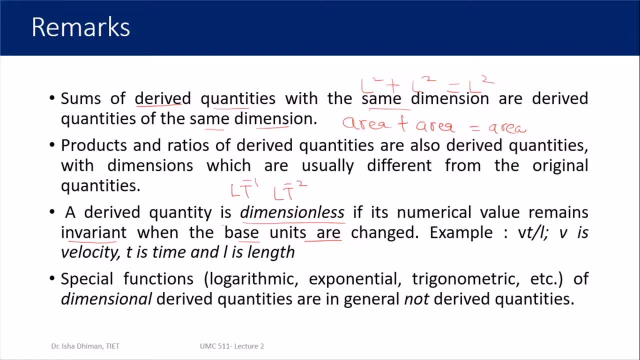 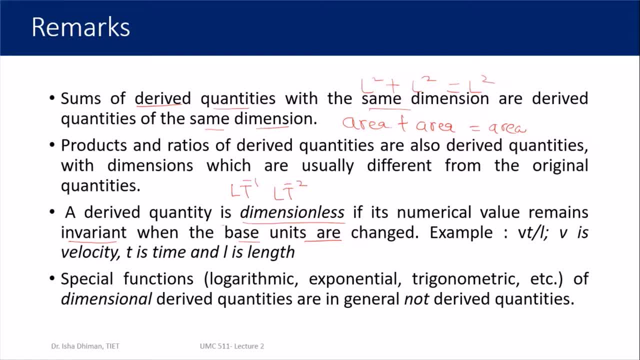 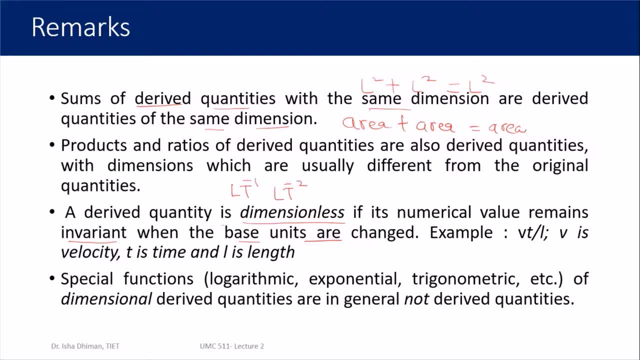 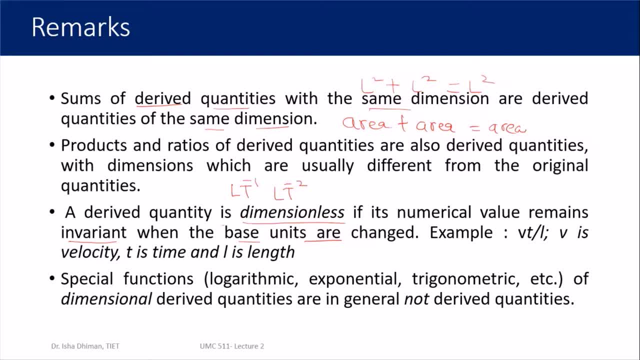 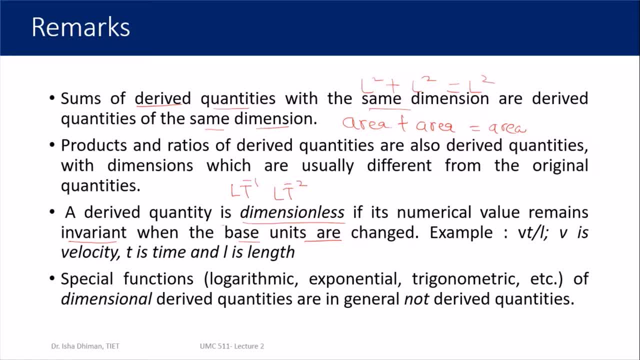 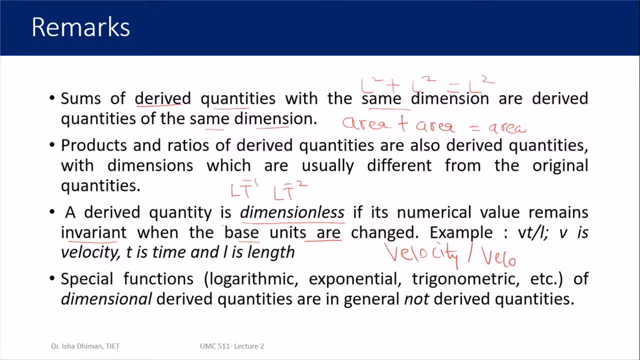 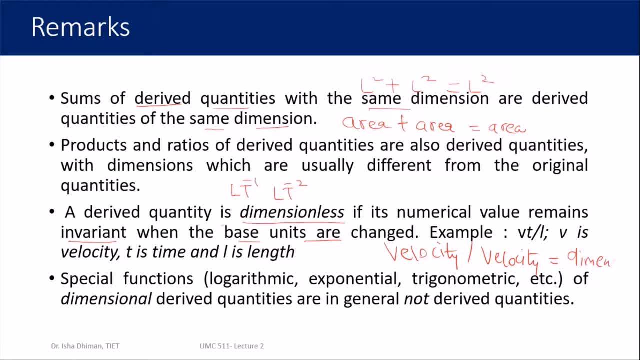 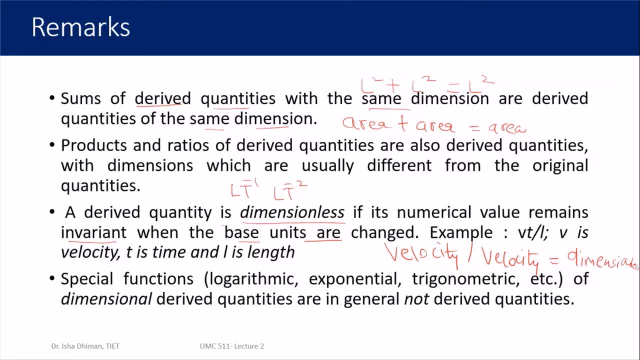 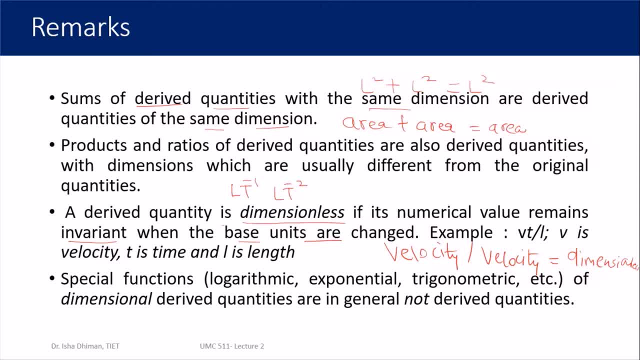 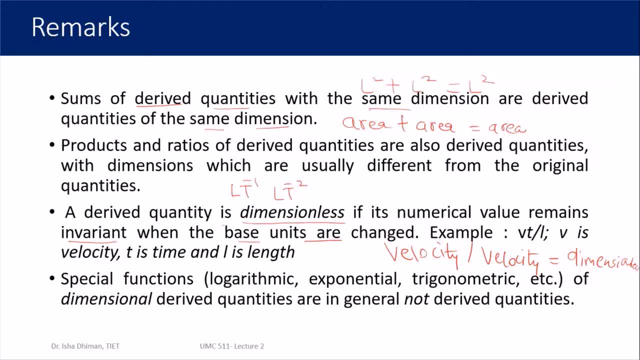 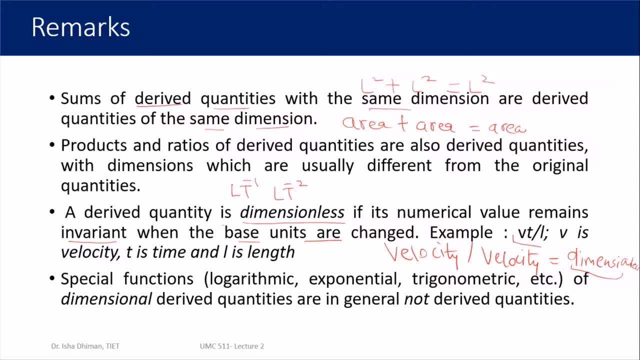 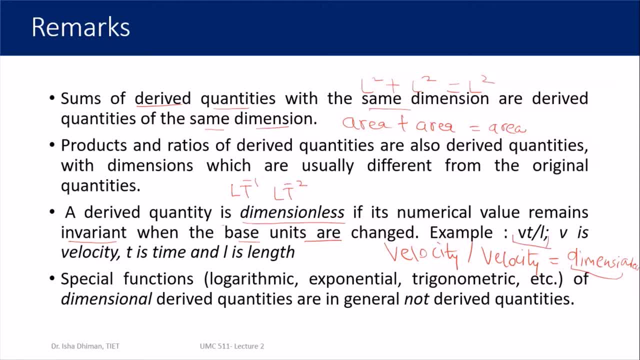 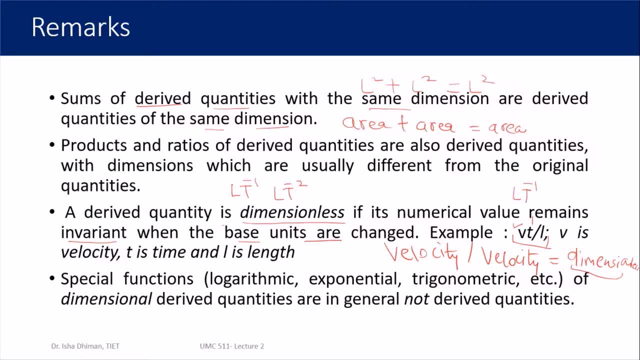 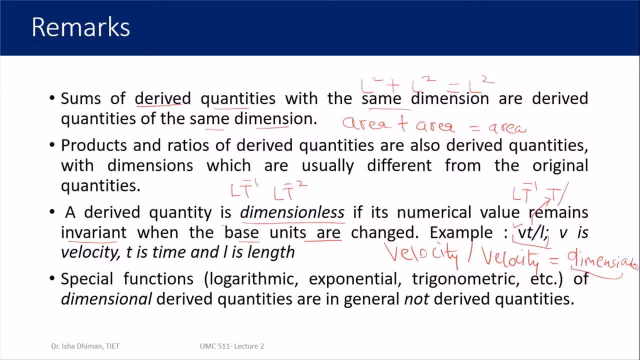 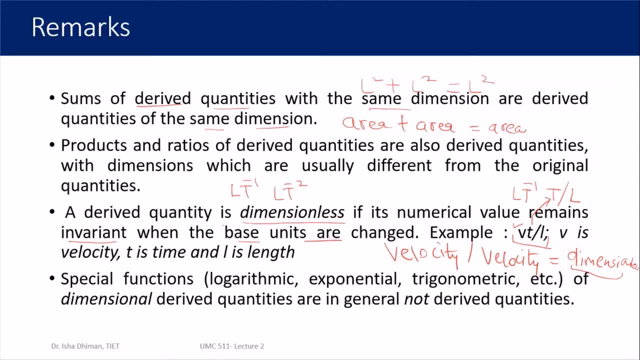 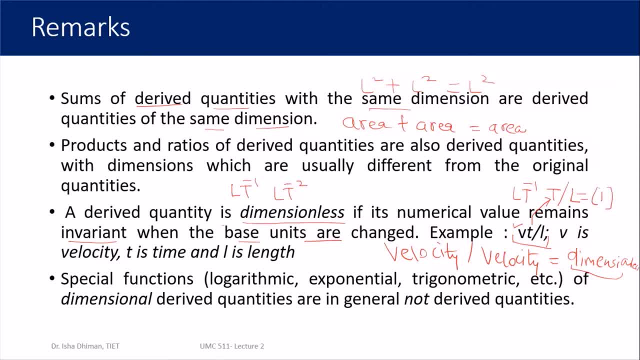 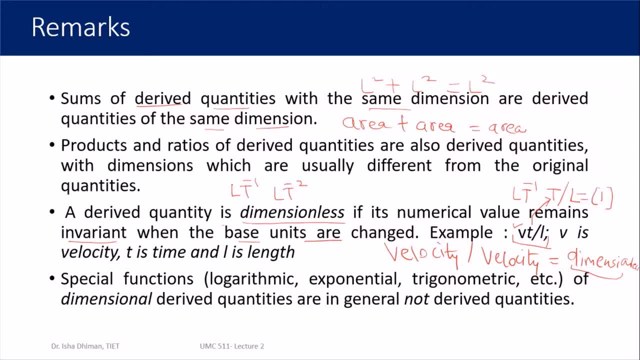 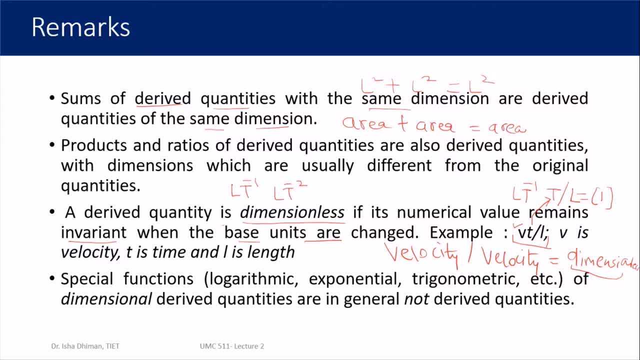 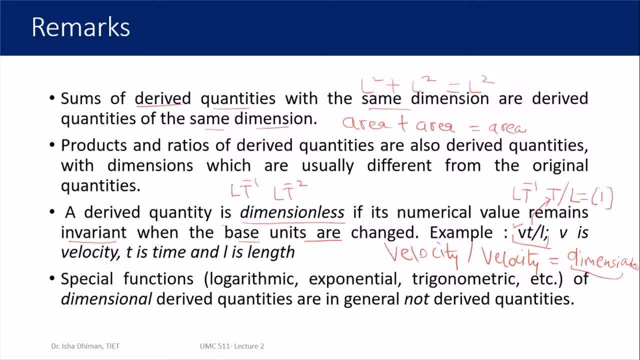 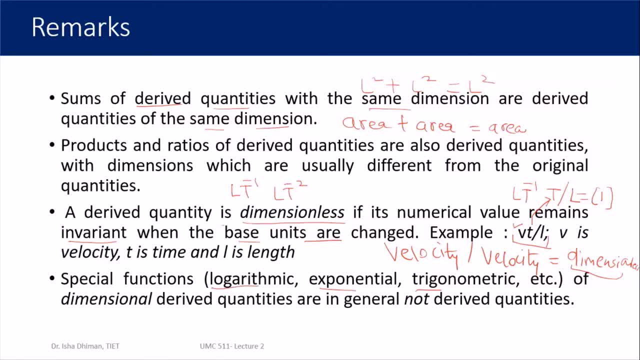 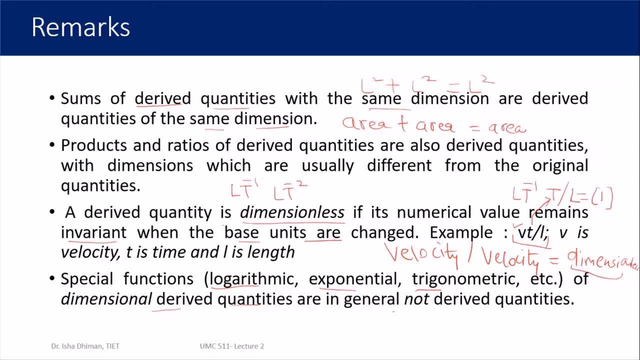 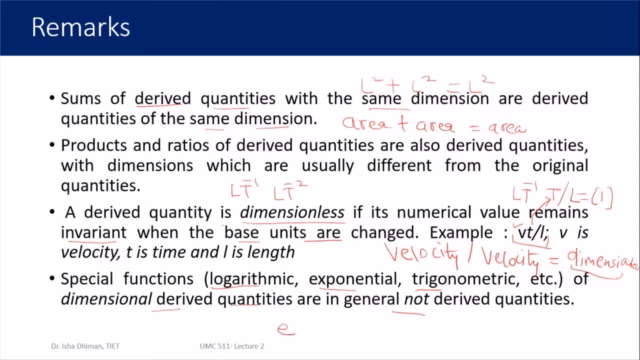 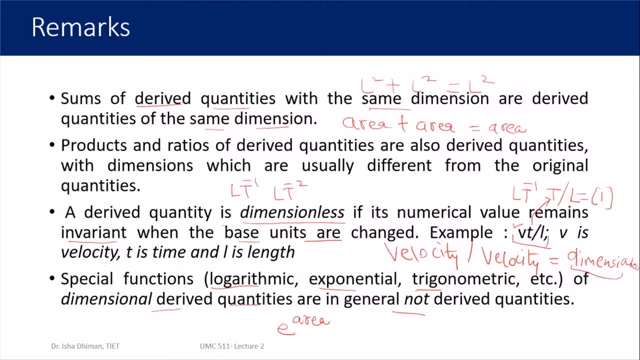 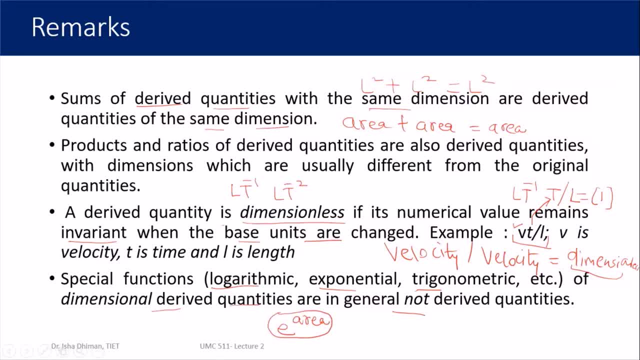 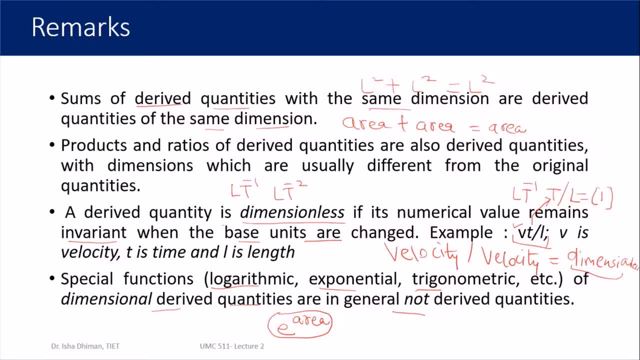 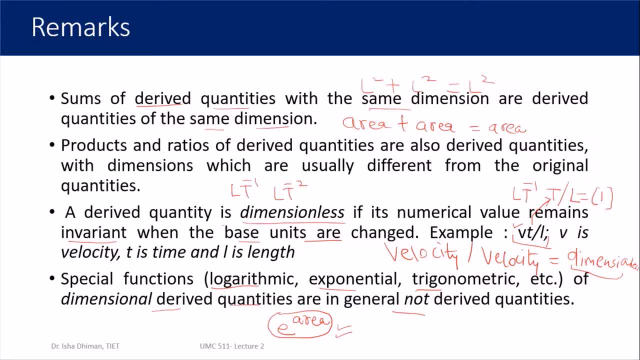 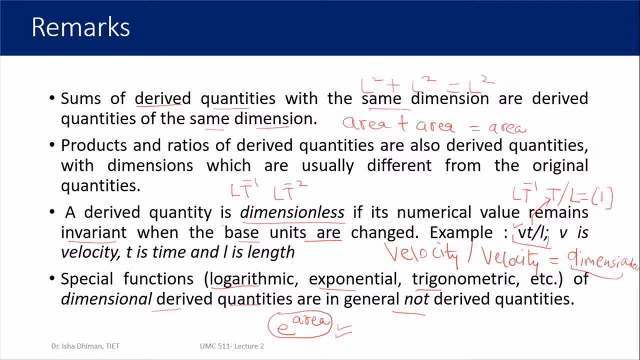 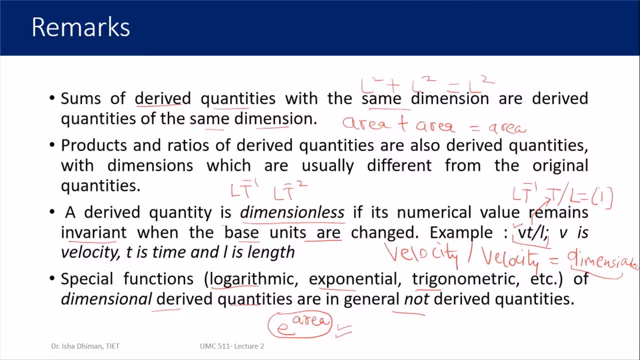 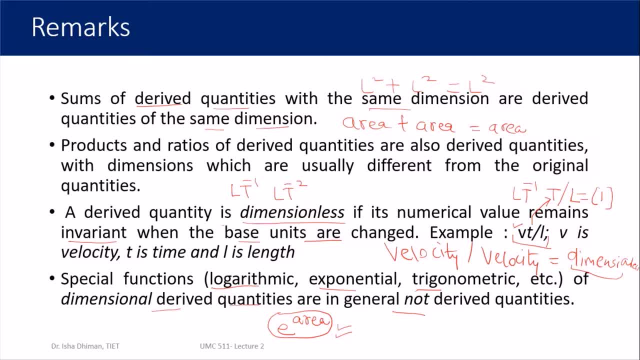 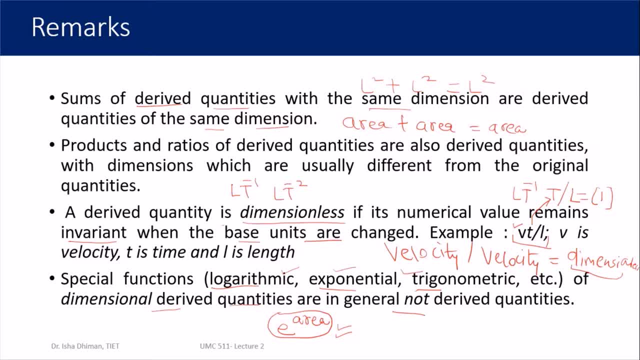 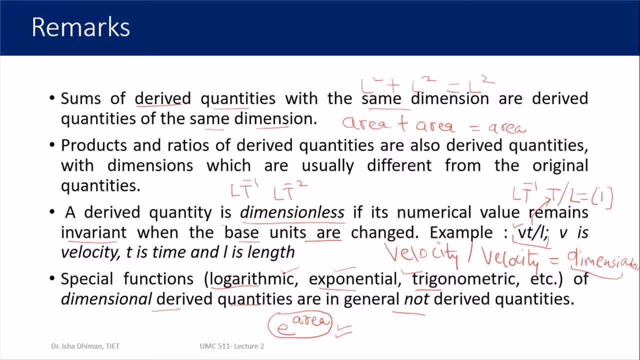 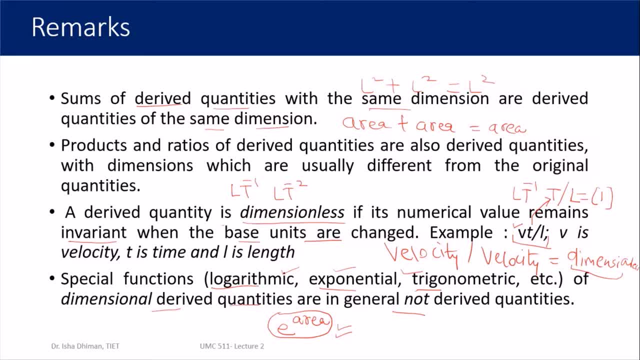 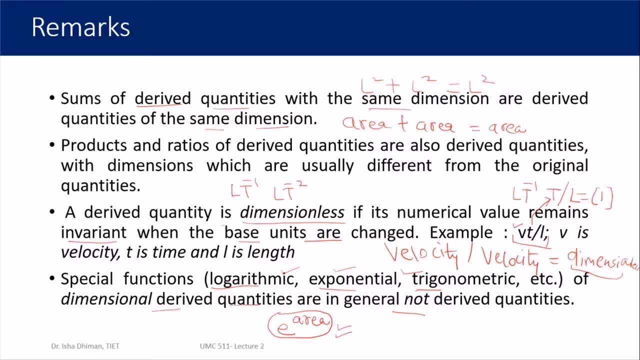 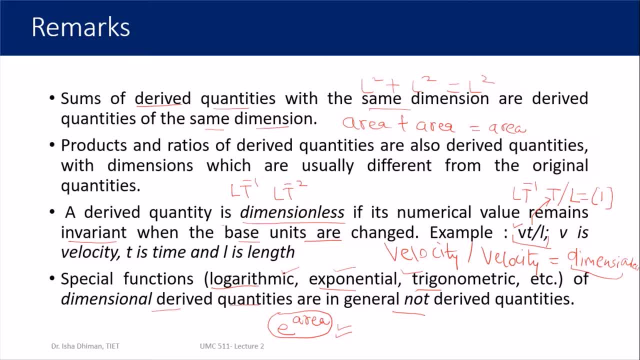 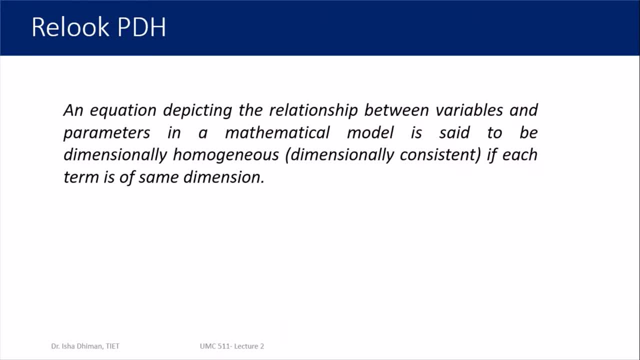 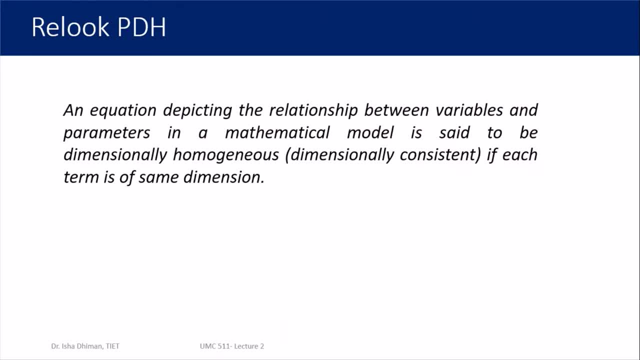 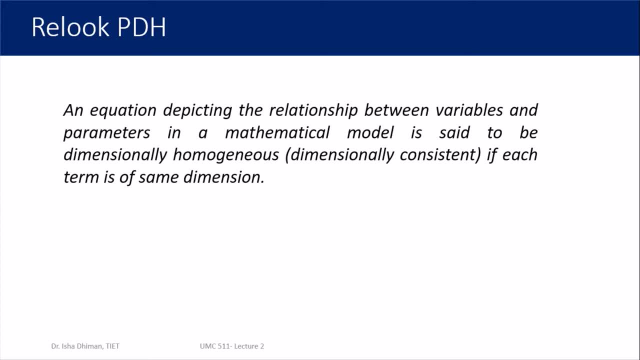 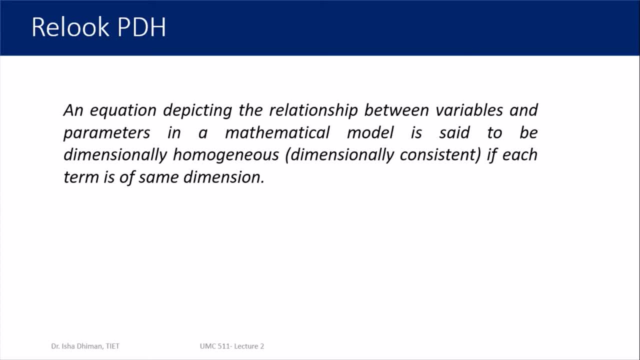 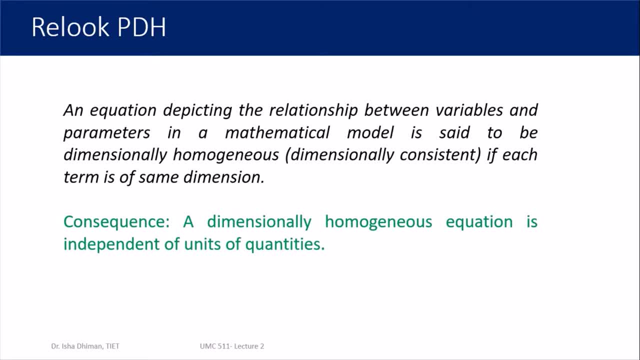 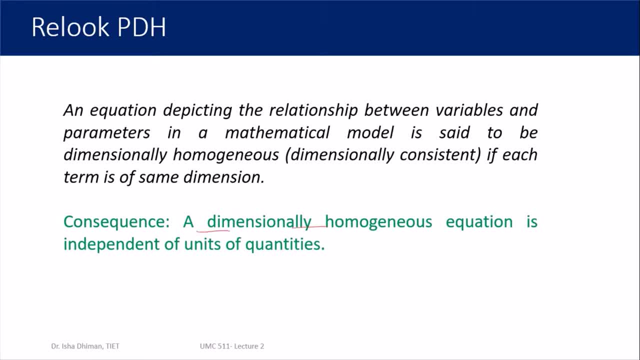 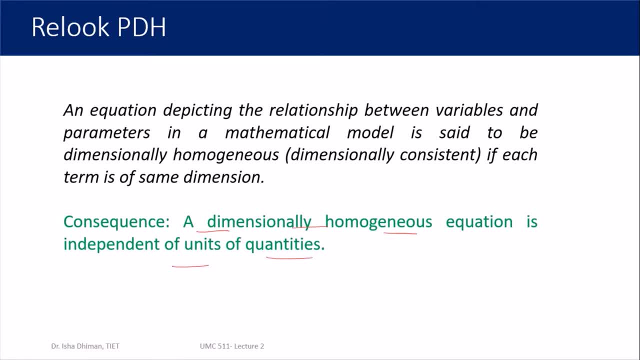 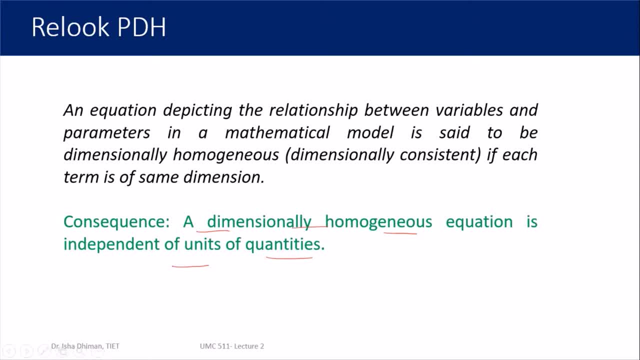 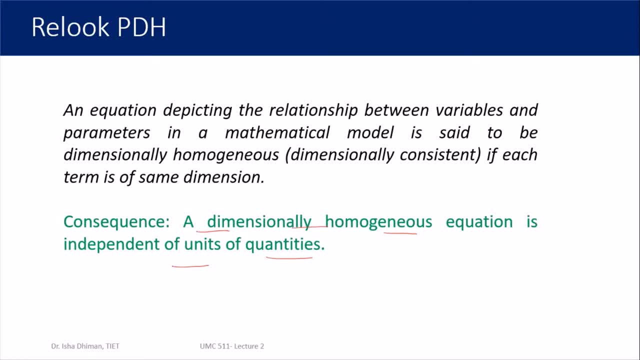 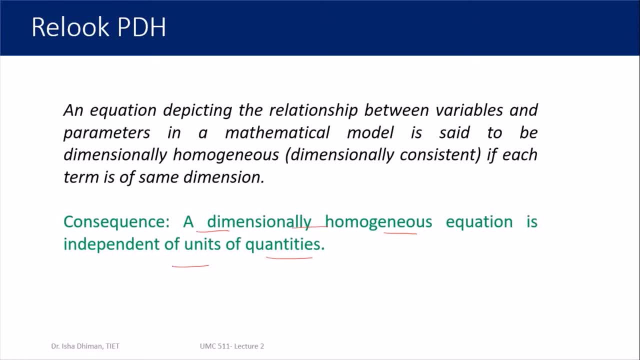 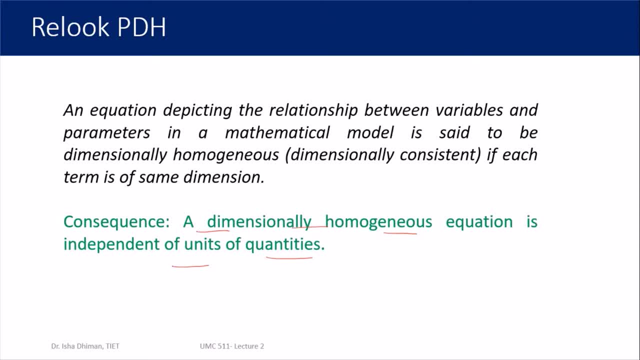 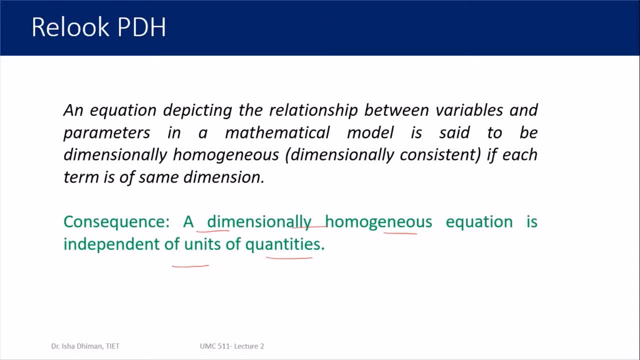 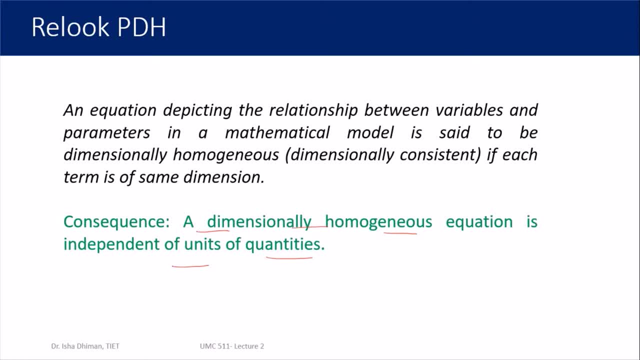 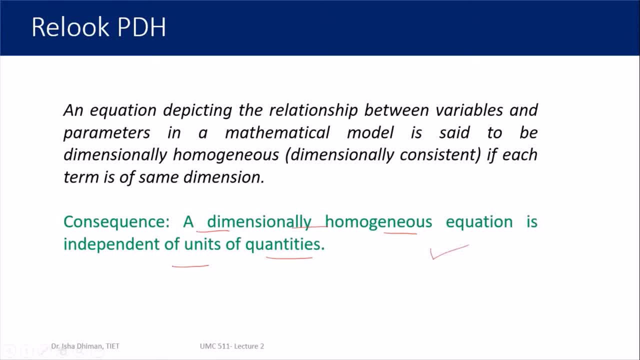 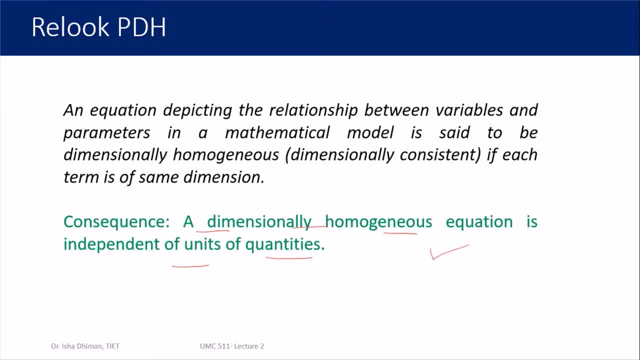 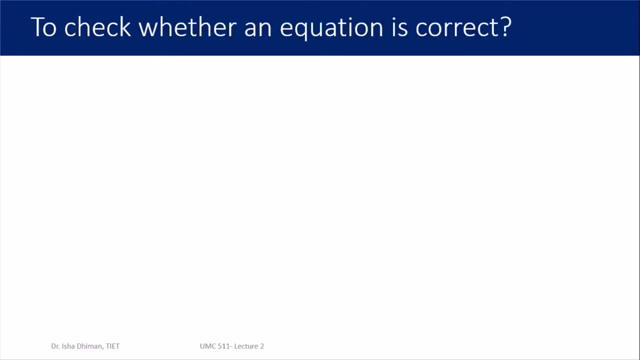 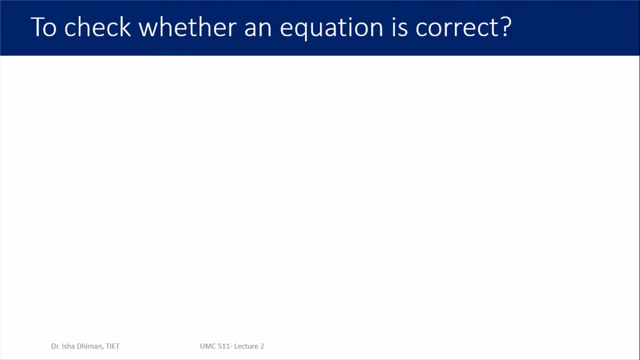 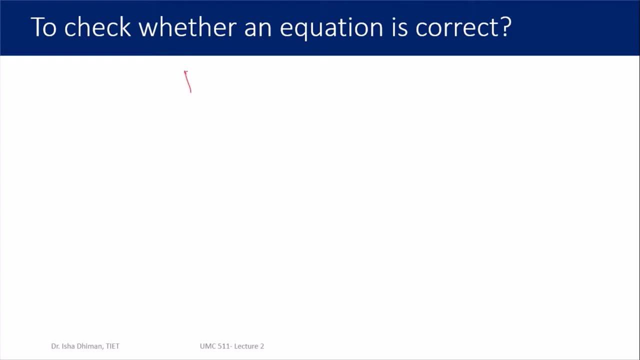 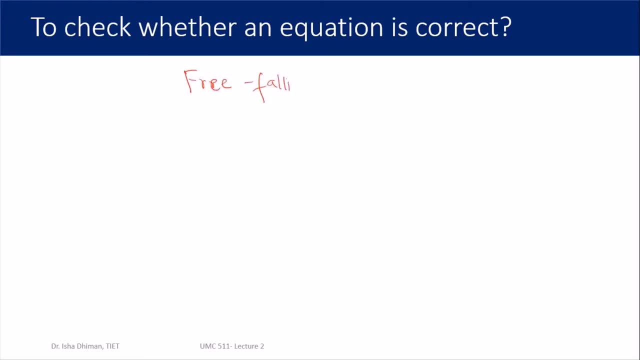 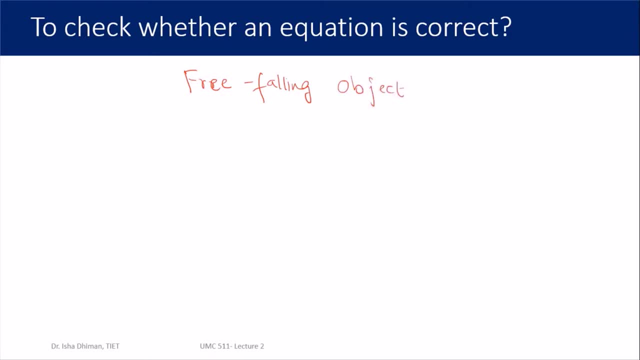 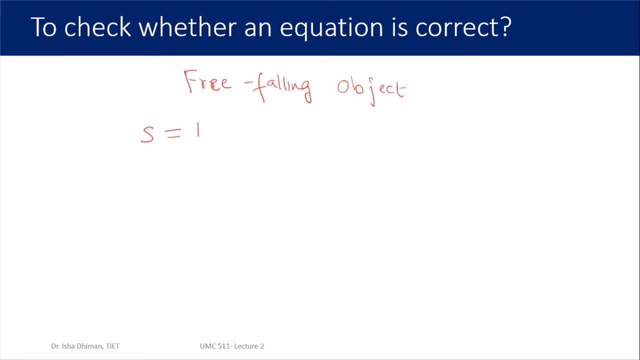 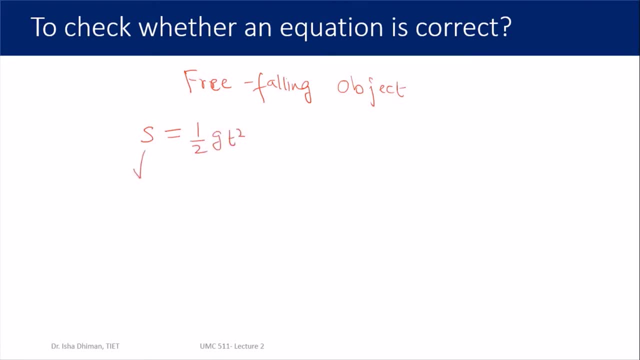 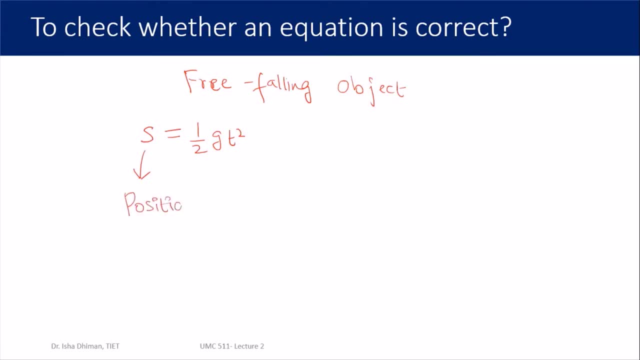 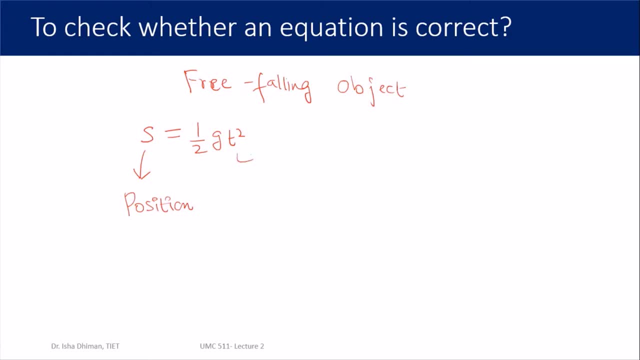 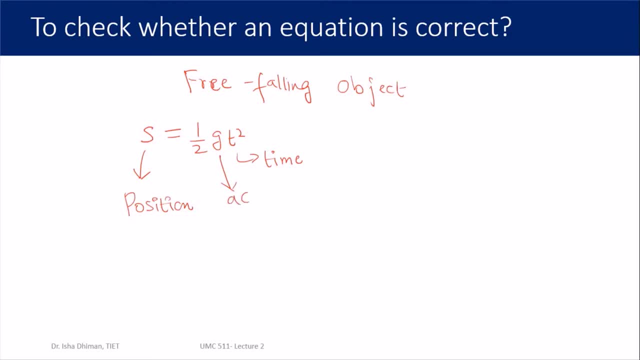 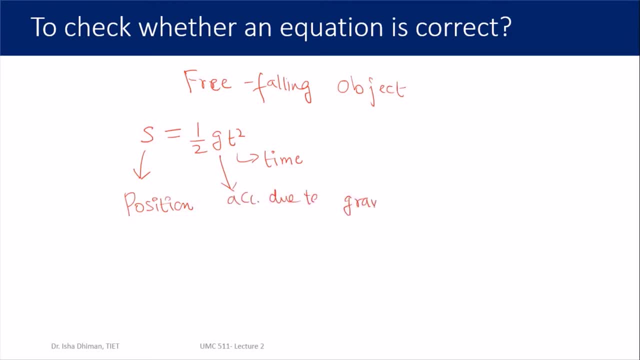 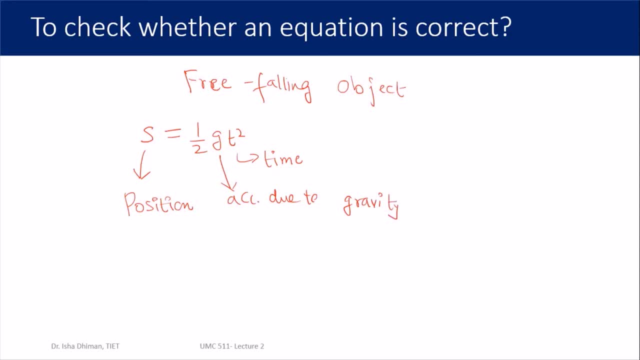 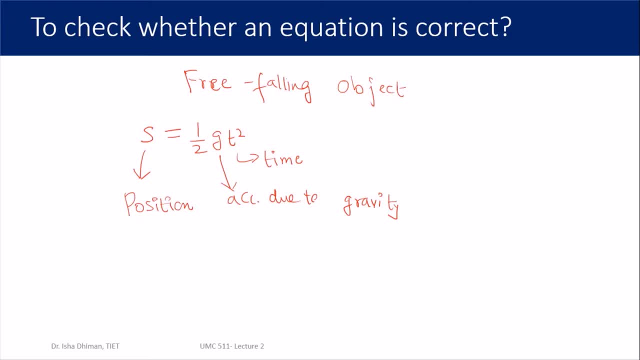 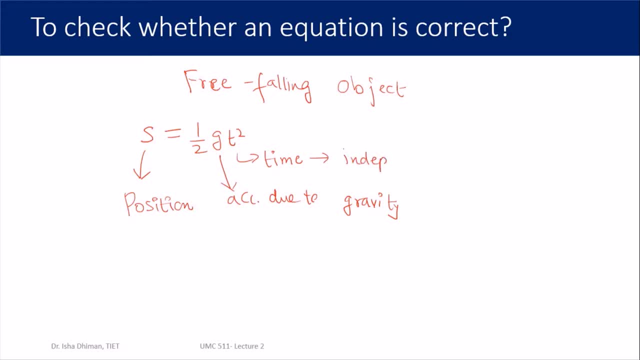 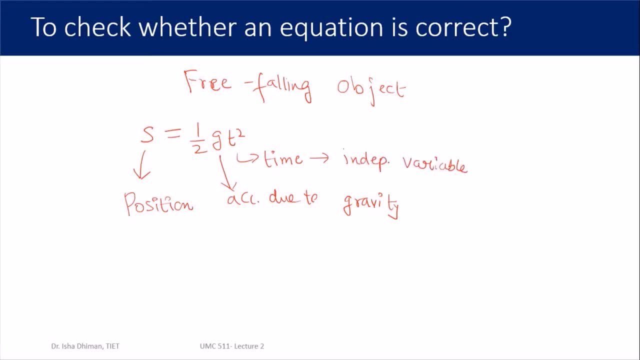 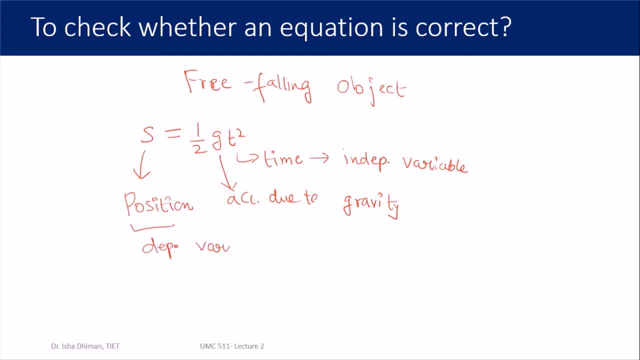 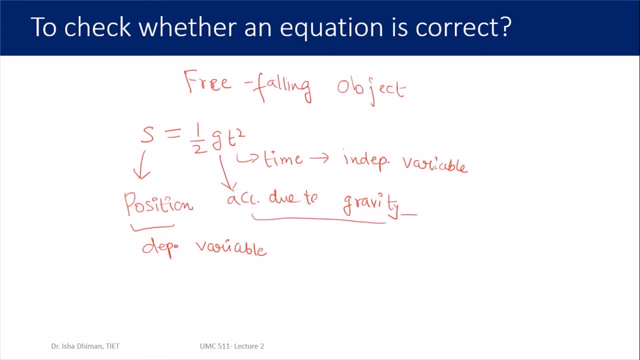 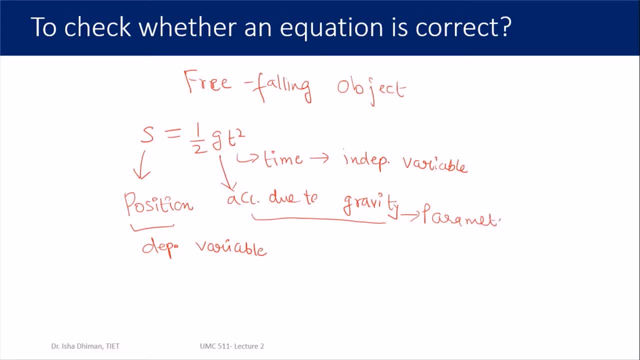 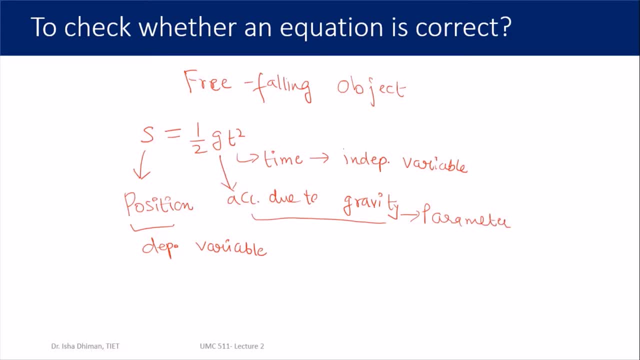 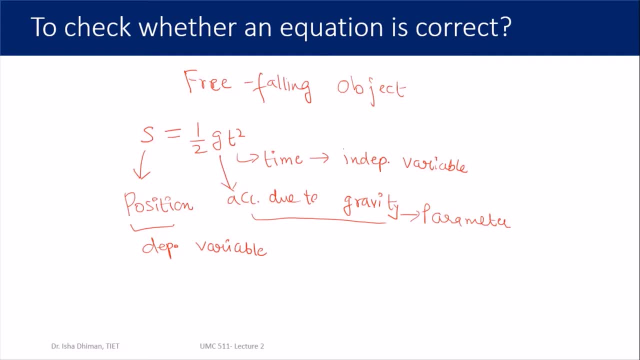 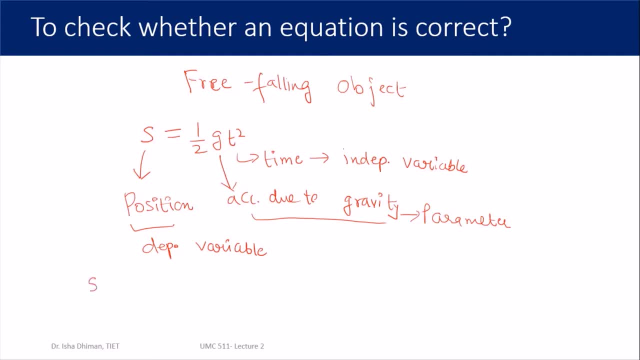 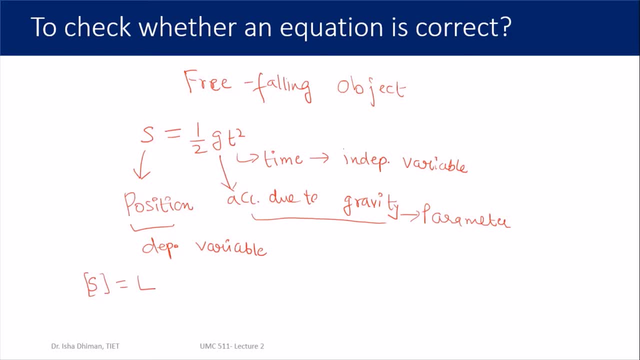 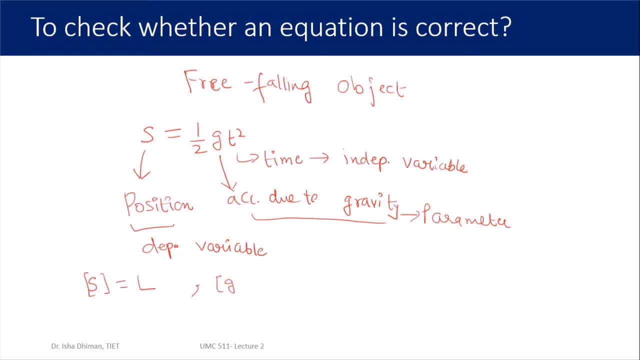 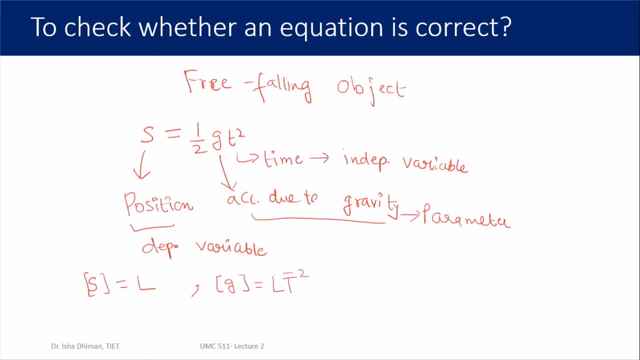 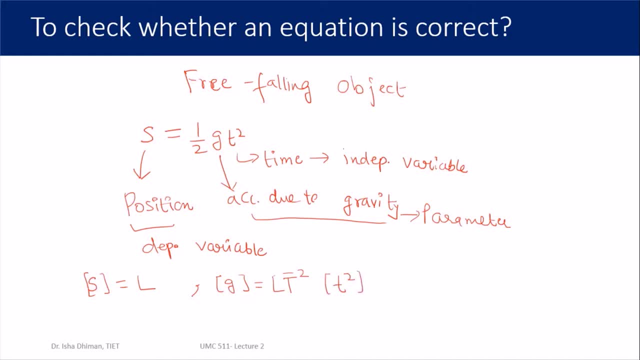 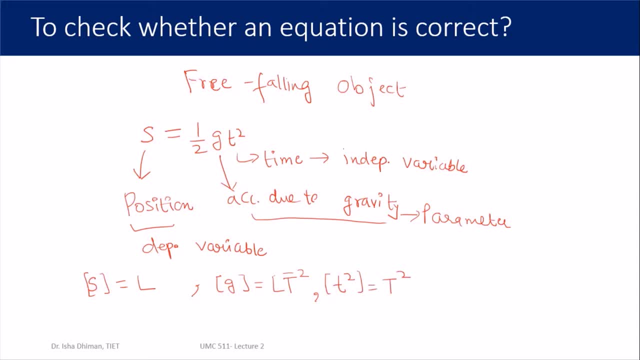 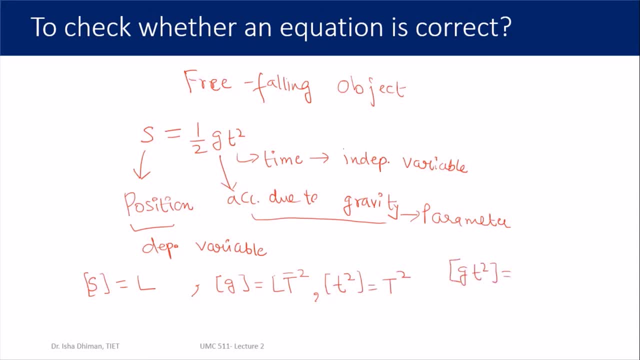 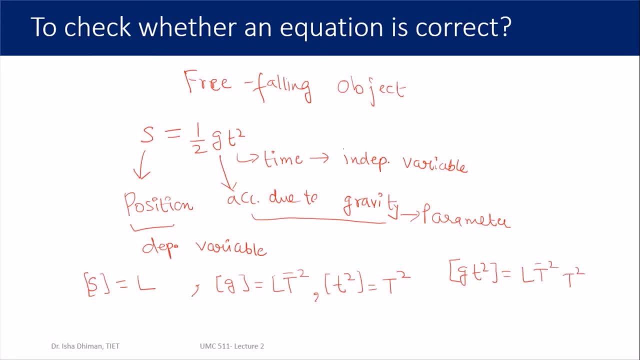 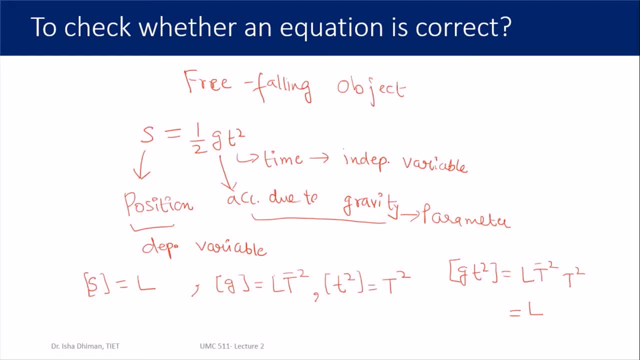 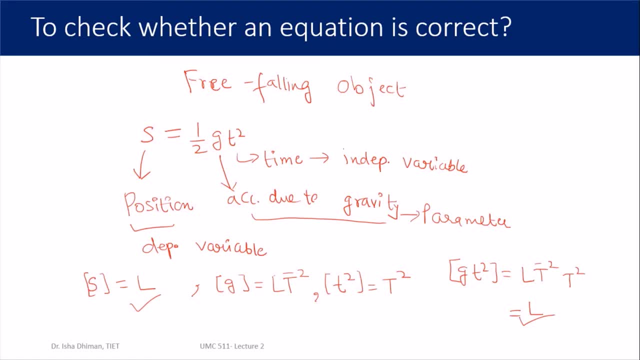 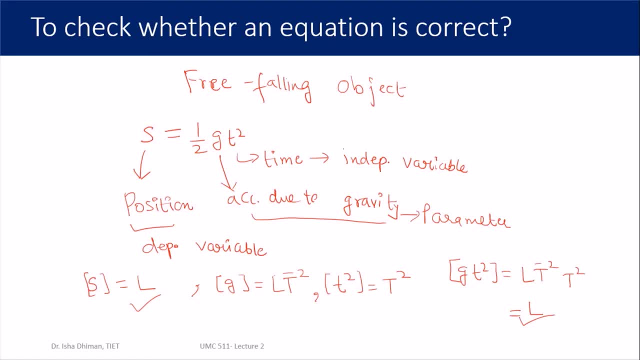 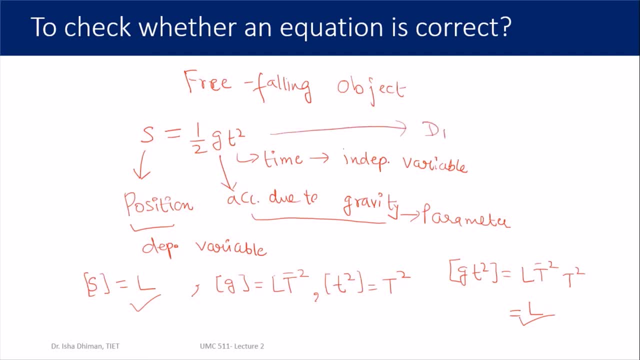 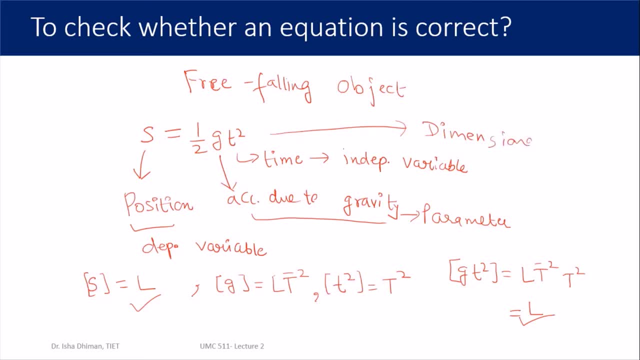 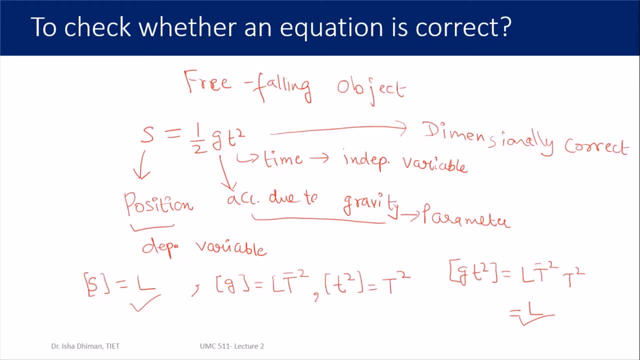 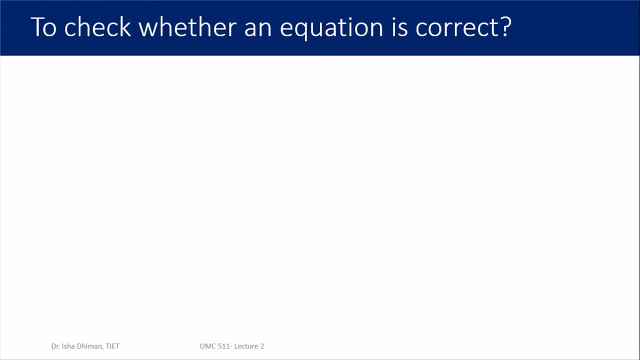 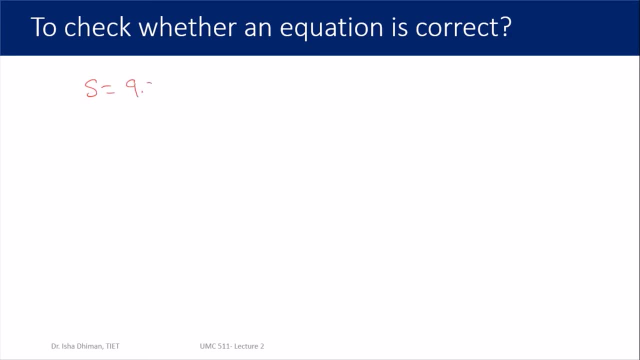 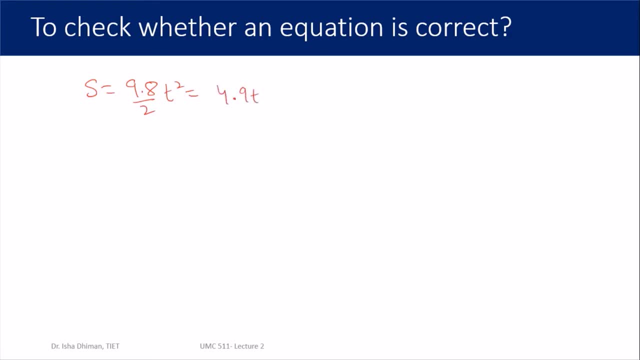 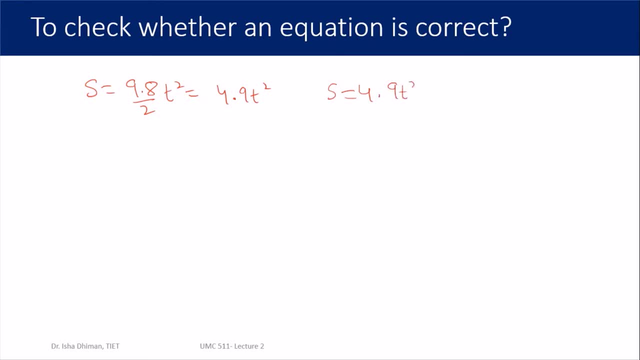 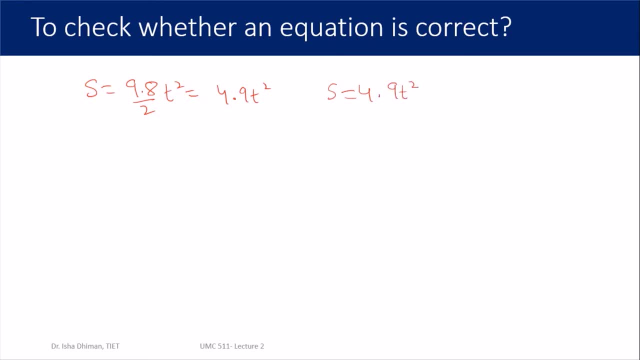 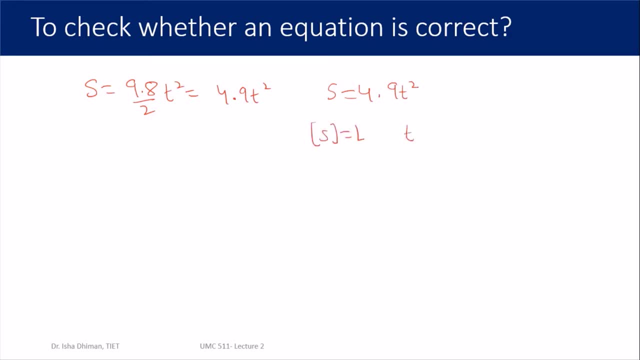 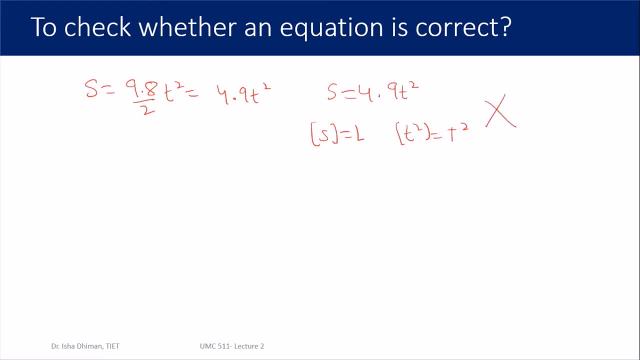 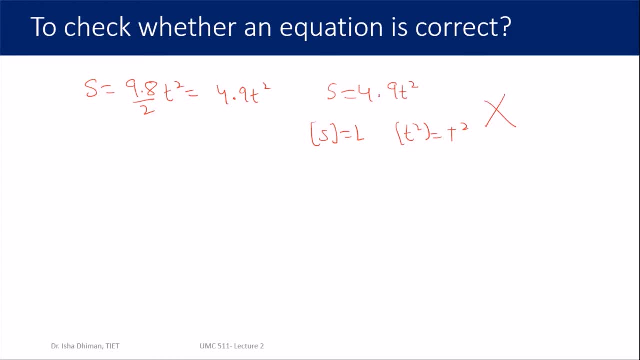 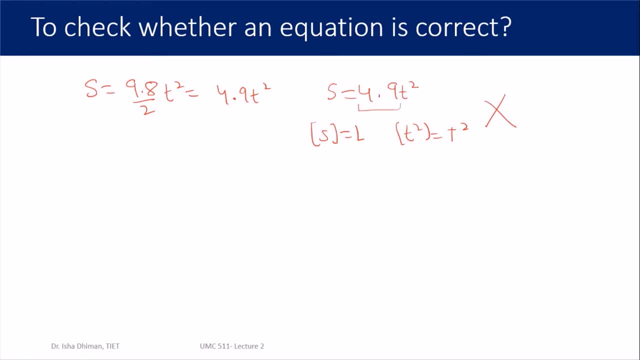 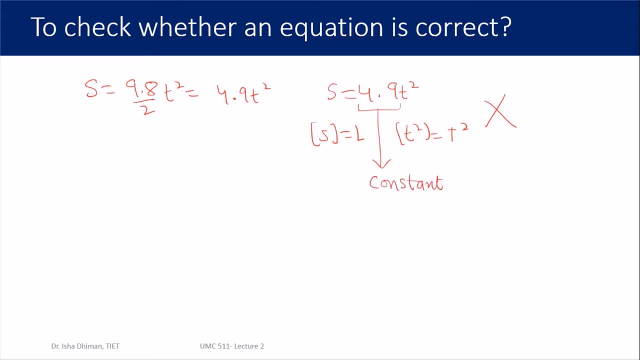 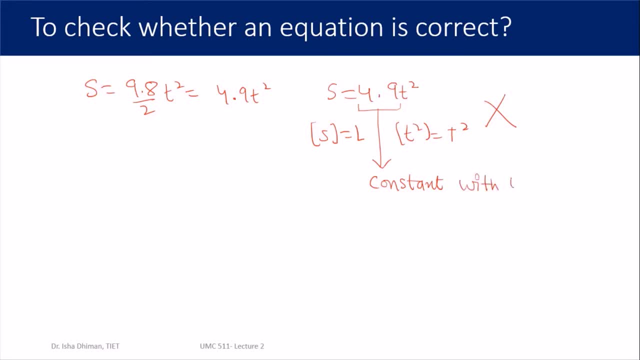 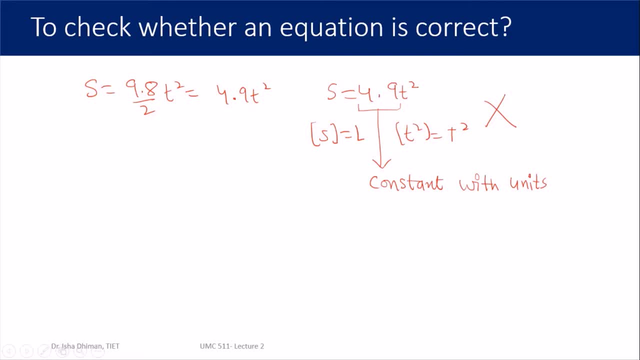 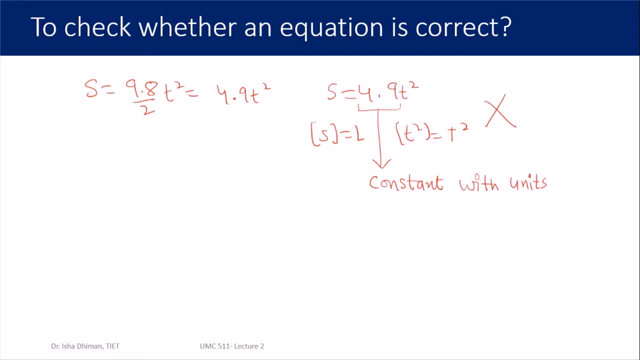 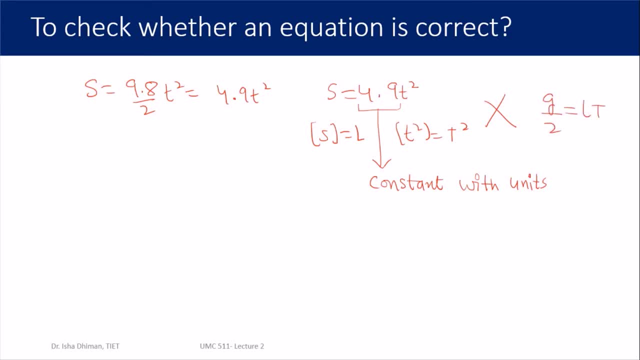 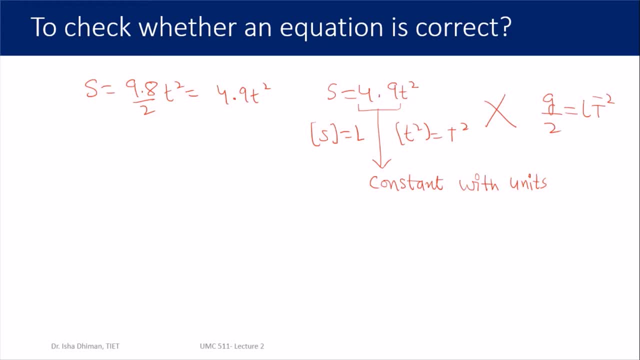 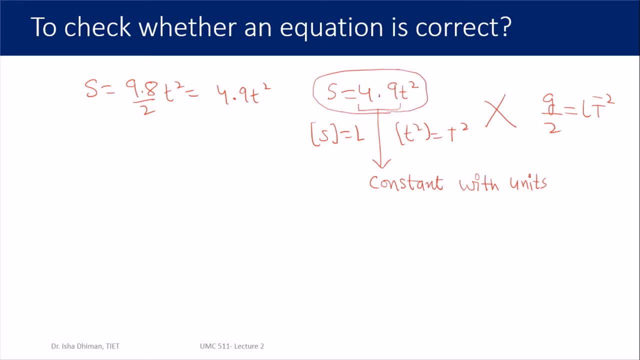 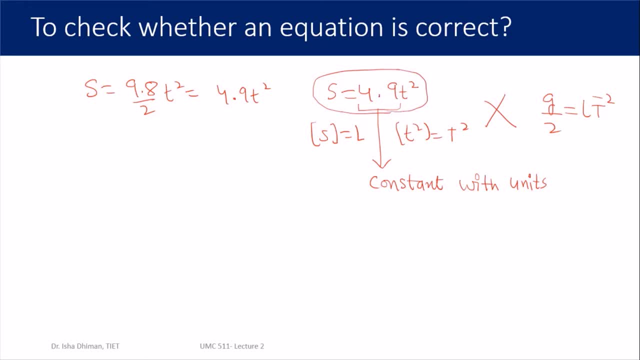 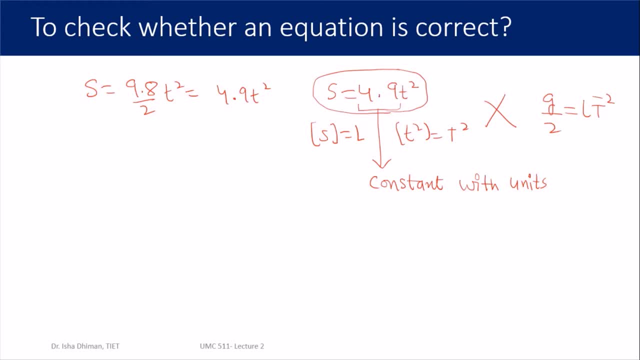 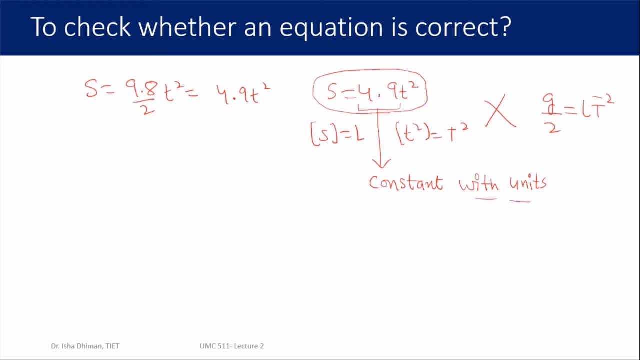 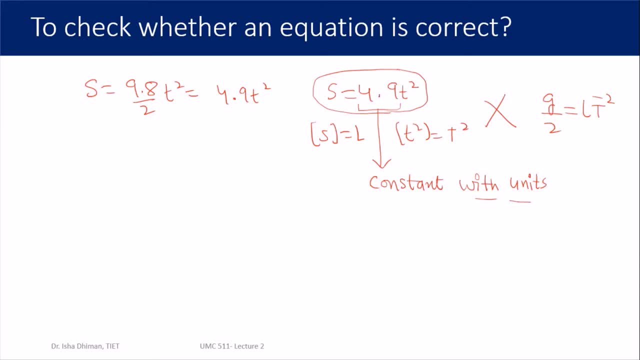 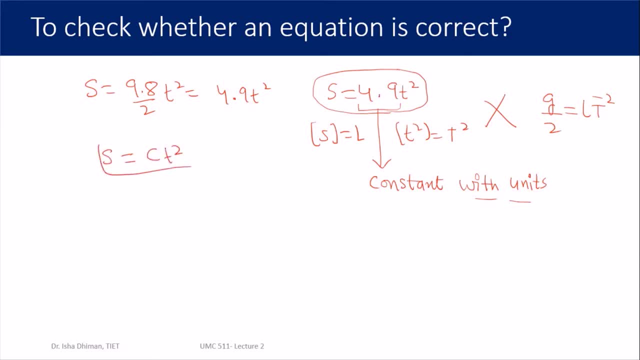 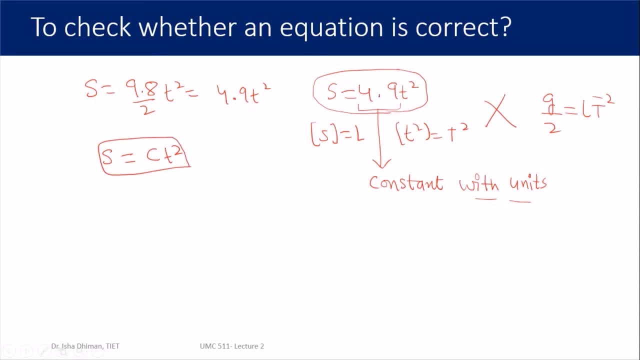 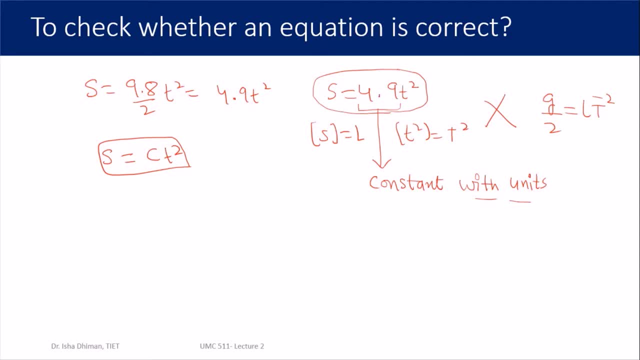 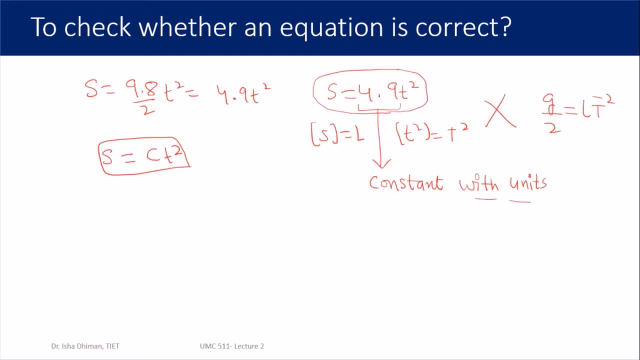 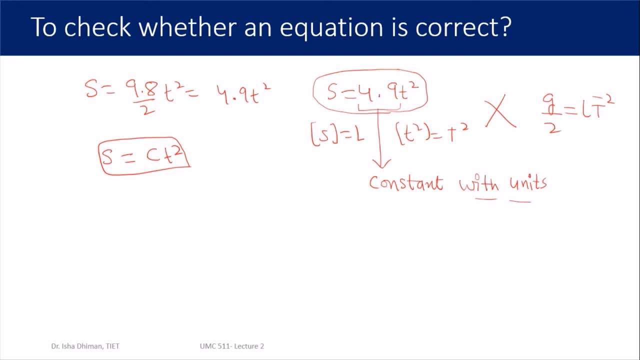 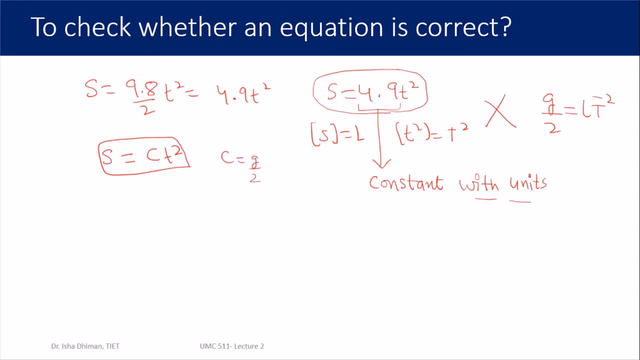 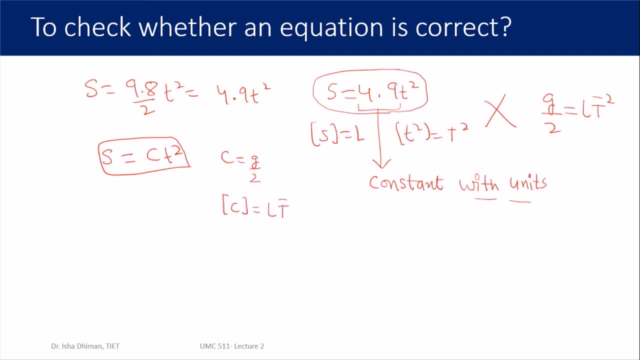 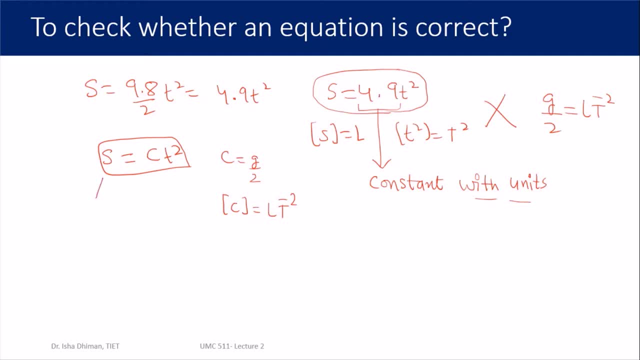 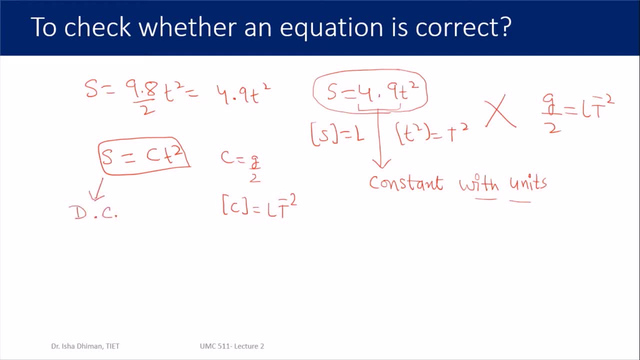 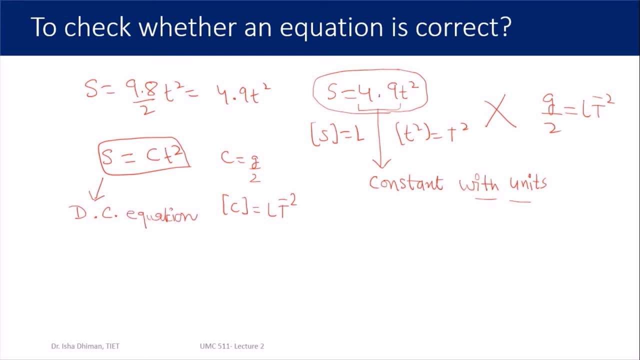 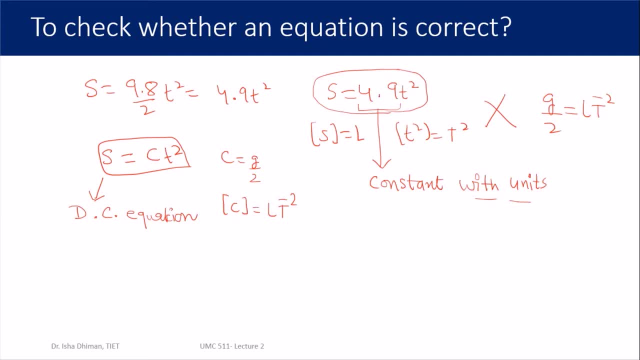 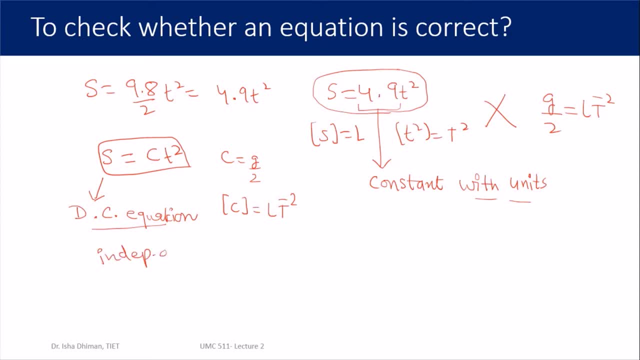 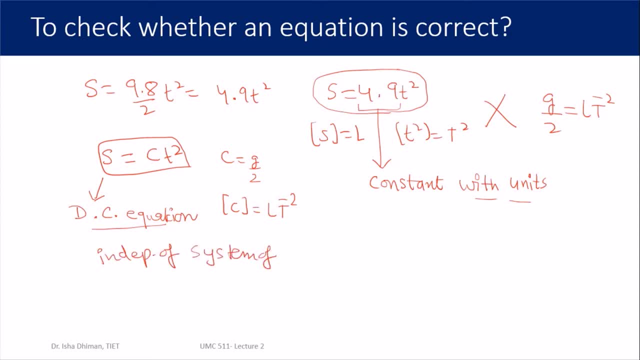 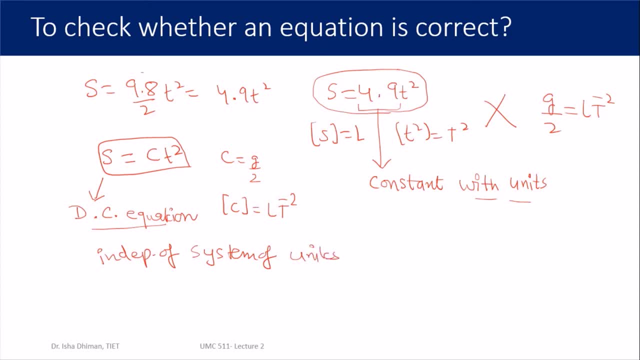 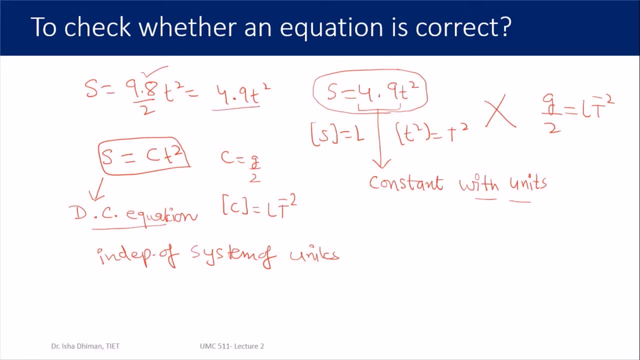 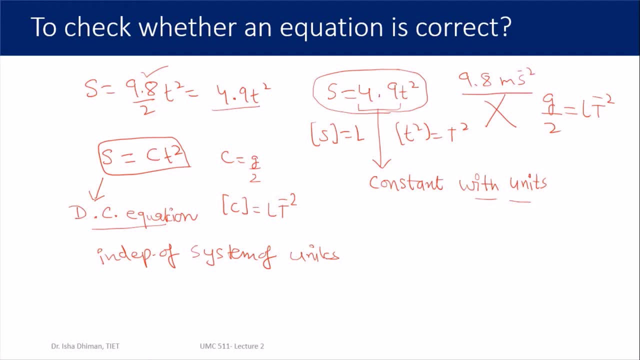 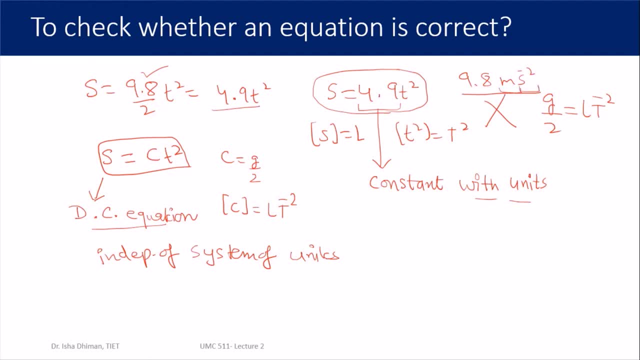 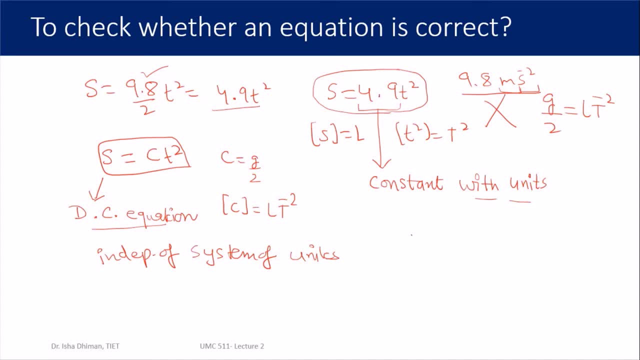 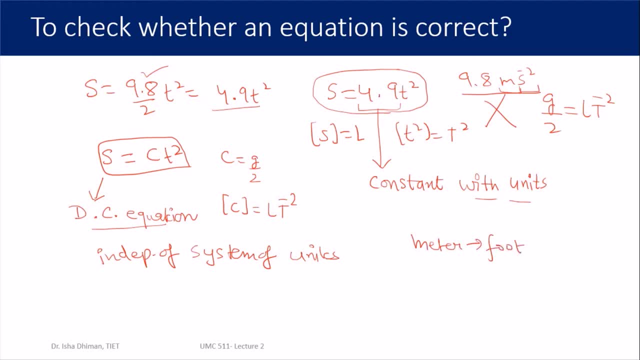 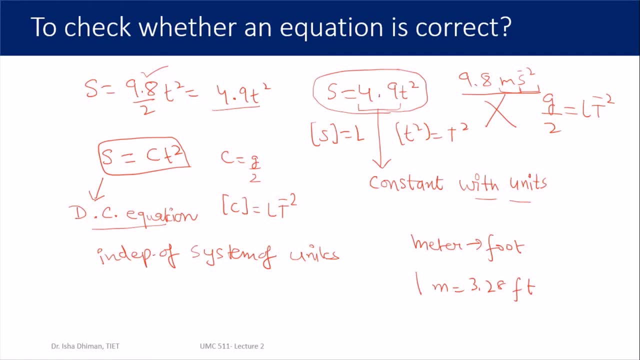 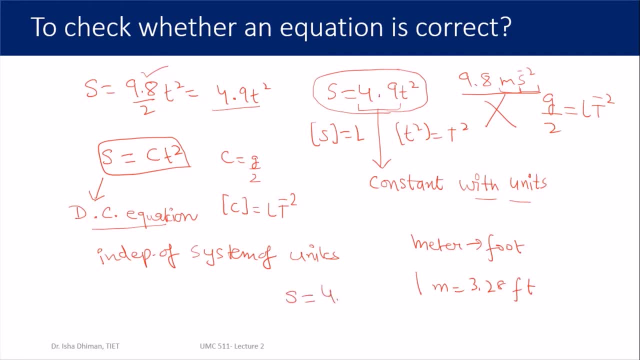 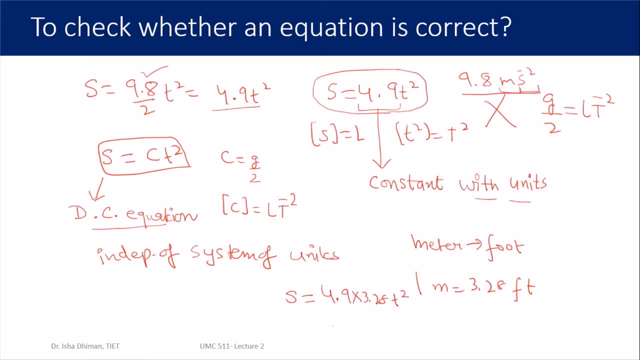 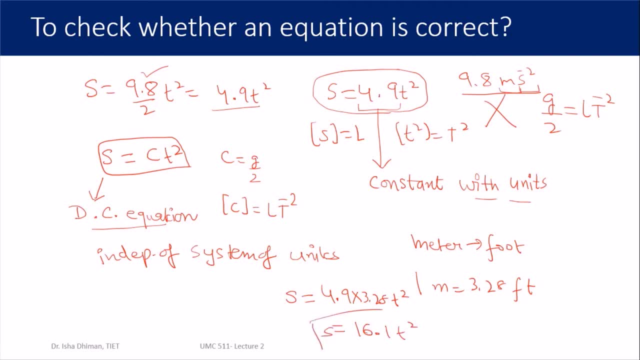 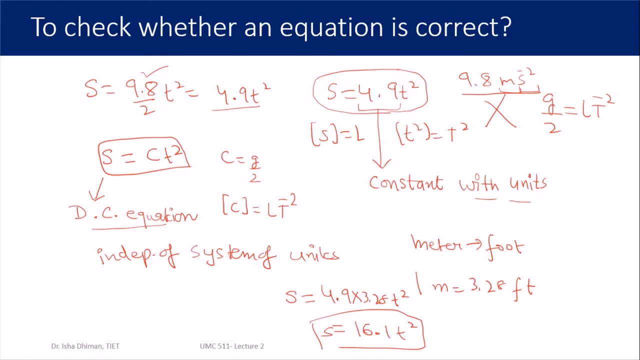 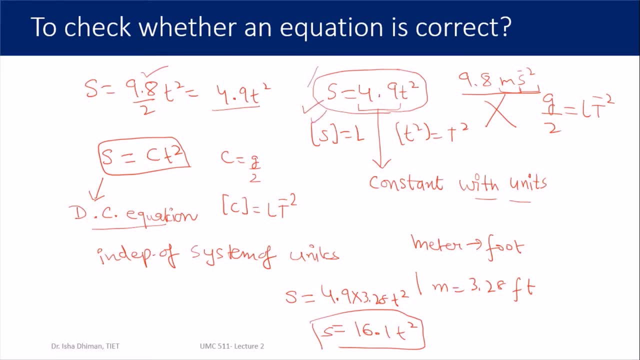 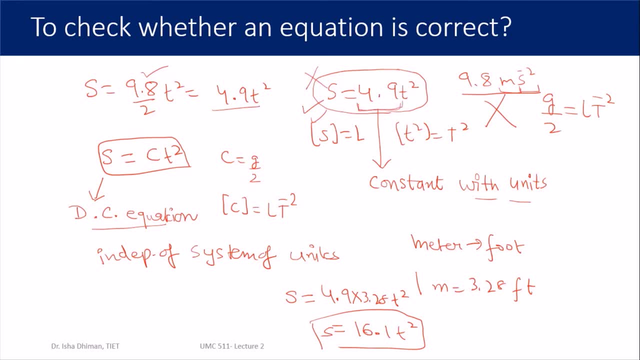 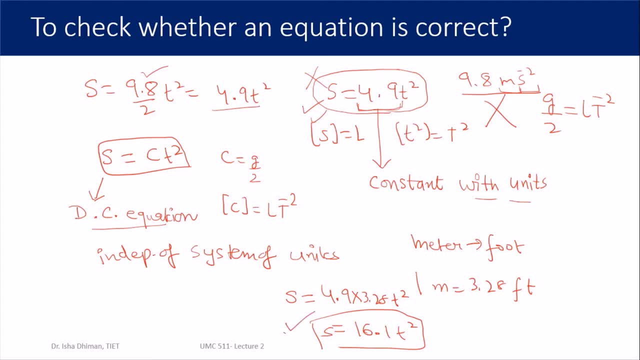 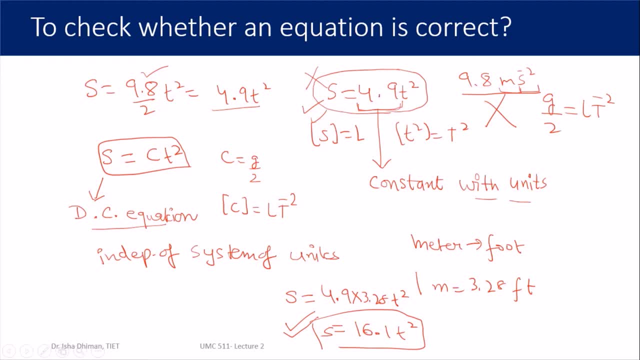 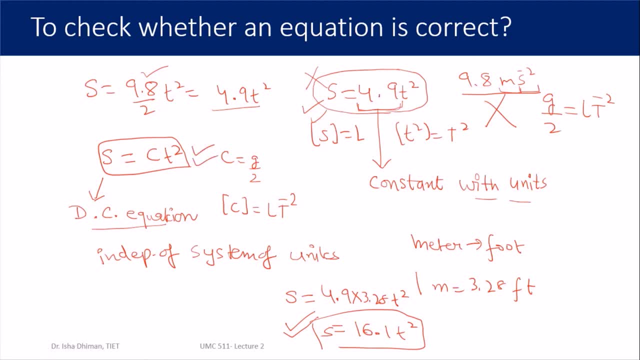 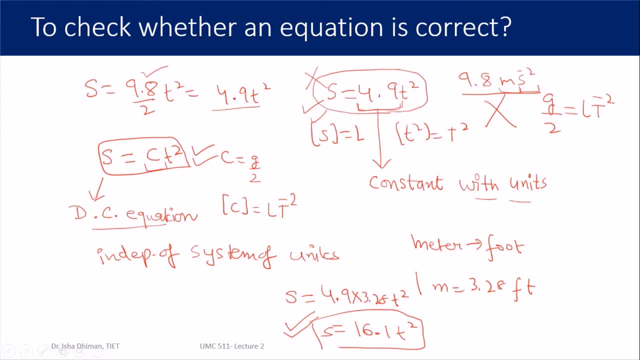 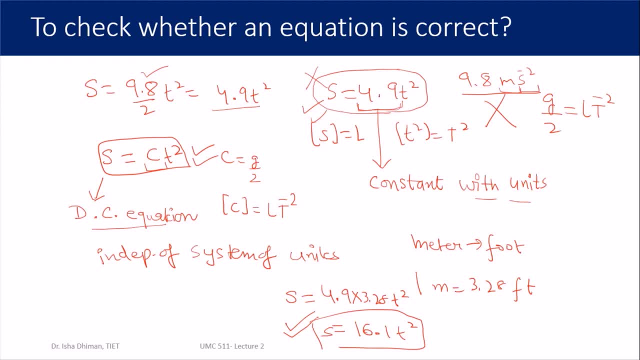 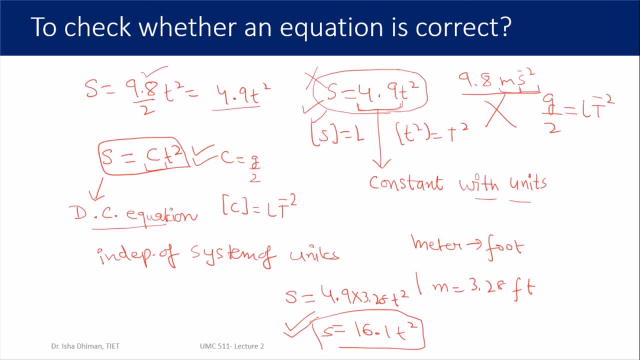 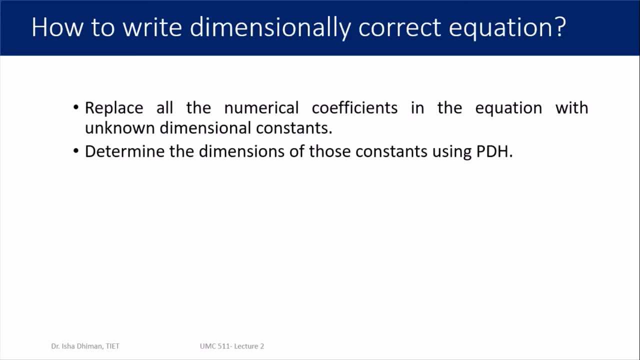 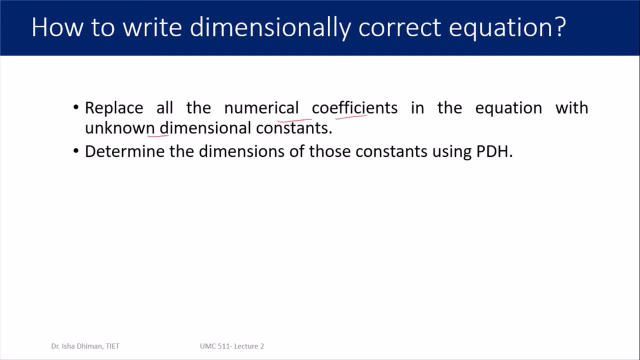 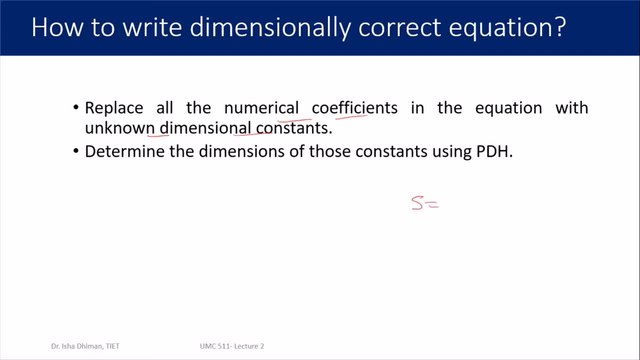 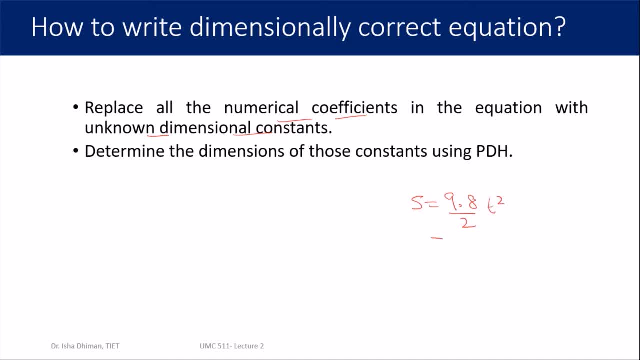 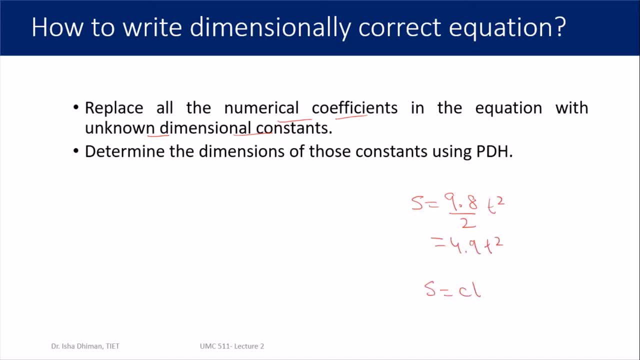 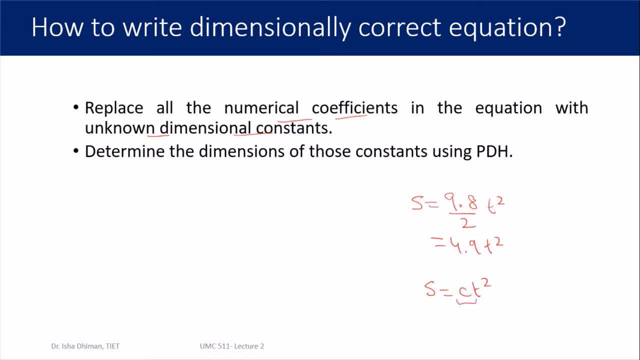 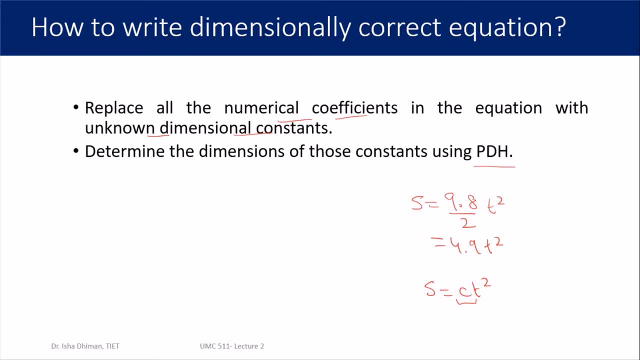 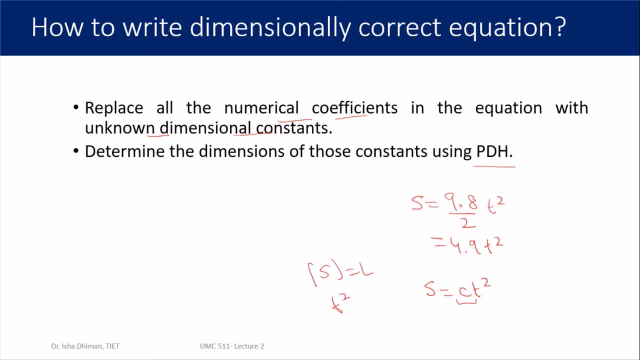 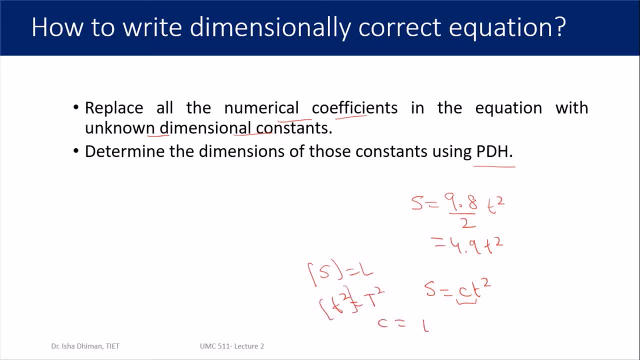 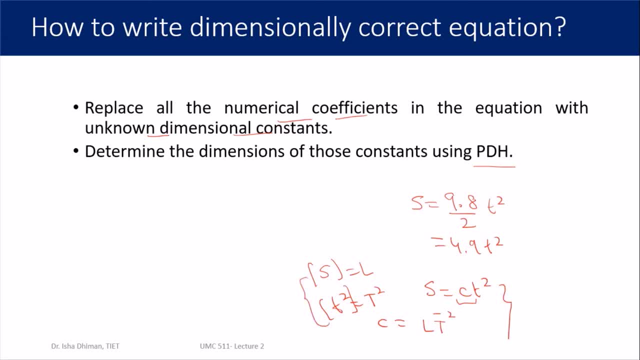 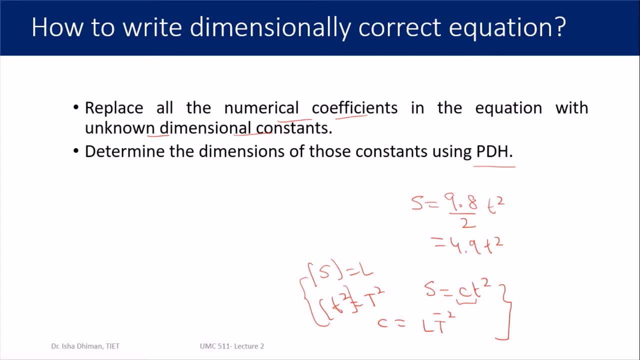 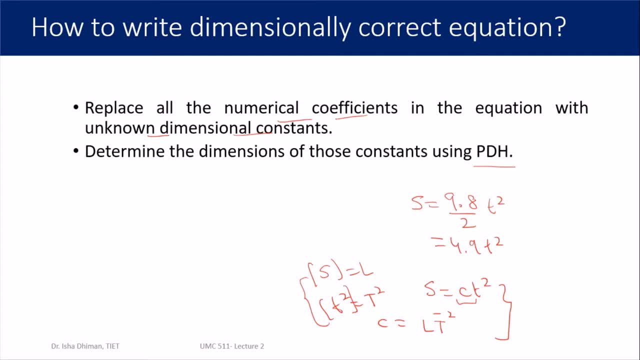 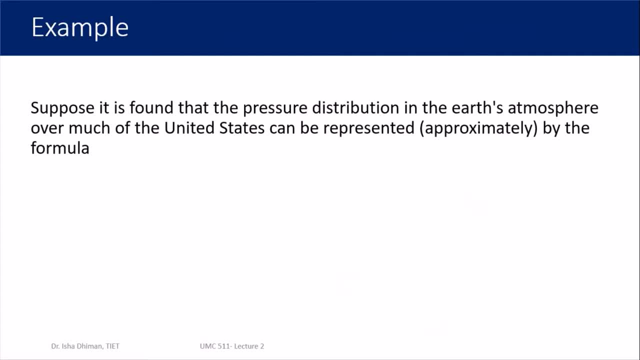 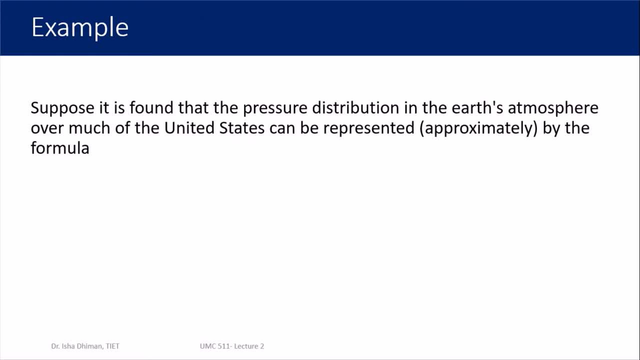 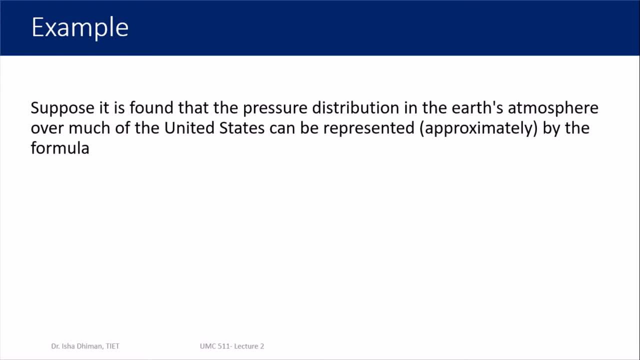 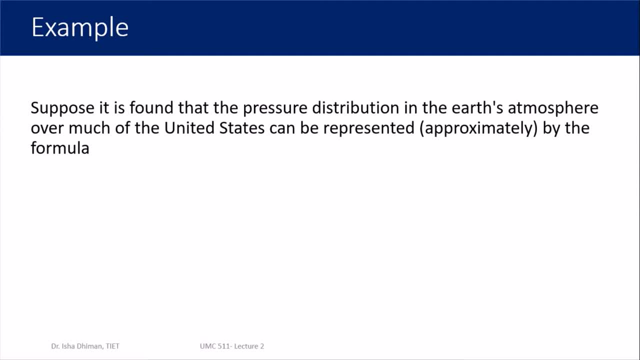 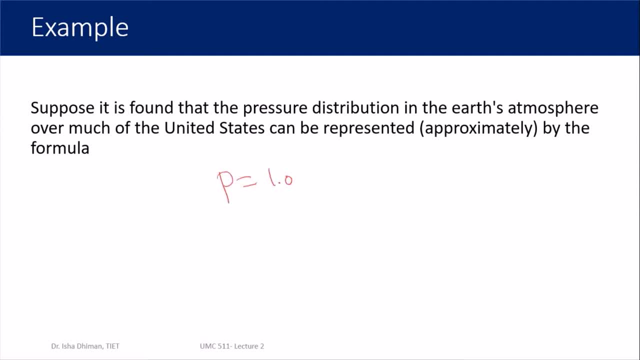 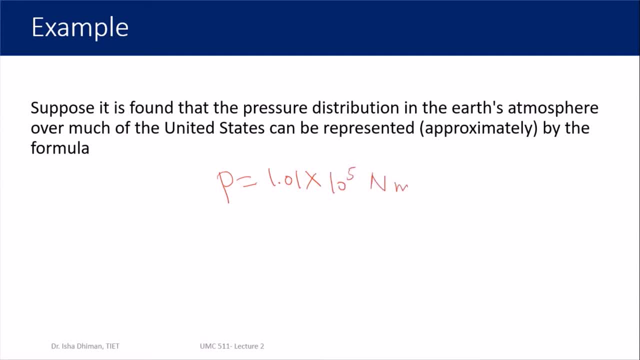 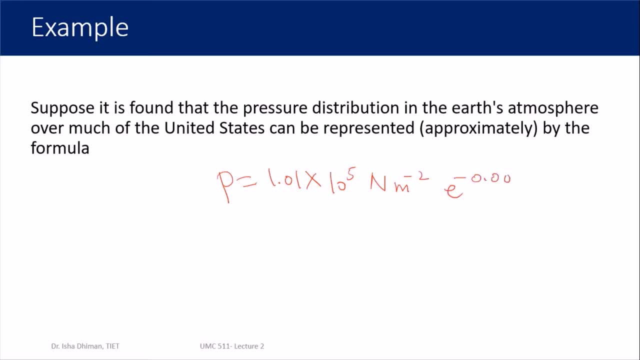 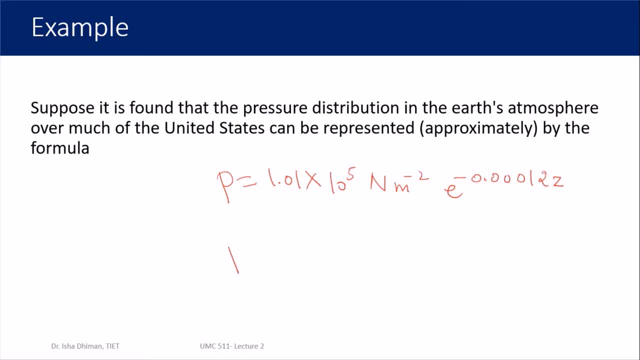 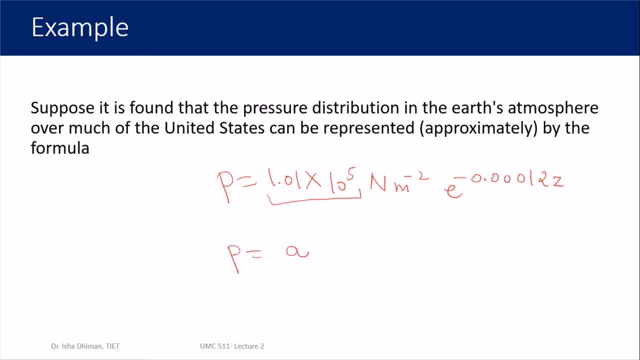 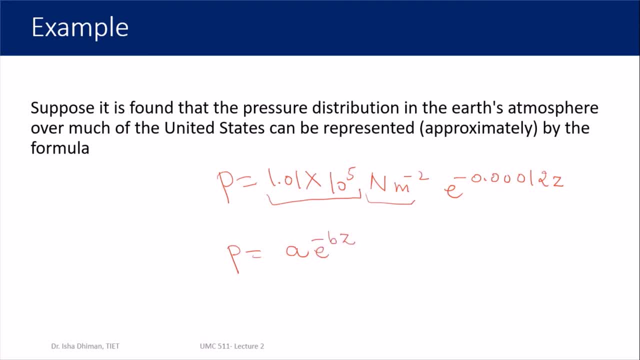 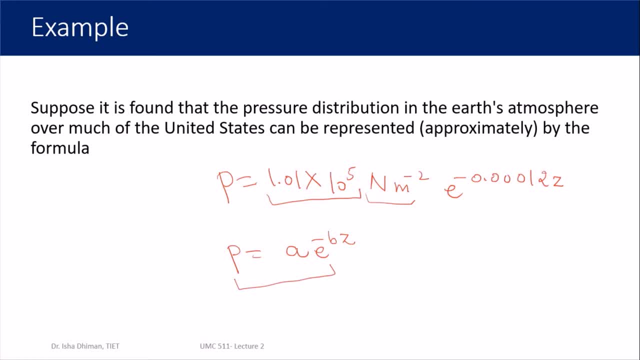 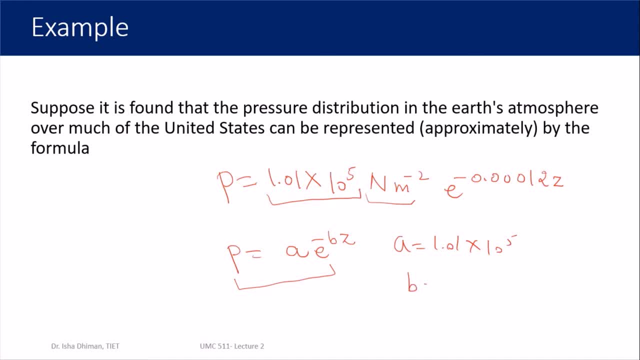 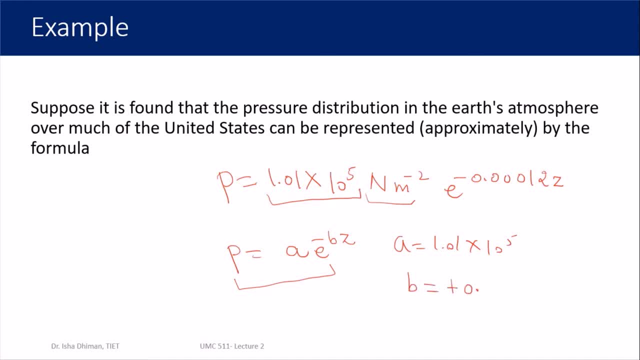 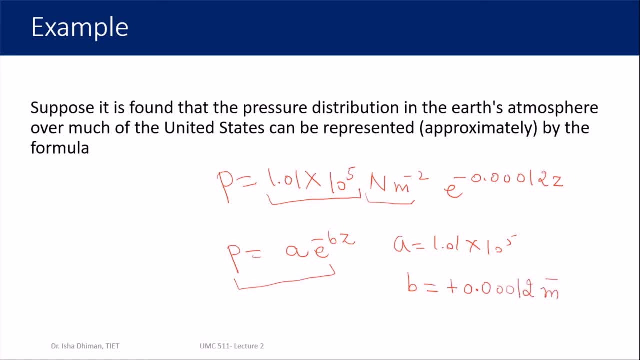 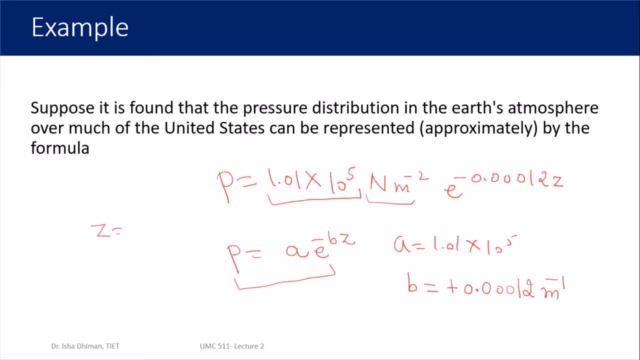 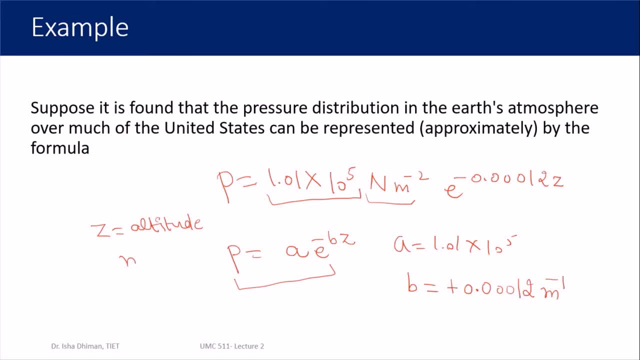 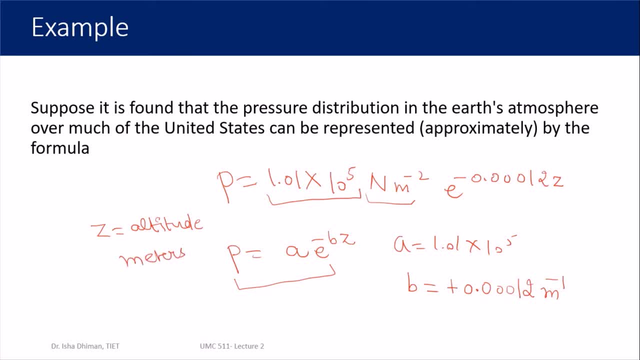 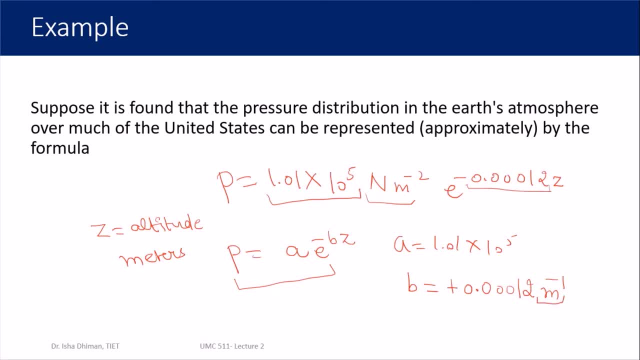 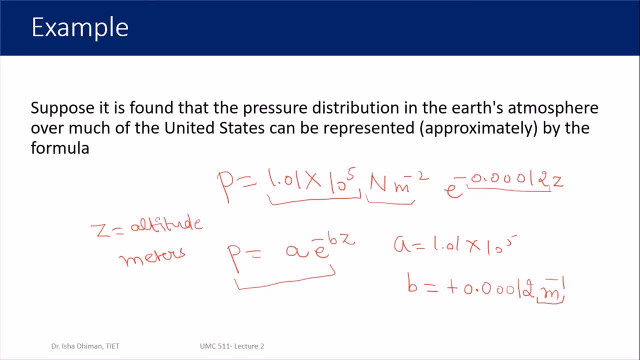 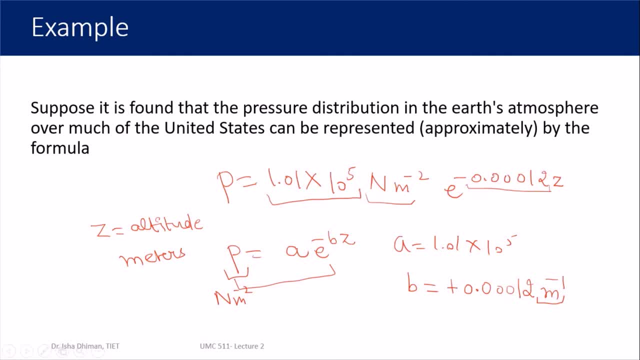 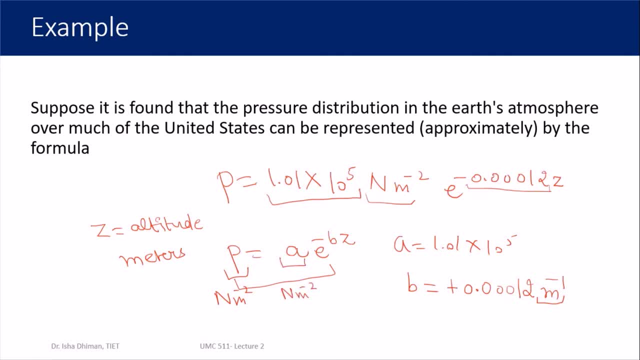 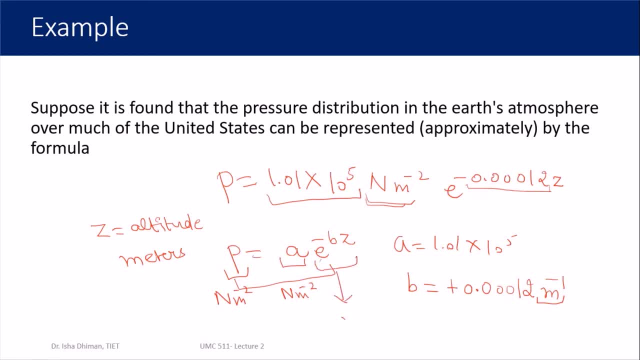 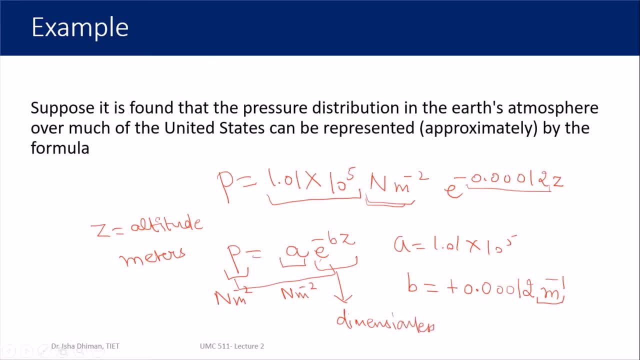 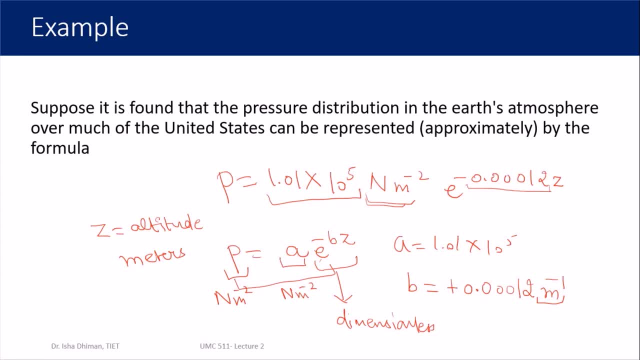 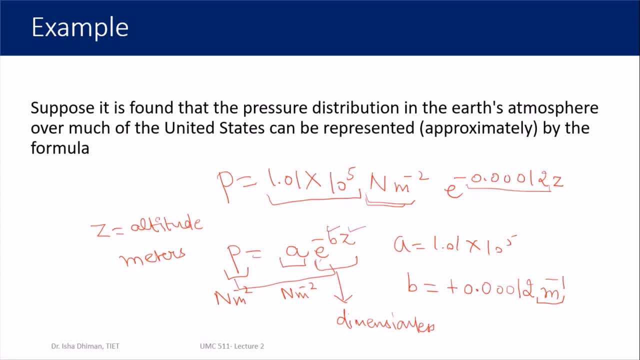 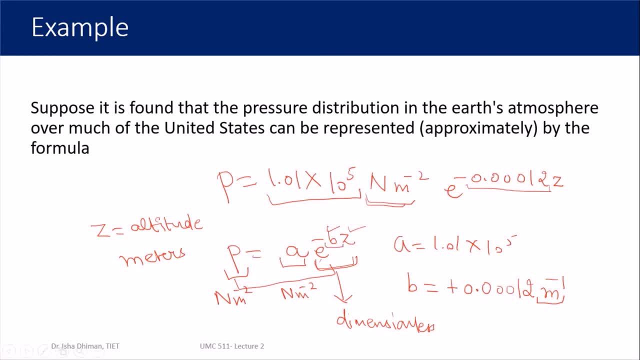 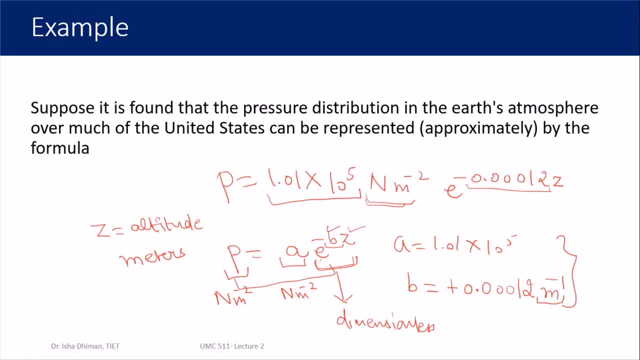 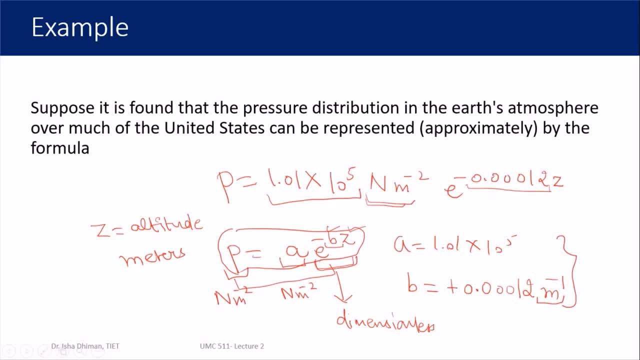